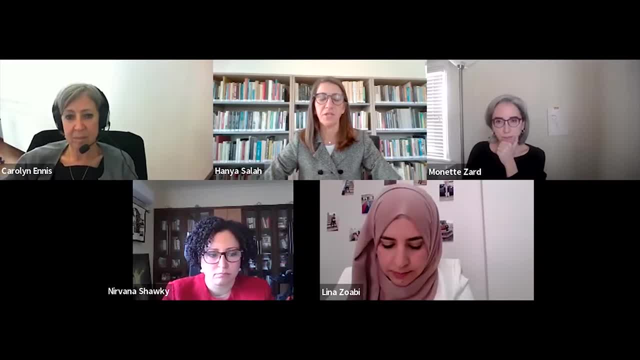 of Columbia Global Centers for Women's History Month on some of the issues confronting women around the world. Today's webinar, organized in partnership with CARE, will offer perspectives and shed light on employment issues facing Syrian refugee women in the MENA region. As many of you know, CARE is an international humanitarian organization delivering emergency. 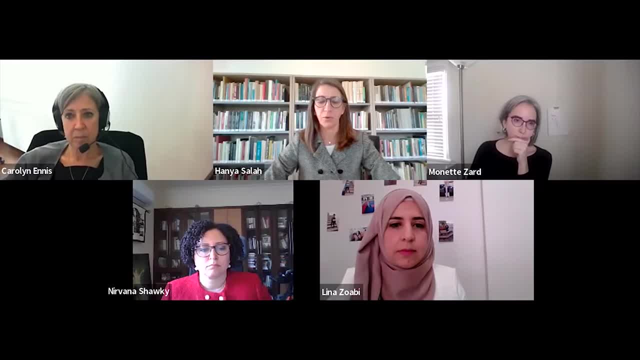 relief and long-term development projects. CARE works with refugees and host communities, with a particular focus on women's health and well-being. It has now been 11 years since the start of the Syrian crisis and many of those displaced neighboring countries are still in need of humanitarian assistance. The impact of the 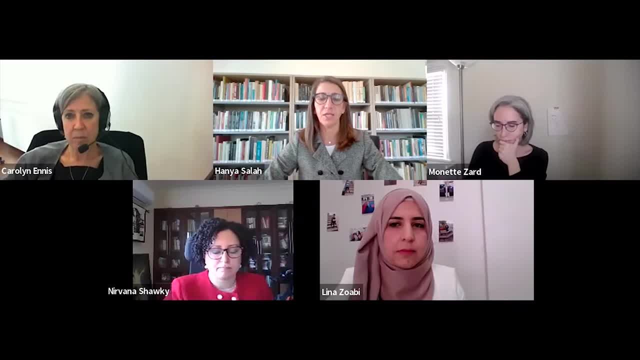 pandemic and increasing poverty has made the situation even more challenging, especially for Syrian refugee women and female heads of households, whose participation in the labor market is low. Although host governments are applying efforts to expand refugees' access to the labor market, they are not able to do so without the support of their families. 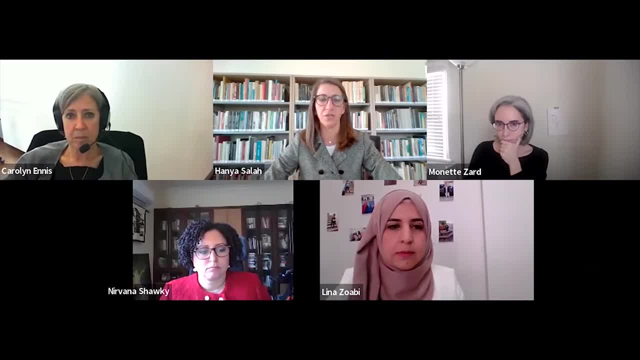 In addition, humanitarian agencies are offering a range of initiatives to enhance access to livelihood opportunities for Syrian refugee women. These challenges include policies that often limit the sectors in which refugees are allowed to work in linking training to work opportunities, as well as challenges concerning mobility and transportation, and cultural 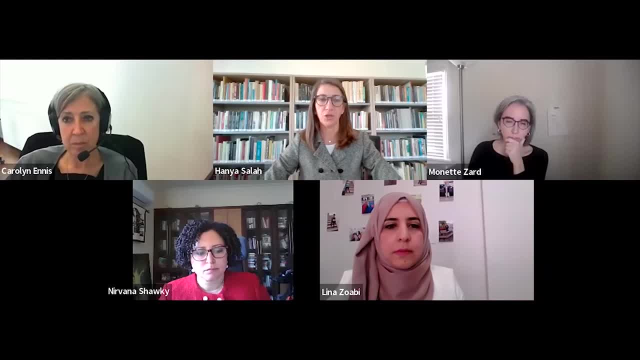 expectations in relation to gender norms. Ensuring that refugees have access to livelihoods is a crucial stepping stone to support resilience and self-reliance. Through today's discussion, we aim to gain a deeper understanding of the livelihood situation of Syrian refugee women and how to include them more actively in processes affecting 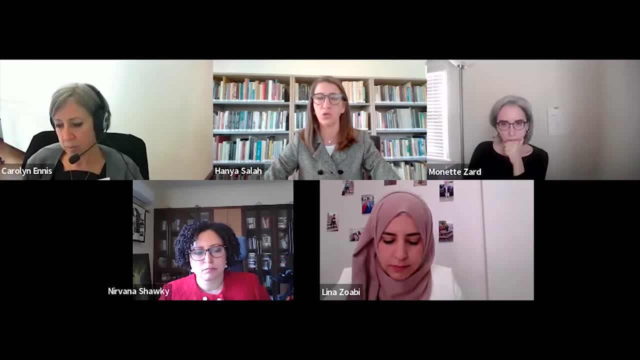 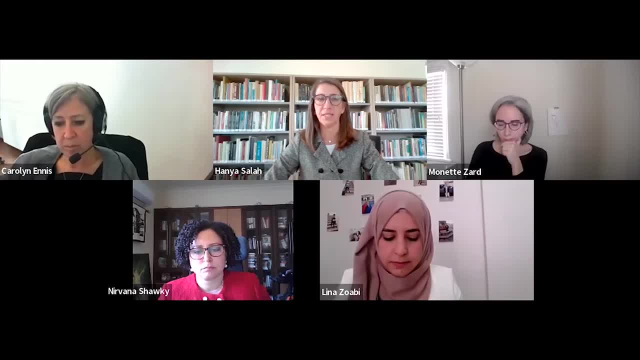 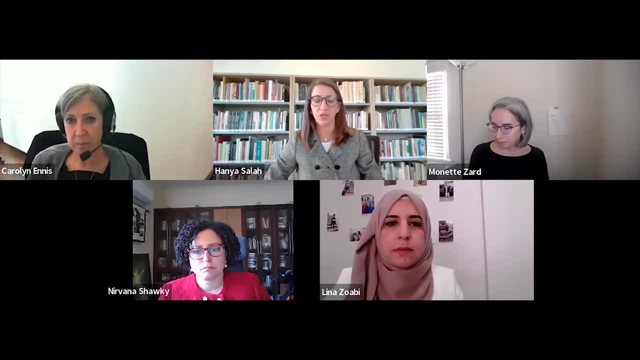 humanitarian sector and academia to offer their experiences and perspectives. I would now like to hand over to Professor Monet Zard, who will introduce our speaker and speakers and serve as our moderator for this conversation. Professor Zard is the Alan Rosenfield Associate Professor of Forced Migration and Health. 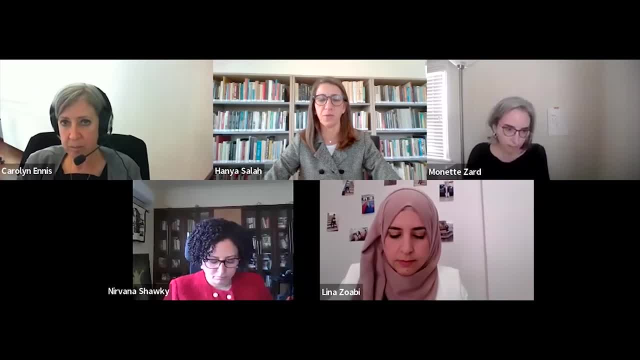 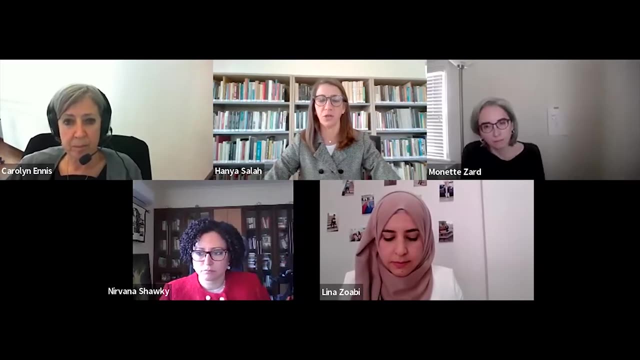 at Columbia University and Director of the Program on Forced Migration and Health, and a member of the Faculty Advisory Committee for the Amman Global Center. Monette has also served as the Global Human Rights Program Officer at the Ford Foundation in New York and as a Research Director at the International Council on Human Rights Policy in Geneva. 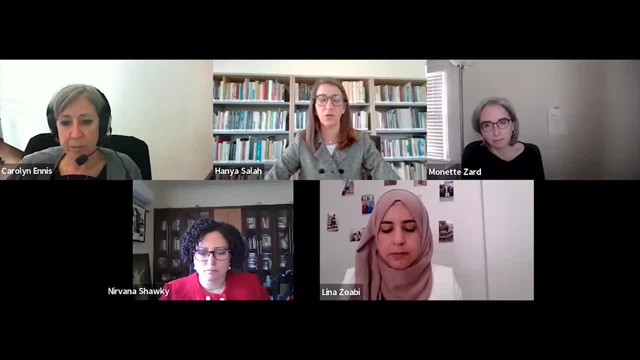 She has consulted on international human rights and forced migration issues for several organizations, including Amnesty International, the Brookings Institute, Human Rights Watch and the United Nations High Commissioner for Refugees. Thank you again to everyone in our virtual audience for being with us. 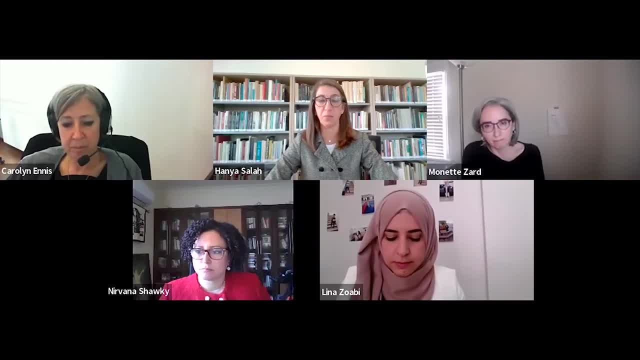 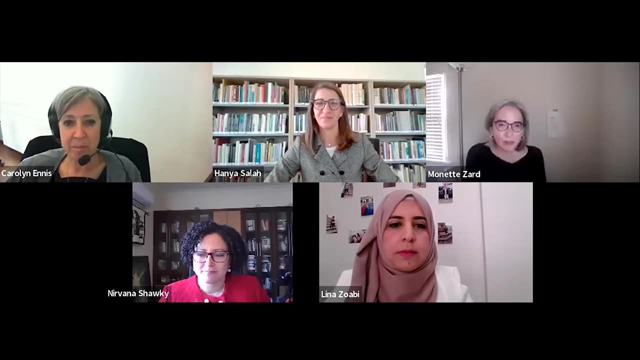 We encourage you to send in your questions through the Q&A chat box at the bottom of your screen. We will address them in the latter half of this webinar. Please join me in welcoming Professor Monette Zard, Thank you. Thank you so much, Hania, for that kind introduction and good morning afternoon wherever it is in the audience. 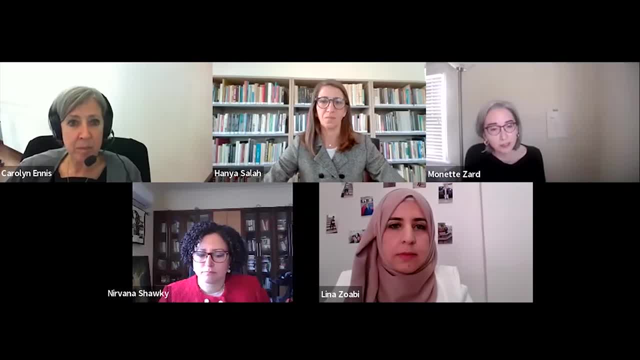 So welcome to today's panel. As Hania indicated in this, the 11th year of the Syria crisis. our conversation today will focus on how Syrian refugee women in the MENA region are navigating work and the livelihood space, what lessons we've learned over the course of this crisis, and what challenges remain and how to meet them. 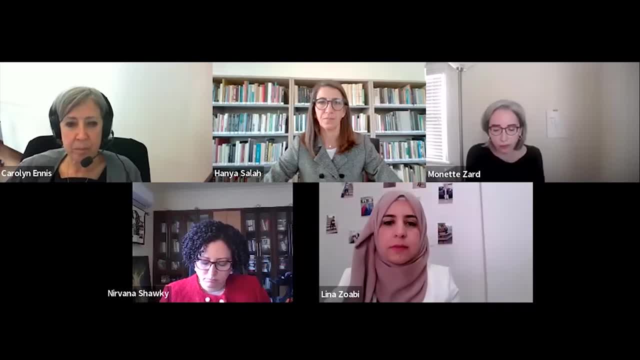 Now we know that access to livelihood is an important pathway to promoting the right to work is fundamental to the dignity, survival and security of refugees. But it's also important for us to recognize that the UN has worked very hard to increase valor and sustainability for refugees. 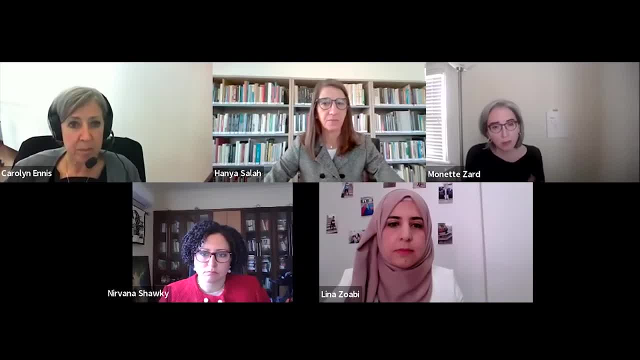 and it is a right that is protected under international human rights law- Promoting a profoundly pragmatic position for both national governments and international donors, given the potential economic contribution of the refugee workforce to local economies and the fact that international humanitarian and development aid budgets are finite. 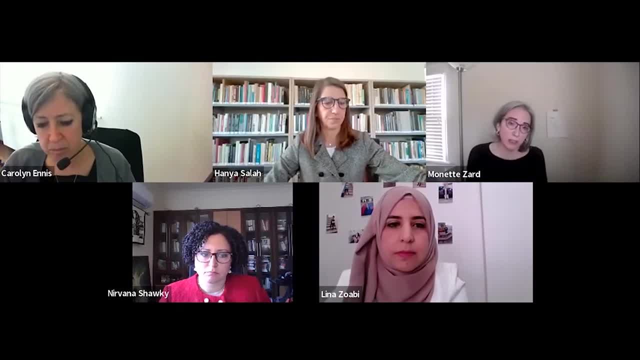 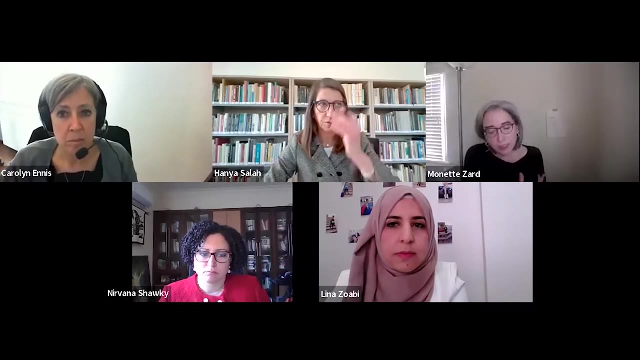 and that the attention span of the international community is unfortunately limited. But the refugee livelihoods discussion in the MENA region needs to be situated against a backdrop of high unemployment, particularly youth unemployment, in many of the hosting countries and a challenging economic outlook made worse by the COVID pandemic. 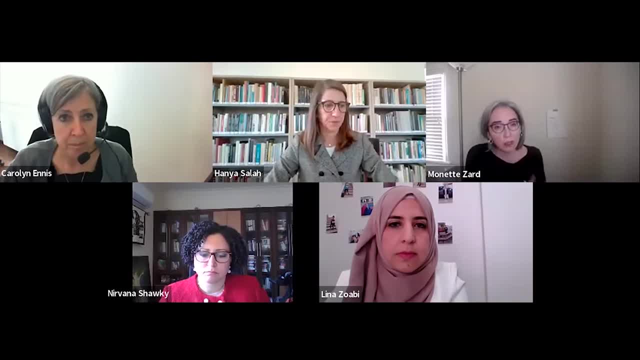 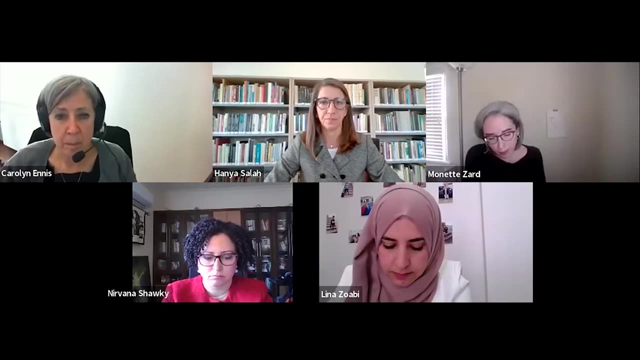 In women. we all need to bear in mind that even prior to the conflict, Syrian women had low workforce participation rates of 13% according to the ILO, and an unemployment rate of 22% intensified both the need and the willingness on the part of women to work and to earn an income. 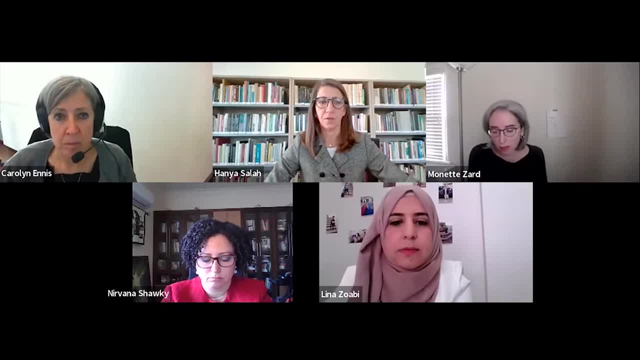 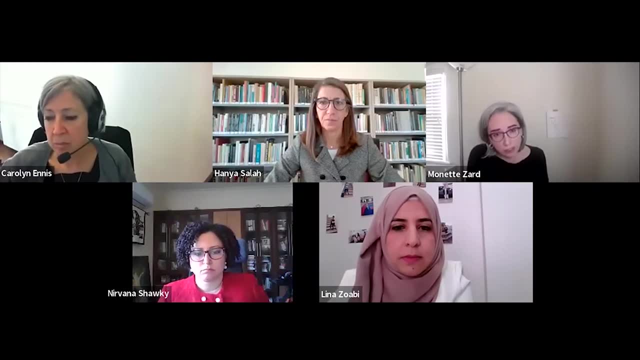 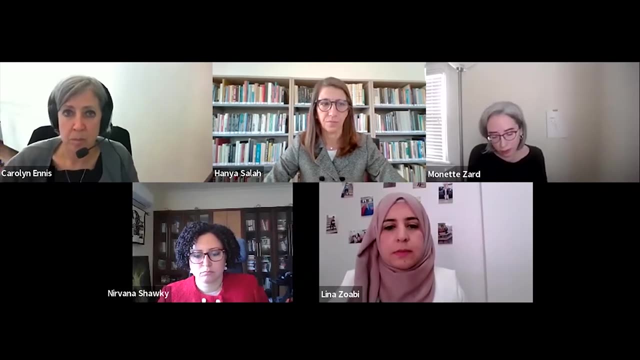 particularly given the prevalence of female-headed households among refugee communities. On a positive note, the MENA region has seen a lot of innovation and creativity in crafting solutions to fostering economic inclusion of refugees and generating livelihood opportunities. In both Turkey and Jordan we've seen moves towards including refugees. 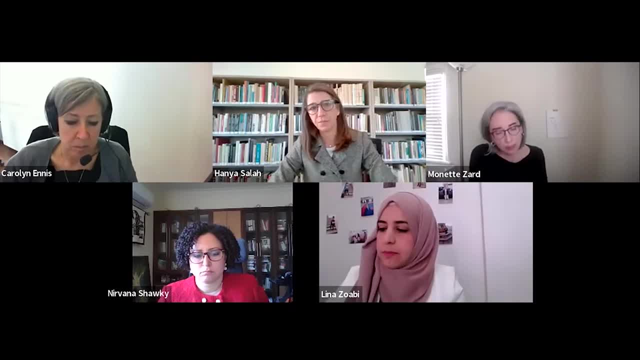 in the formal labor market through issuing refugees work permits. The 2016 Jordan Compact, for example, saw the government pledge to provide 200,000 refugees In the current year. more than 2.5 million refugees are currently on the road. 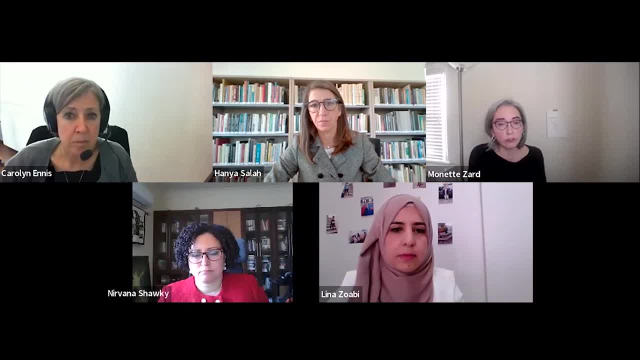 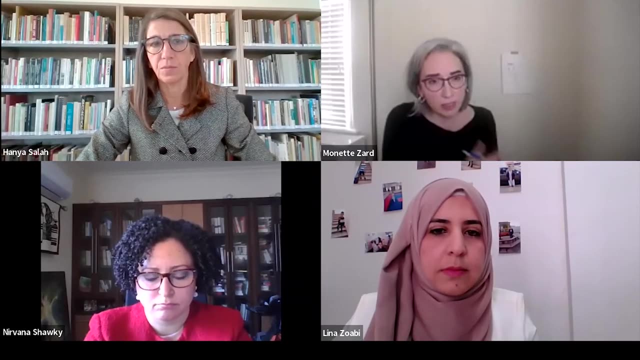 to work with children or adults making the most of the opening hours, of work permits for Syrian refugees In other humanitarian responses variants being issued- an estimated 62,000 last year, although that was a record number And there are numerous reasons for this. 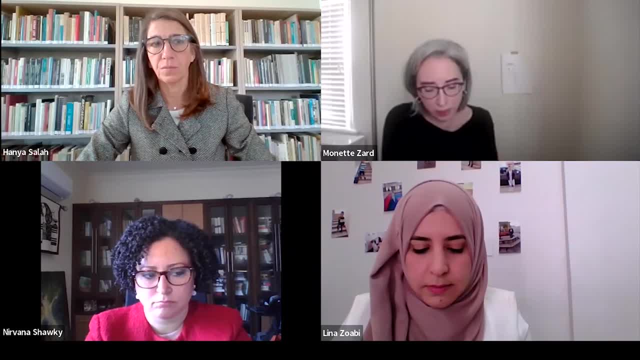 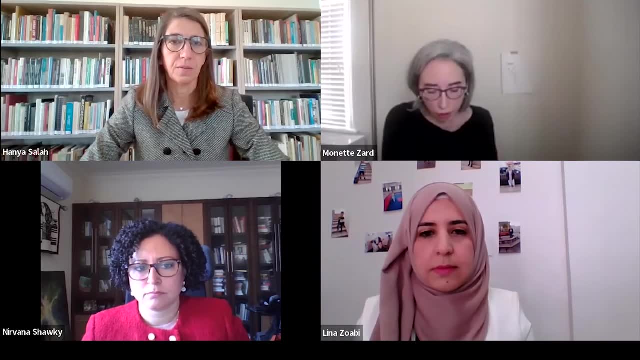 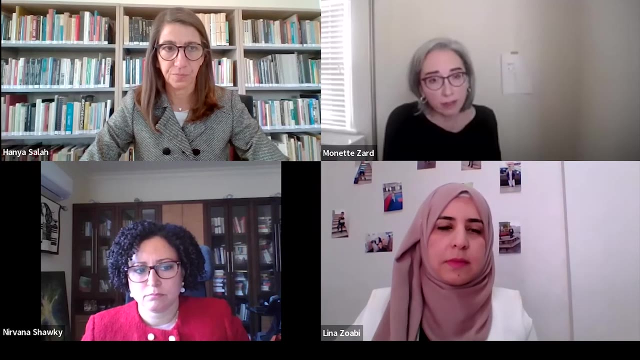 I think, as Hani alluded to, Employment of non-Jordanians, for example, is still limited to a number of primarily low-skilled occupations and sectors, primarily in the construction, agriculture, manufacturing and service, And there are, of course, gendered implications that flow from that, as the professions that generally attract women 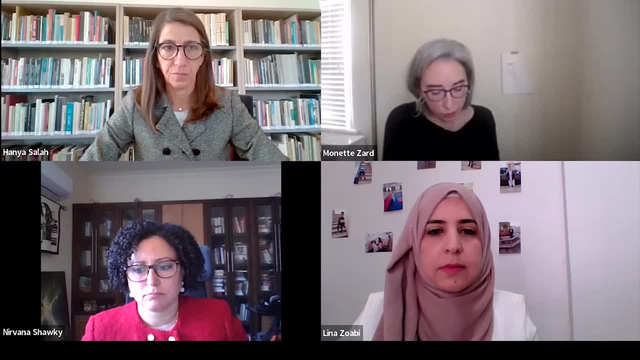 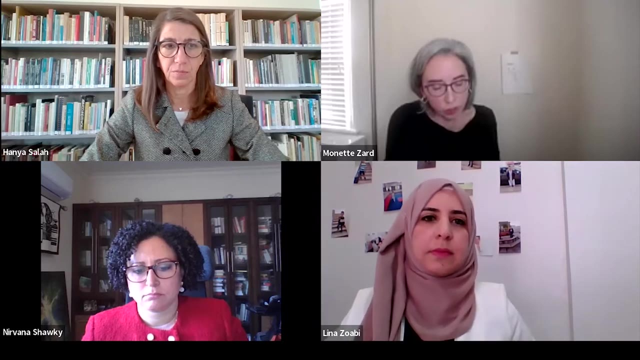 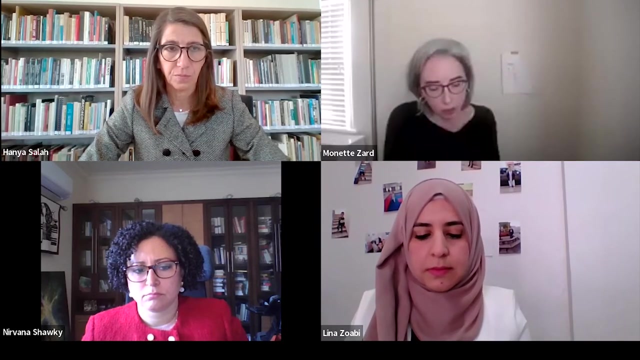 The list of closed professions actually expanded in 2020 to include vocations such as hairdressing, which have been a traditional focus of job training programs. Professions such as healthcare, teaching and business have remained largely off-limits to refugees, although, again because of the pandemic, to grant some exemptions for healthcare workers last year. 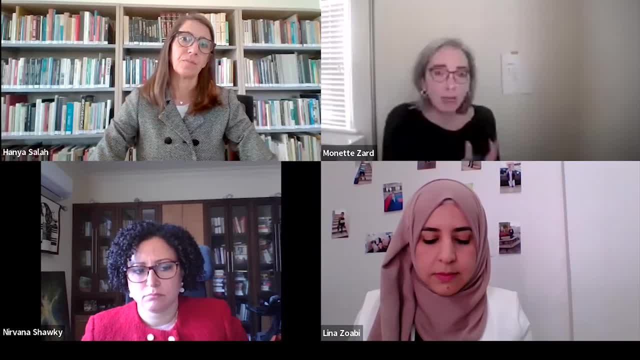 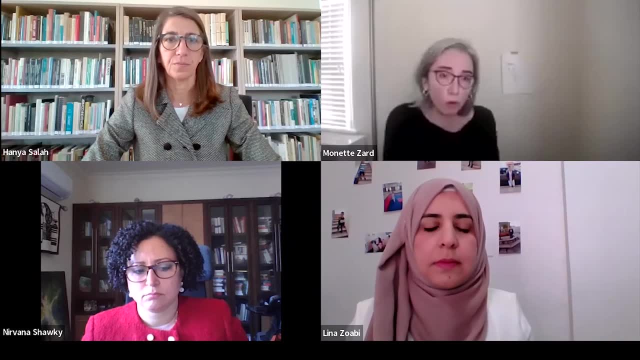 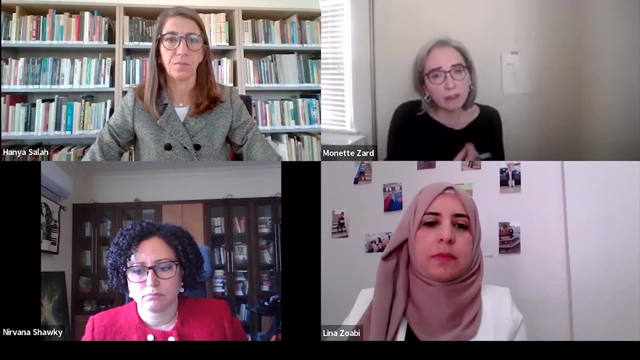 There are other barriers as well. There are unrecognizable, There are unwieldy procedures, lack of information and fees, which all together conspire to exclude refugees from the formal workforce. Also faced barriers to work alluded to really is relating to the lack of accessible and affordable transportation, issues to do with family obligations and childcare, and work environments that need to be cultured. 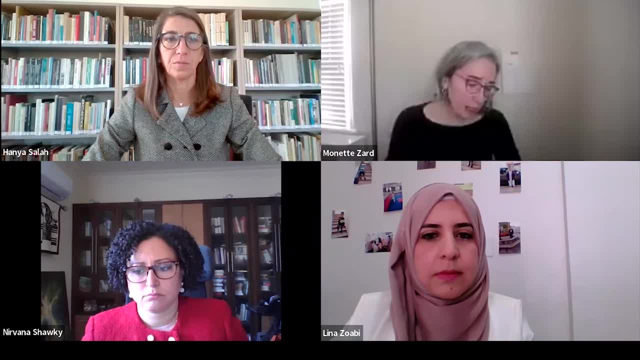 Also faced. barriers to work alluded to really is relating to the lack of accessible and affordable transportation, issues to do with family obligations and trafficking, and work environments that need to be cultured. Another area of particular concern is the policy and opportunity challenges posed on the 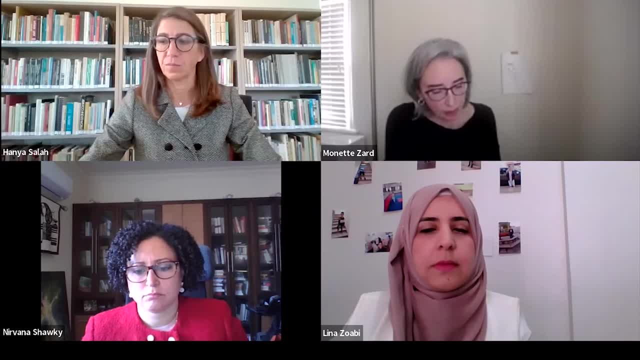 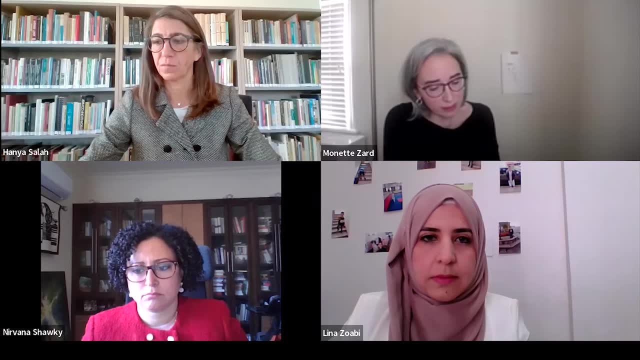 복 clutching of Bolivian feature issues andะ Claire. another area of particular concern is the poverty рын, claritystation and themadisson'slle 2009aben Yah Dehan, Media Appушки, Abuse Rules and your rights in Japan. Com, Tennessee. problematic sectors- care, poverty slicing and extradition- were last year pronounced particularly severe. でもmsi, Our nationalidéehity punto, There is suddenly a stretch of hard labor that is seen beyond the Sun as the distinct economy anymore. over the years, 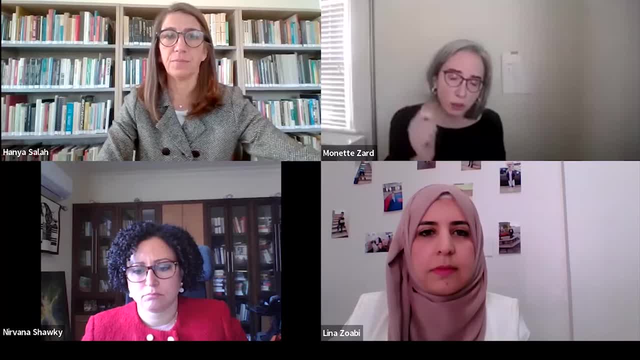 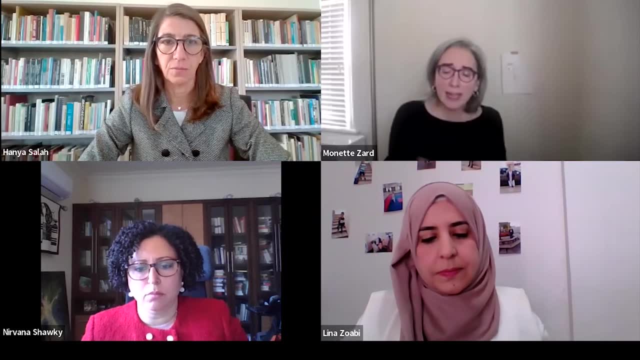 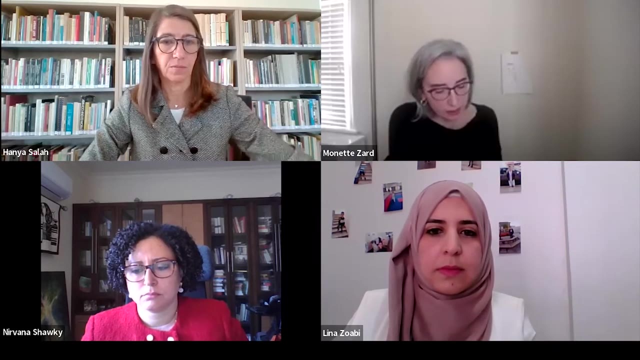 programs which are on offer throughout the region. but again, making sure that training is attuned to the needs of the labor market continues to be something of a challenge. so, against this backdrop, our distinguished panel today will help us probe and understand the strategy have been used to. 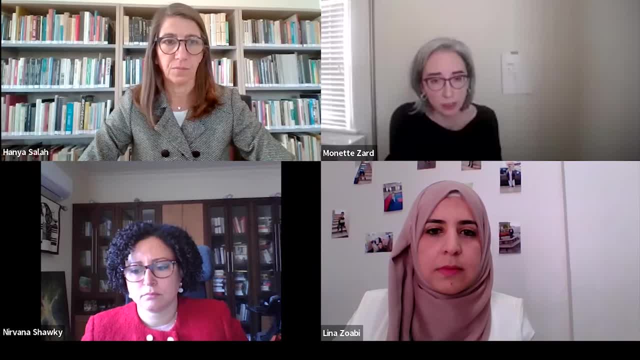 enhance women's participation in the work, the barriers that remain and the opportunities that are out there to really realize the full potential of refugee women to contribute to the livelihood of their families and to the economy as a whole. So our first panelist is Carolyn Ennis. 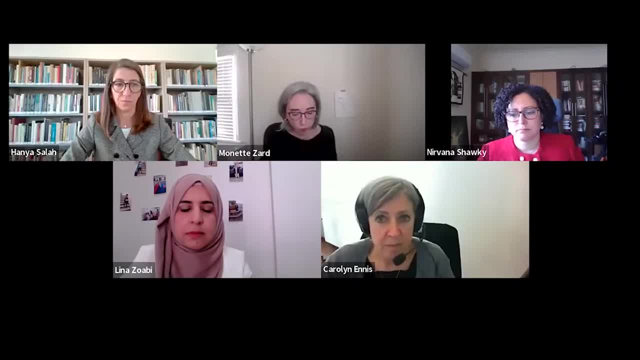 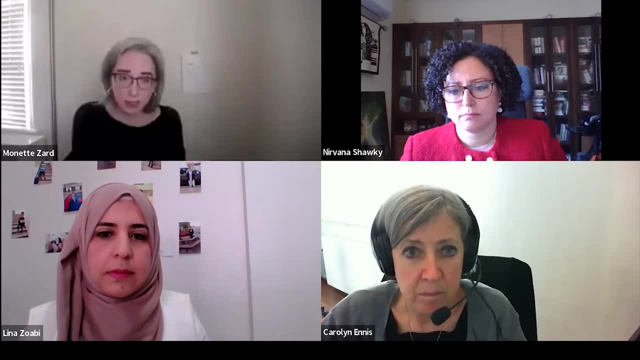 who is the deputy representative to UNHCR in Jordan. Since joining the UNHCR in 1999, she's served in the office of the inspector general as an assistant representative focused on protection in the Democratic Republic of Congo, as well as in Iraq. She's had positions in Turkey. 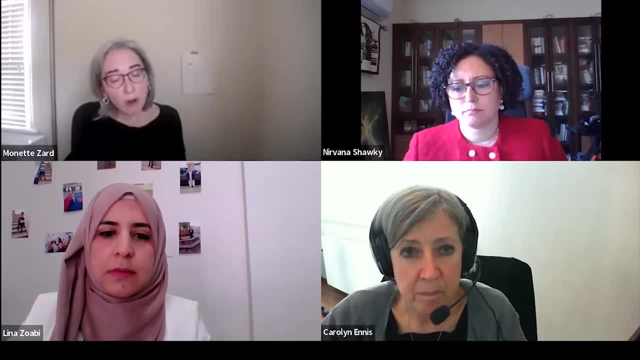 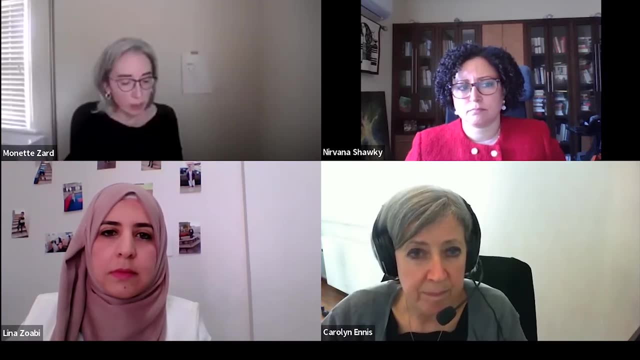 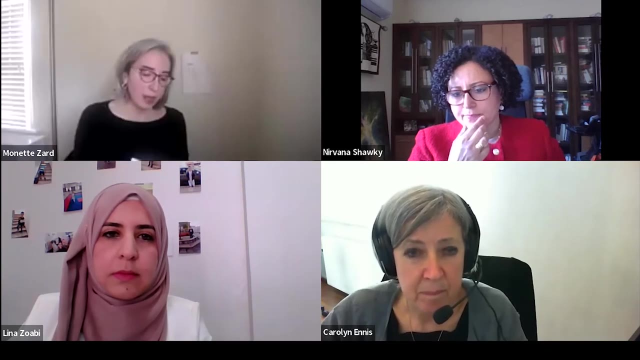 Africa and Egypt, and prior to UNHCR, Carolyn was a refugee officer in the US departments of Bureau of Population, Refugees and Migration, based at the US embassy in Cairo. She was an editor for the American Chamber of Commerce in Egypt and also for the International Council of Museums in Egypt. 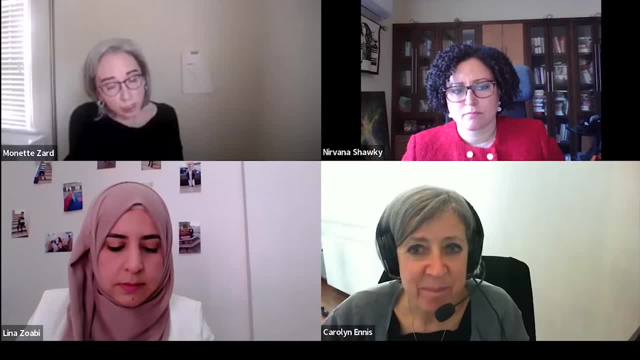 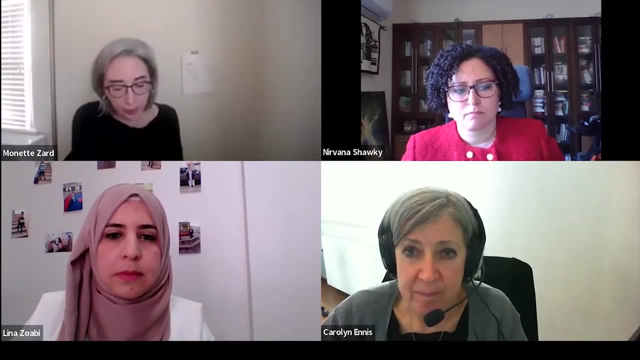 Our second panelist is Nirvana Shaoui, who is the regional director for CARES Middle East and North Africa region. Nirvana has two decades of experience working in the Middle East in multiple roles, from academia and media to advocacy and campaigning. Nirvana has served as regional 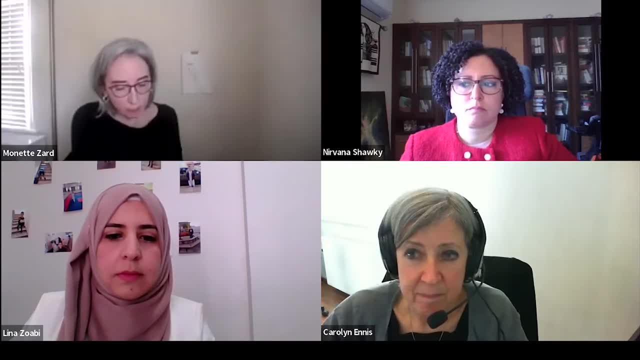 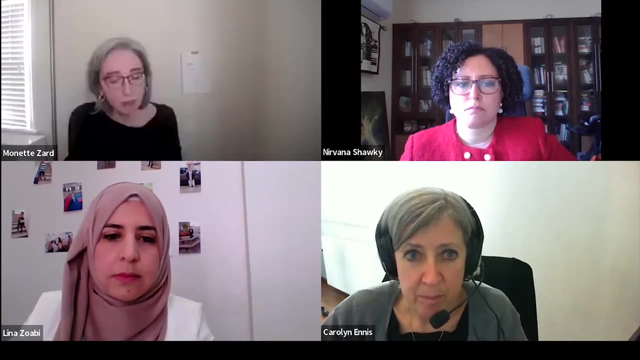 director of care since 2018, overseeing programming across 11 countries with a dual mandate in both humanitarian response and development. Before joining care, Nirvana worked with crisis action in multiple positions and most recently as international partnerships and director. As a regional expert on advocacy and conflict, she has led global efforts to protect. 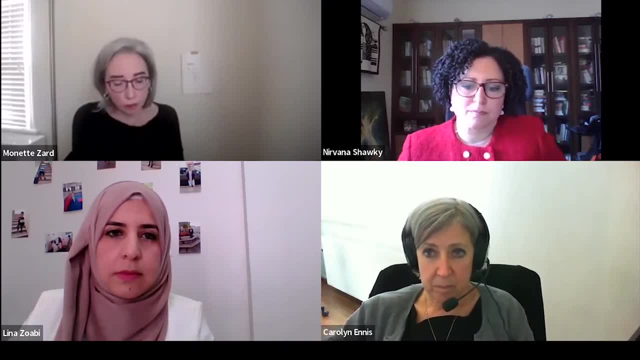 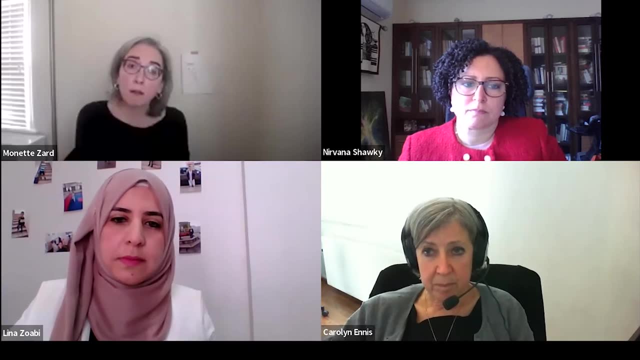 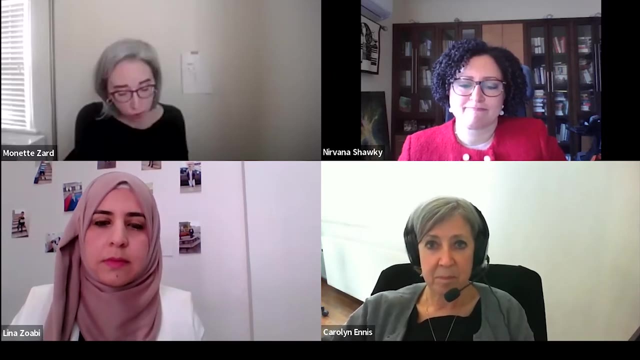 civilians and humanitarian crises in the Middle East, including advocacy on emergencies in Lebanon, Libya, Palestine, Syria, Western Sahara, Sudan and Yemen. Before that, Nirvana had a distinguished career in journalism. worked also as a researcher for Al-Ahram Center for Political and Strategic. 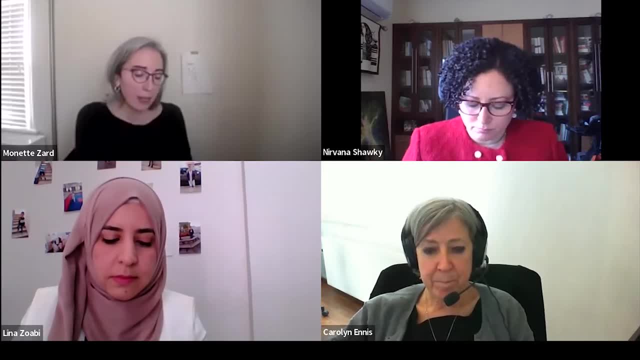 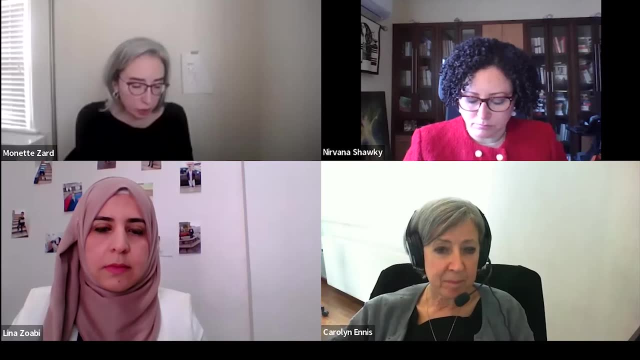 Studies and also as an academic lecturer. And our final panelist today is Lina Al-Zabi, who earned a master's degree in English literature from Al-Zaytuna University of Jordan and a professional diploma in refugee and refugee studies. Lina is a professor at the University of 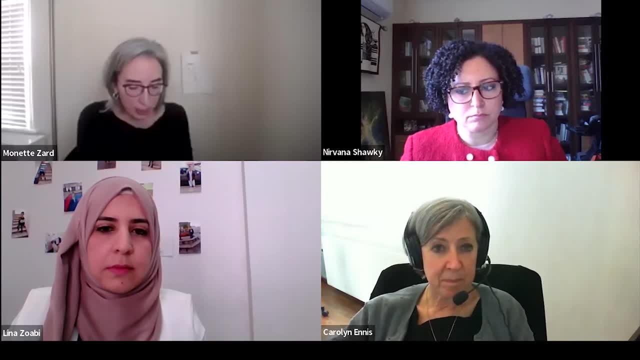 Jordan. She has a diploma as well in social work with a focus on refugees and migrants, from the German Jordanian University, And she's currently pursuing a PhD in English literature at Karabuk University in Turkey. Since 2015,, Lina has been involved in a variety of volunteer initiatives. 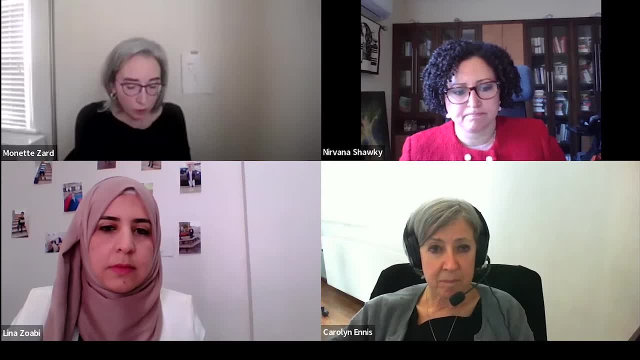 with refugees in Jordan and collaborates with a number of non-governmental organizations, And we're going to talk a little bit about her. Lina, thank you so much for joining us. Recently, she launched a social initiative called Hopes Beyond Borders: Refugees' Unheard Voices. 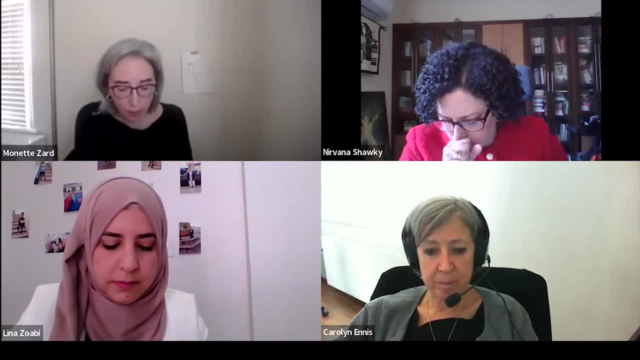 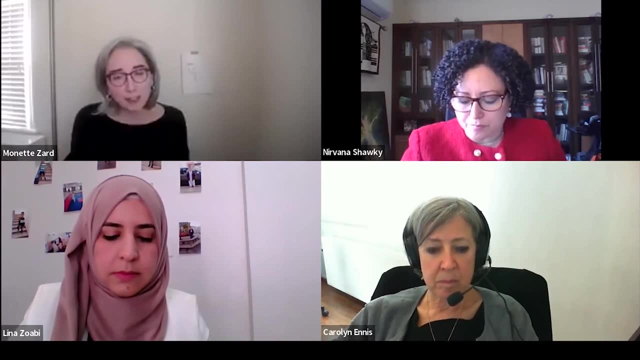 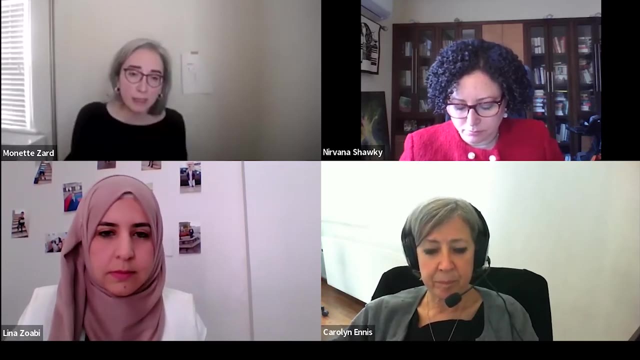 in a bid to provide every refugee with an online platform to make his or her voice heard. So just a reminder: we're going to have a conversation as a panel for the next 40 minutes to our audience. If you'd like to pose any questions, please put them in the Q&A. 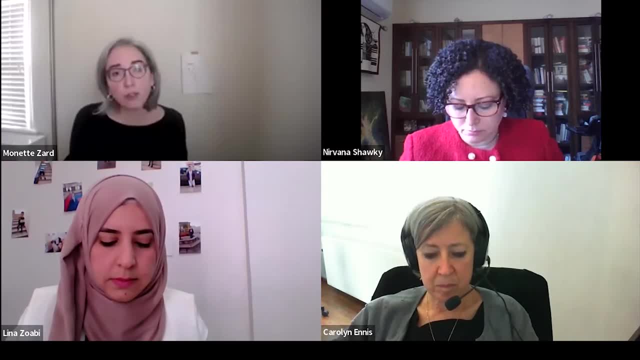 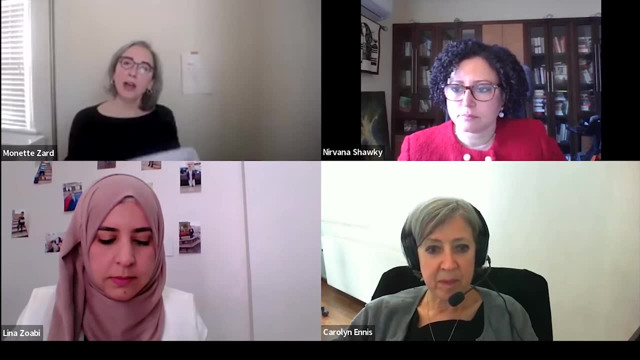 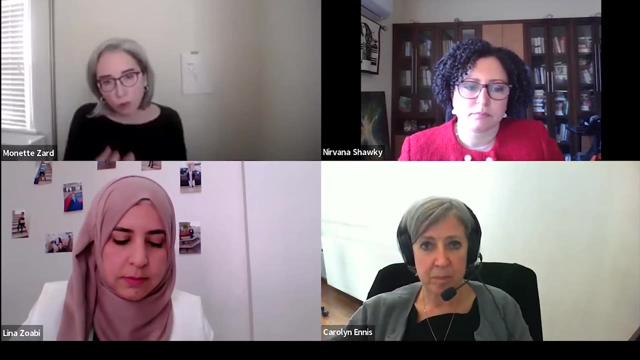 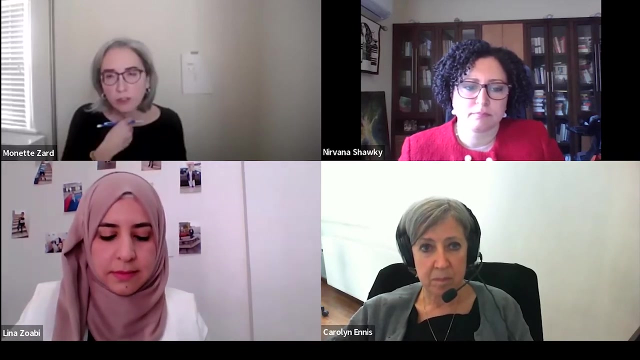 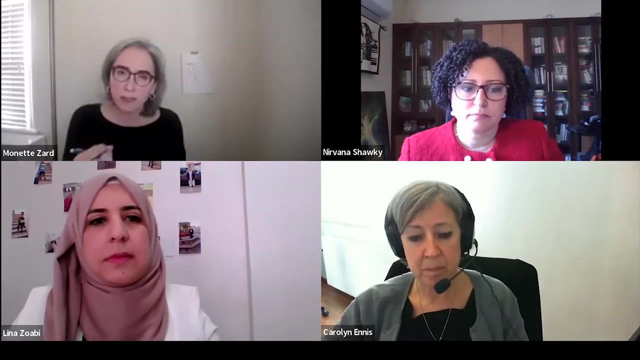 and we will allocate some time towards the end of the session. So let's begin with Carolyn. Carolyn, can you help us set the context for this and then really take a look at the region and give us your analysis, sitting from the perspective of UNHCR, and what the current livelihoods context looks like for refugee regions and how UNHCR really 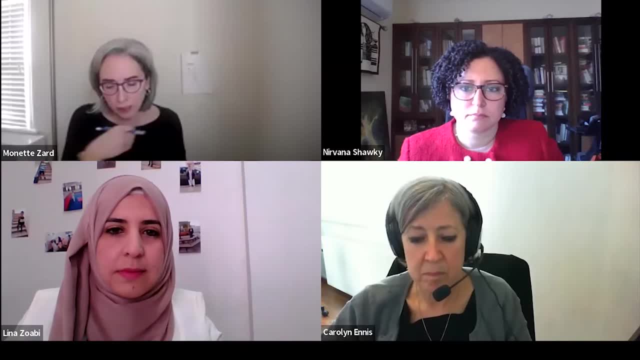 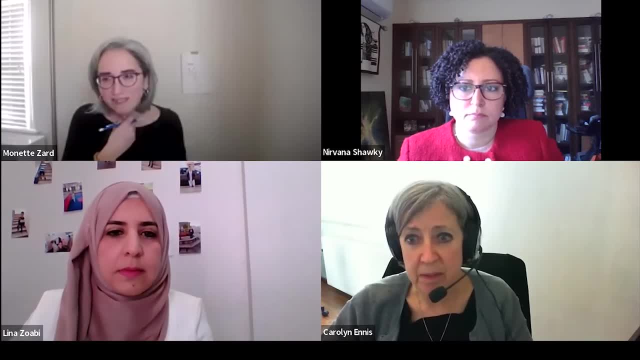 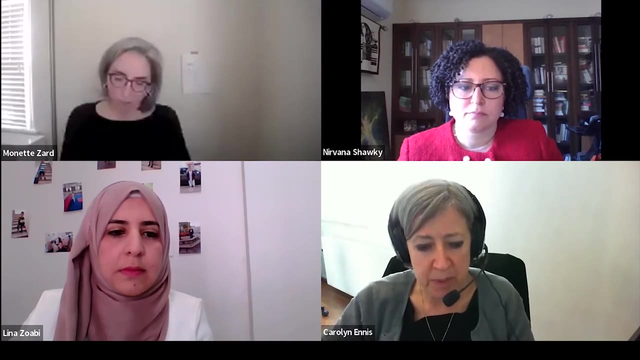 Well, thank you so much, Manette, for the excellent introduction and also for including UNHCR in this panel. The region is still home to the largest refugee crisis in the world, and UNHCR- UNDP- are working with more than 270 partners to try to address the needs of 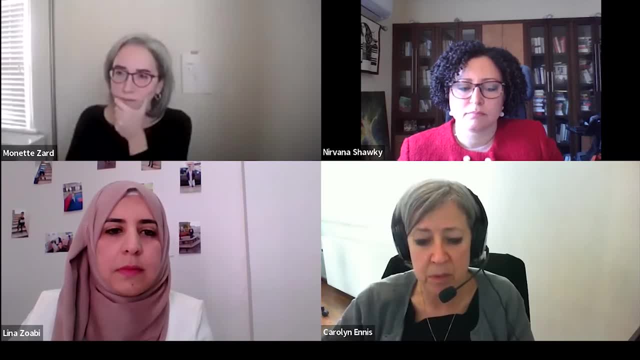 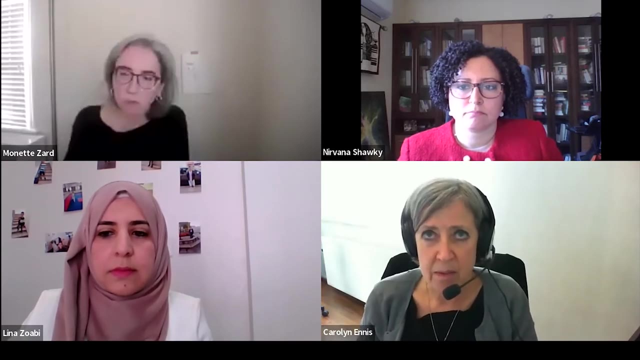 approximately 7.1 million refugees, asylum seekers and stateless persons, including 5.6 million registered Syrian refugees, in Turkey, Lebanon, Jordan, Iraq and Egypt. So we work closely with partners throughout this response, and let's just take a minute. 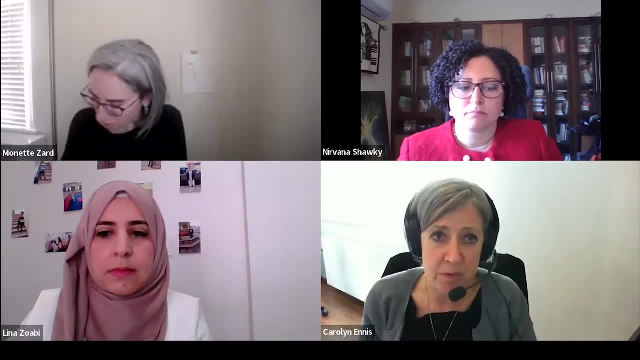 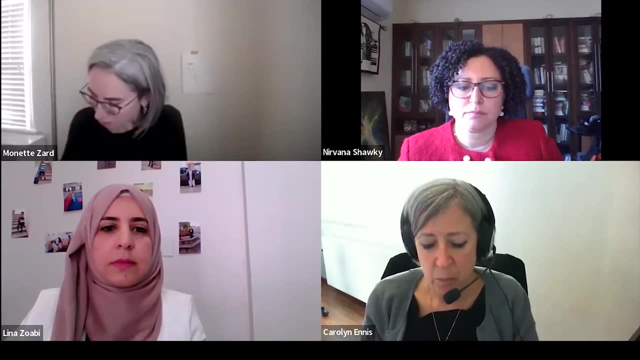 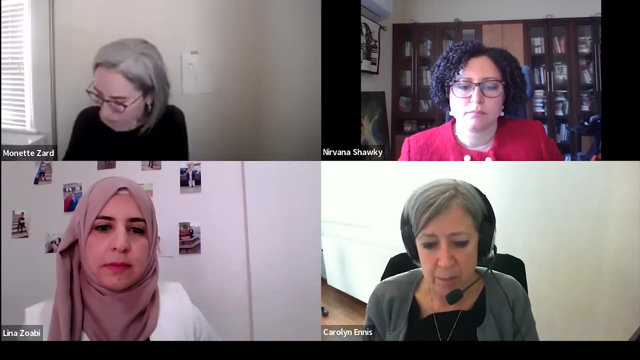 to reflect that behind these numbers are people who've been forced to flee, and thus we call them refugees. And in the midst of this situation, women. everyone has specific needs, but particularly women and children and a very, very high number of youth. We recognize that host countries face 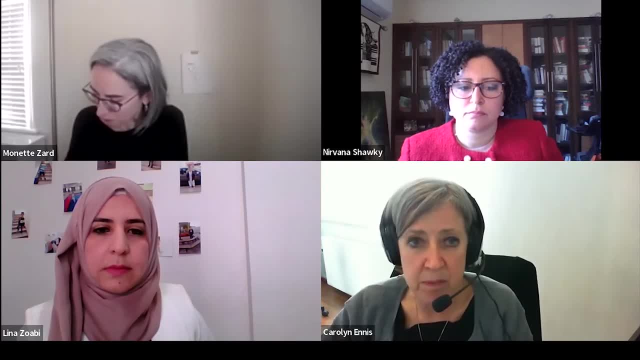 enormous pressures at a level not seen since the onset of the crisis because of COVID. The 3RP countries have been facing enormous pressures at a level not seen since the onset of the crisis because of COVID. The 3RP countries have been facing enormous pressures at a level not seen since the 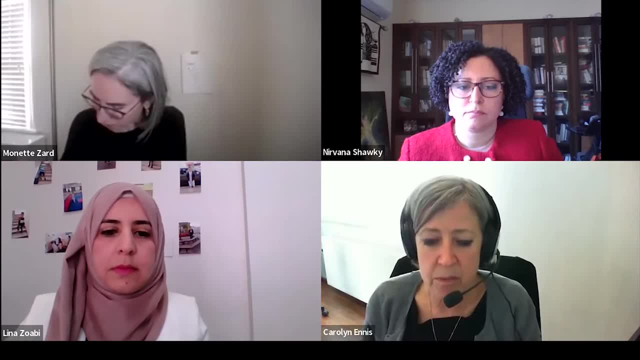 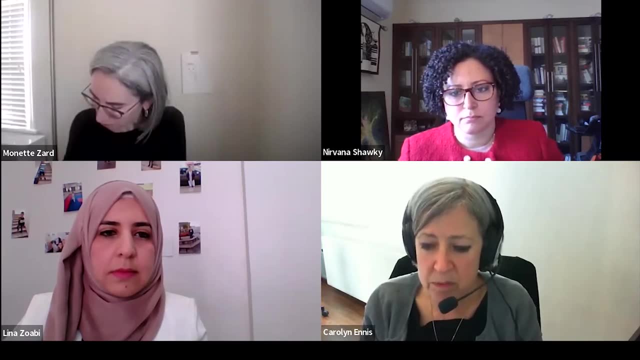 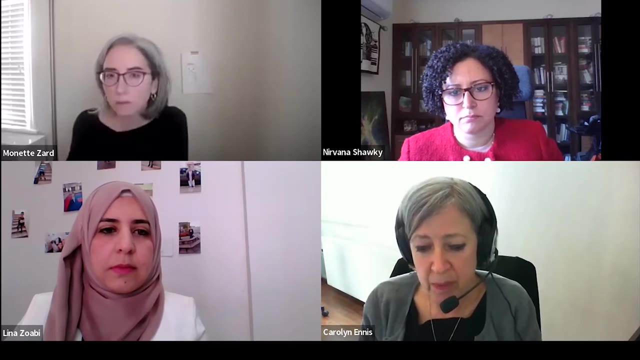 onset of the crisis because of COVID, The 3RP countries, the ones I just mentioned, continue to face varying degrees of socioeconomic crises, exacerbated by COVID-19, and, in some cases, coupled with political crises Since the establishment of this response mechanism, particularly amongst the host community members. 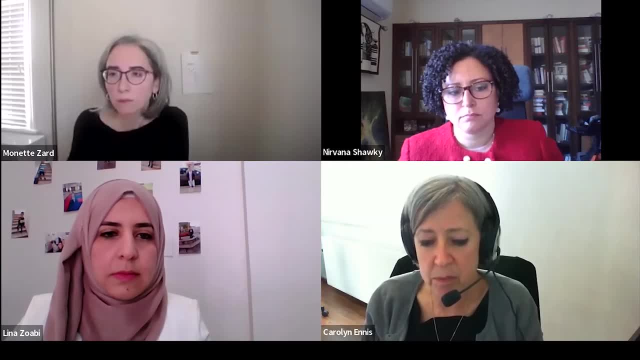 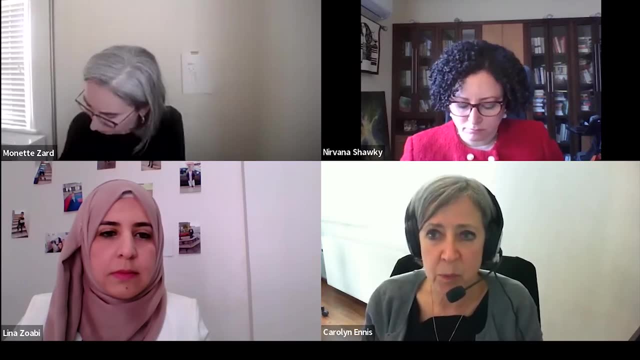 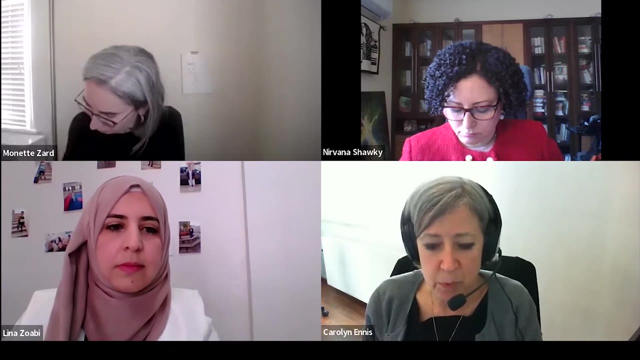 the number of people in need has approximately doubled since before the COVID-19 pandemic, due to the socioeconomic impact and increasing vulnerabilities, And this is the area in which refugees women- Syrian refugee women- are trying to support themselves and their families. So, on the big strategic level, yes, we have the numbers, the registration. 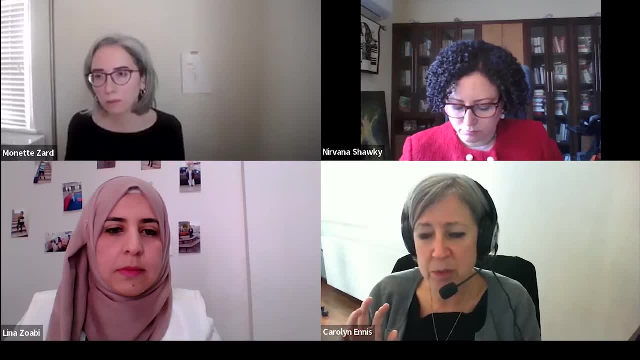 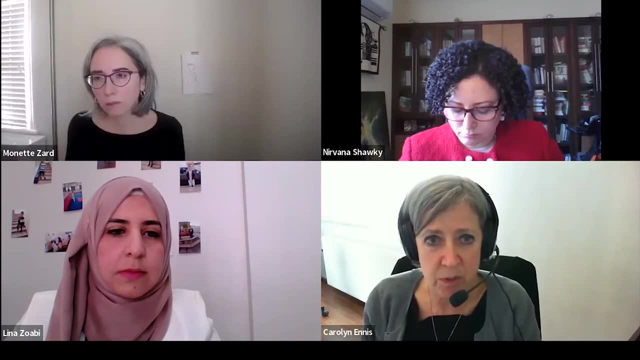 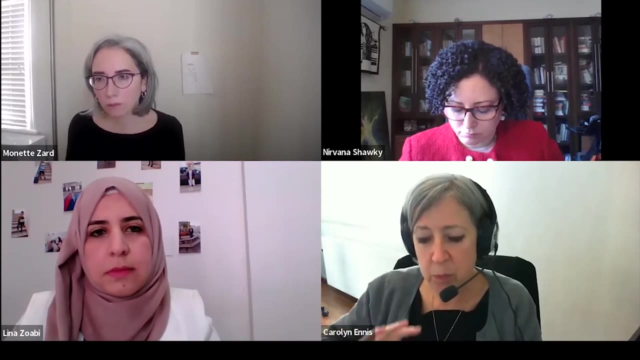 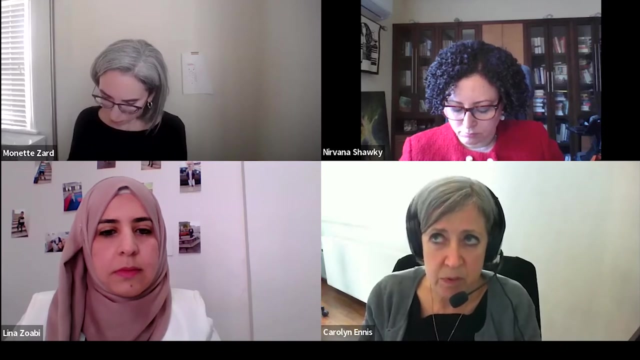 the partners, and we do, as a protection agency, have a strategy developed with our partners that's really grounded in international refugee law, in the principles of the Global Compact on Refugees and which speaks to the Jordan Compact, And within this big framework, we try to have programs that are set up to really support both refugees and host communities. to 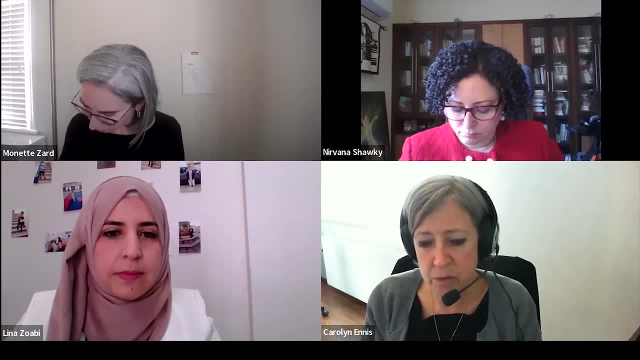 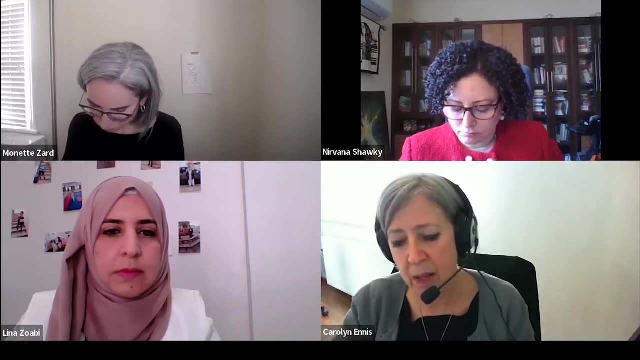 support social cohesion and really try to foster the resilience and the capacity of refugee Syrian refugee women and all the other people who've been impacted. The specific areas that we've highlighted as challenges to be overcome are the recessions, the rising levels of unemployment and poverty, worsened inequalities, particularly putting the 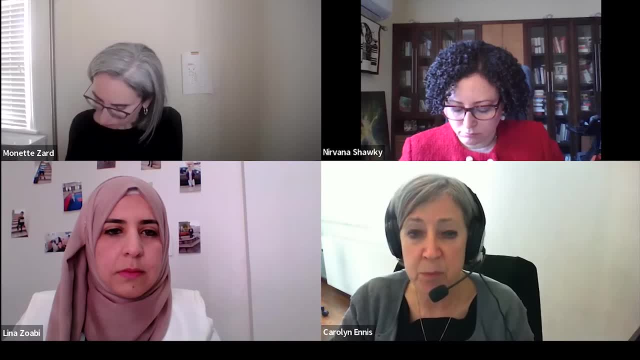 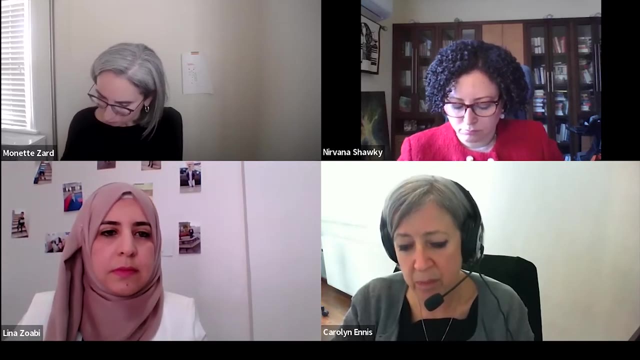 vulnerable population groups back. We had a lot of people, especially in Jordan, who were almost managing, but after COVID they're back into extreme poverty, Food insecurity, increased dependency on what is still unfortunately limited humanitarian assistance. This has led 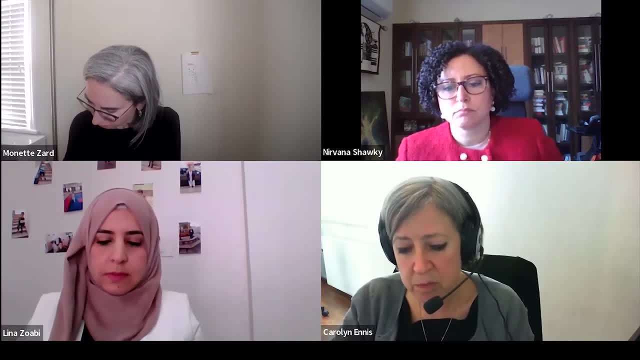 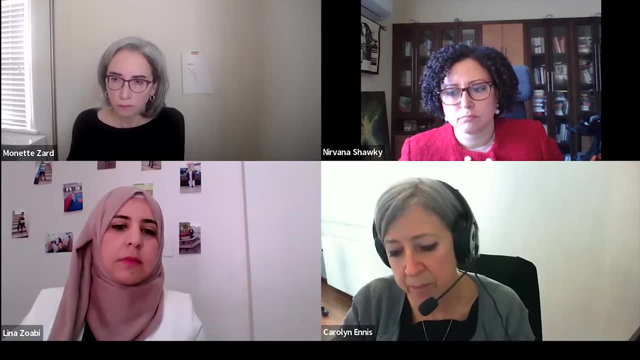 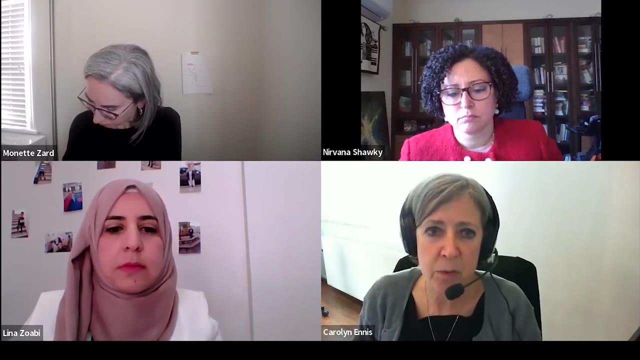 to evictions, higher debt, income losses coupled with the absence or limited capacity of social safety nets. in most of the countries that we're looking at, This has also brought on increased mental health, a whole variety of serious protection issues, which lead to what we call. 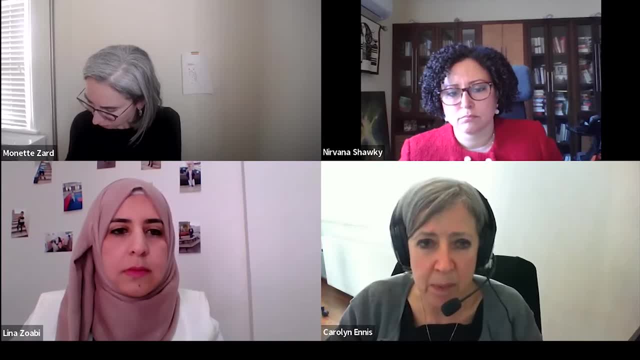 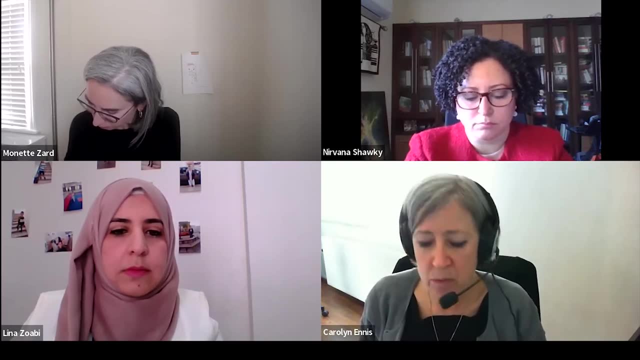 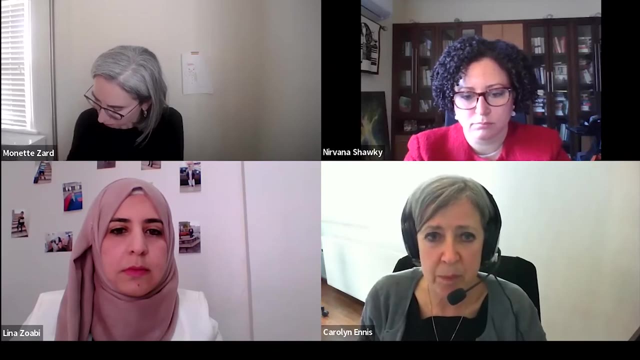 negative coping mechanisms which place far more burdens on the refugee women that we're talking about. So we have a whole range of strategies to try to support resilience in the community. with our partners, We provide cash assistance, we provide training and we also try to really highlight the capacity and potential of 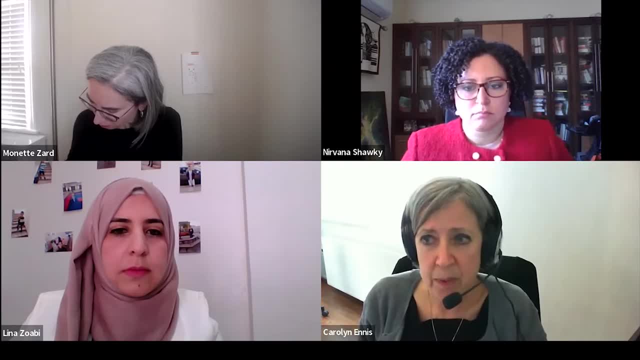 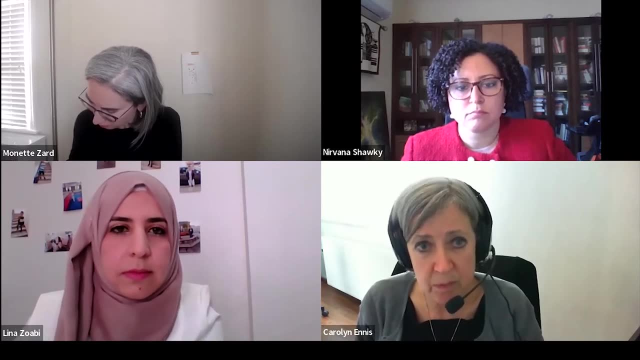 the refugee population, particularly the women. But we also have to note the social constructs which often make it difficult for refugee women to go out and work. This is often a new role, particularly for Syrian women here coming from Daraa, where they 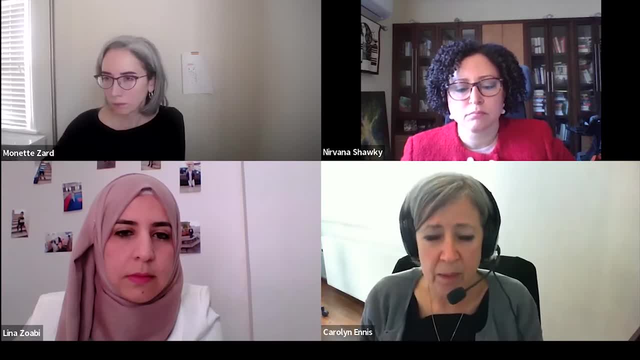 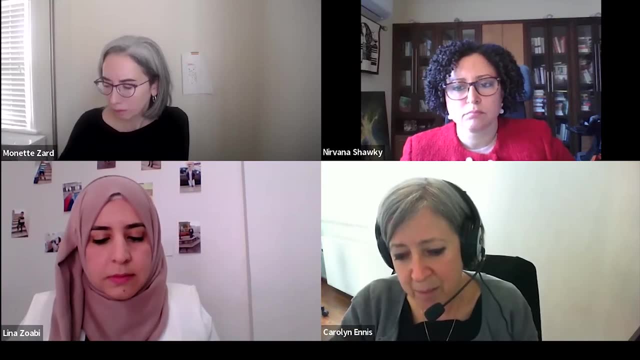 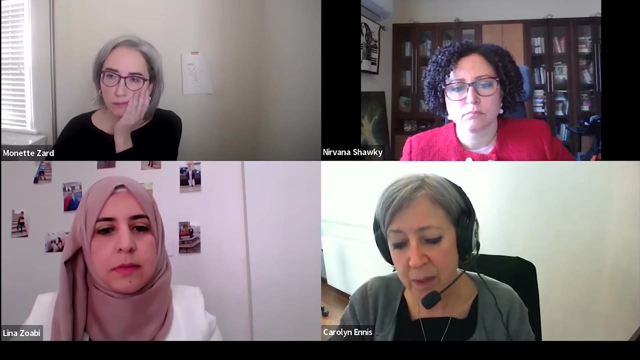 were not necessarily working before, and even social constraints against working. More and more refugee women have started to work, And what I'd like to really emphasize is that we're trying to help people to become self-reliant, but we have so many really talented women, a lot of potential. 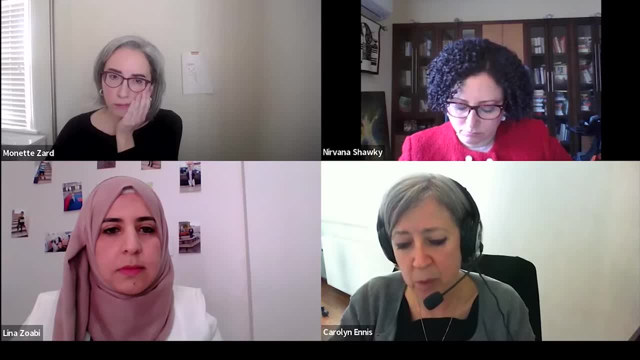 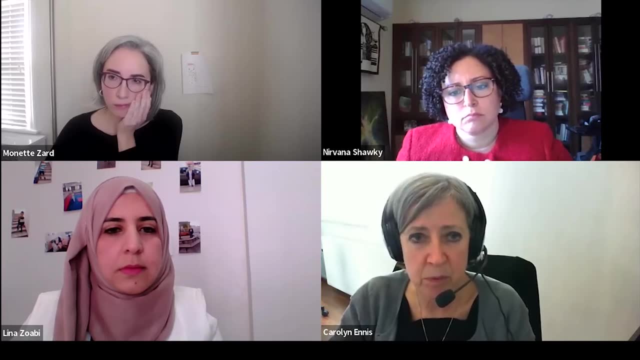 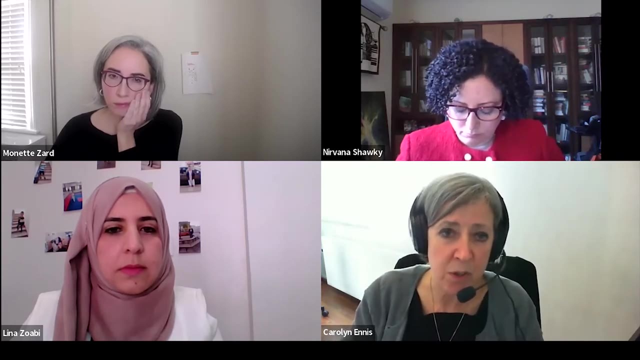 a lot of skills who want to make contributions- qualified architects, teachers, people qualified in law and medicine and a lot of women who are also working in the less-skilled areas, And we're trying to really leverage opportunities in each country where we work to target refugee women and really 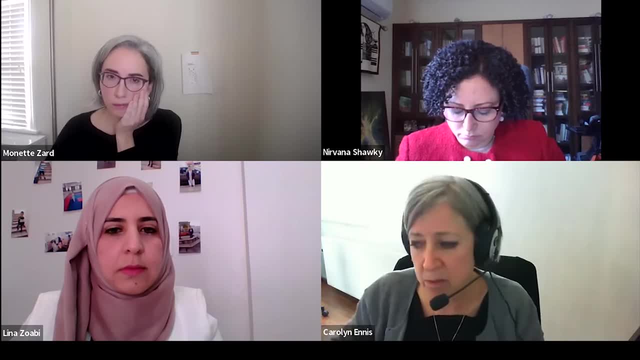 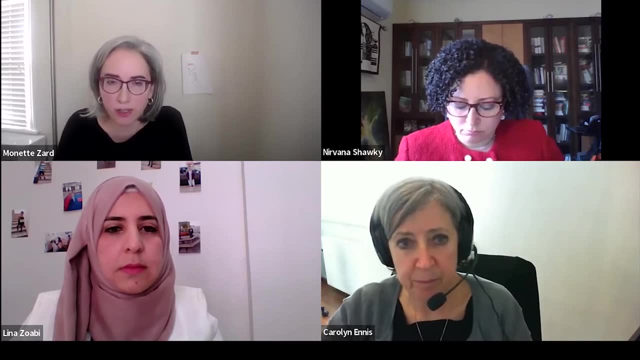 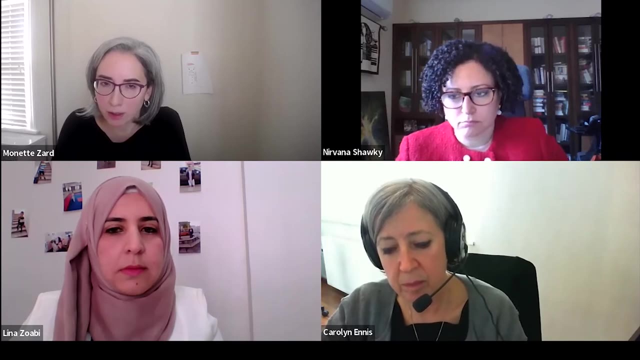 support the refugees and affected populations as a whole. Thank you, That's just very helpful and sobering sort of foundation for the discussion. You alluded to the Jordan Compact And we discussed the Global Compact on refugees as well. Could you talk a little bit more about what the sort 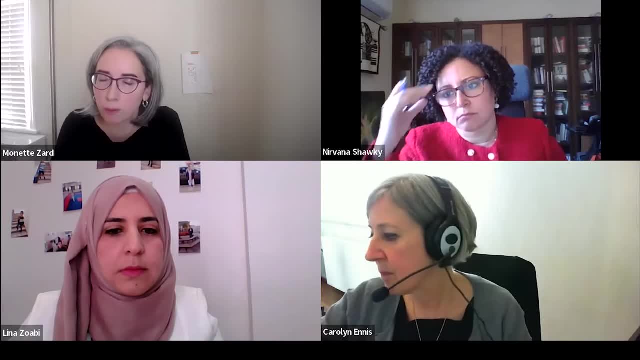 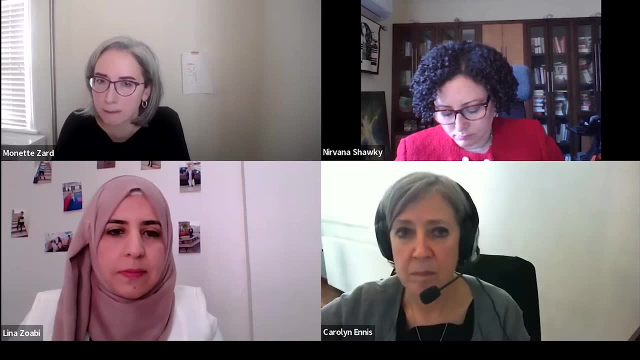 of broader policy commitments are at the global and the regional level the UNHCR uses to sort of frame its work on behalf of refugees. Well, let's see At the Jordan level, yes, Across the board in the context of the Global Compact. 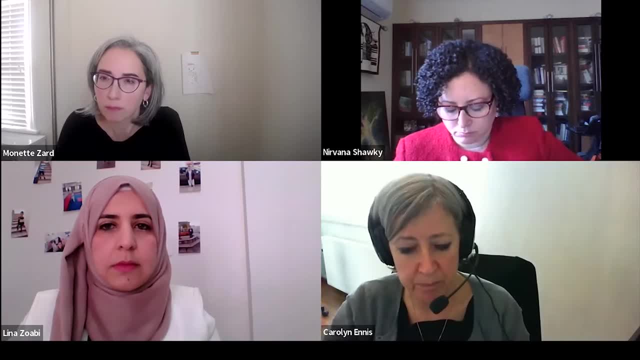 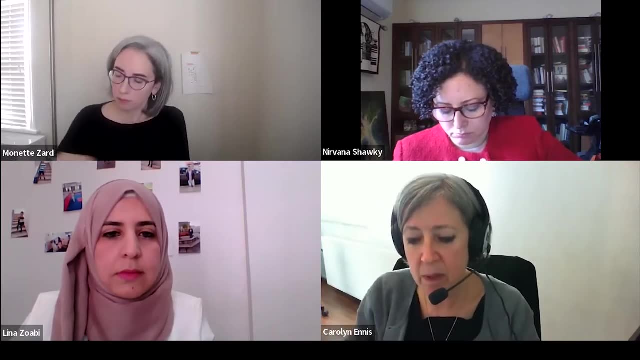 that's a big part of the identity of the Jordan Compact Pope, So being accessible to other incredible people. Heidi titled these workshops where refugees were publishắt compact on refugees. So let's look regionally first at the Global Refugee Forum, States and. 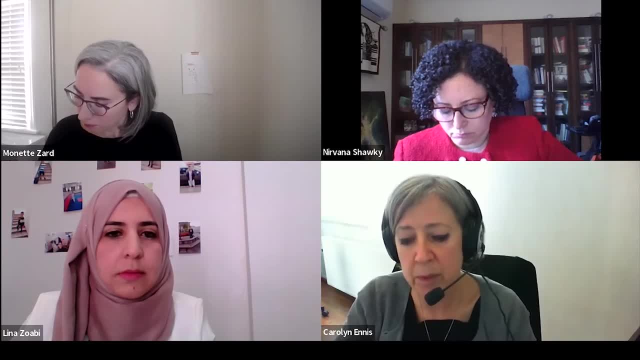 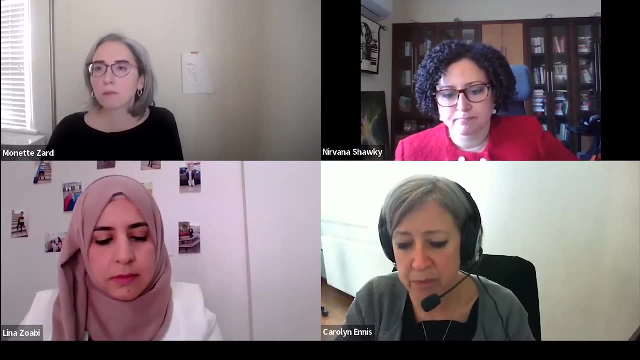 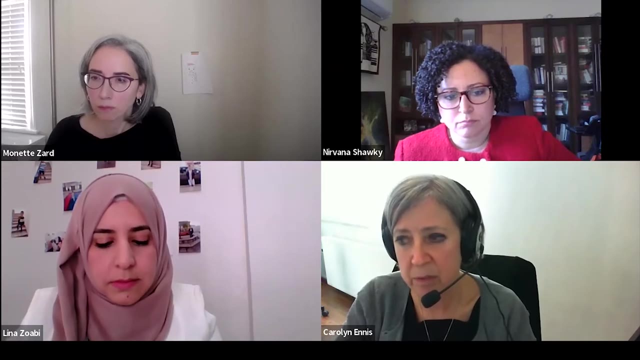 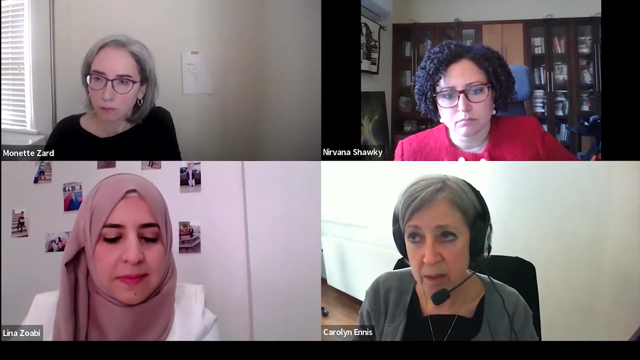 other stakeholders submitted pledges to foster inclusive economic growth for refugees and host communities through decent work, job creation and entrepreneurship programs. Of the total of 140 pledges, 40 are reported in progress and planning are already fulfilled. So globally and in the region, we're really trying to support access to decent work for refugees and for the vulnerable. 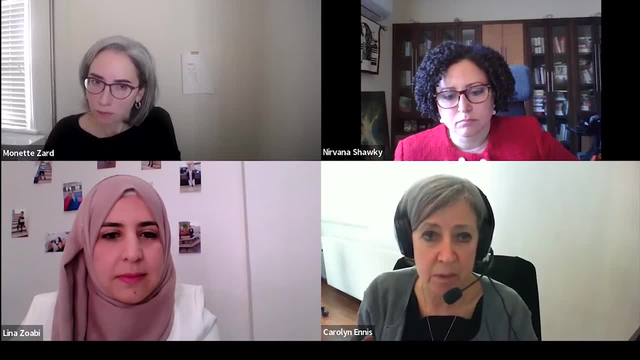 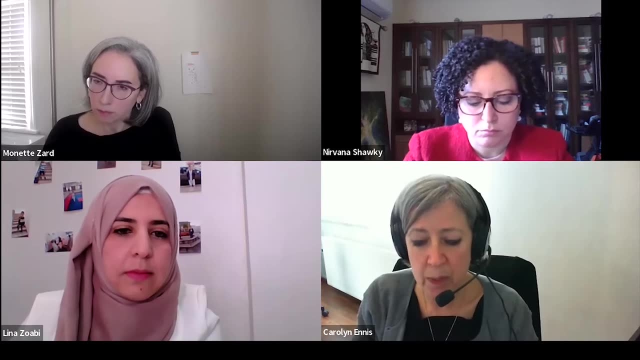 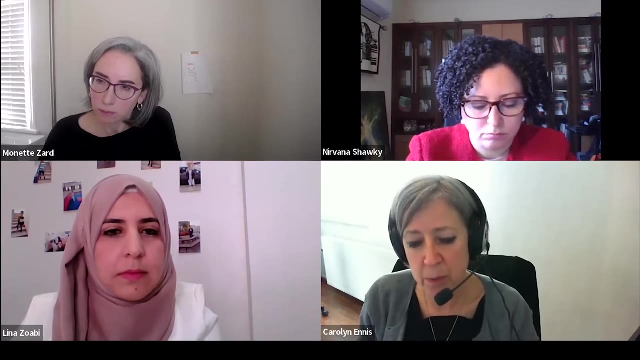 host communities And, obviously, because of their vulnerability, we are really looking very closely at women. And then, when we come to the Jordan Compact, this was a really forward-looking initiative And we've seen a steady improvement in the rate of issuance of work permits and access. 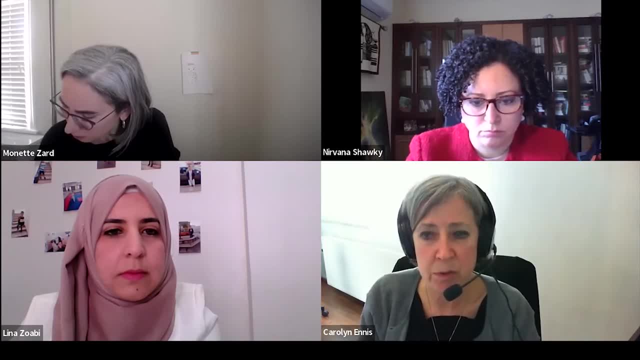 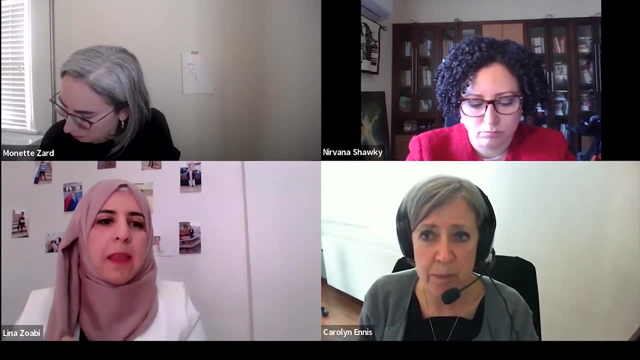 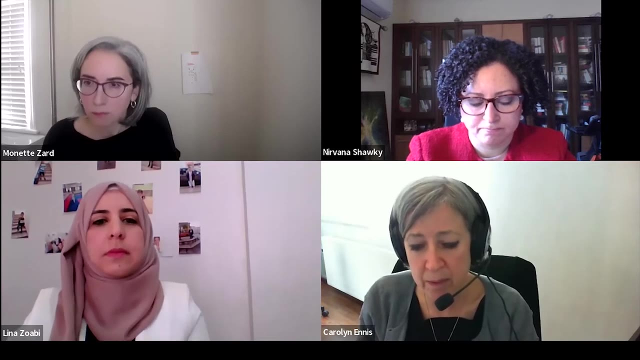 to decent work and a new development in Jordan, The Social Security Corporation, through which refugees can actually pay into a fund which will provide some protection And if they become unemployed, they should actually get some protection rather than going back to depending on cash-based interventions. 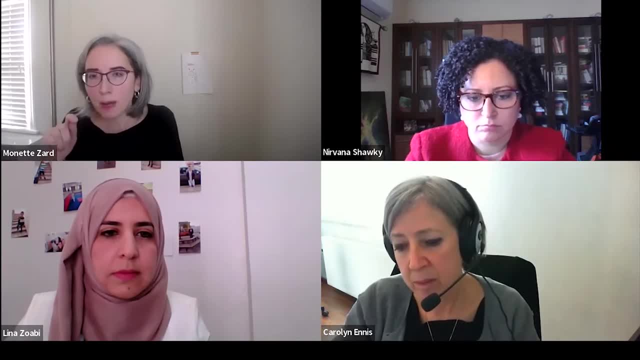 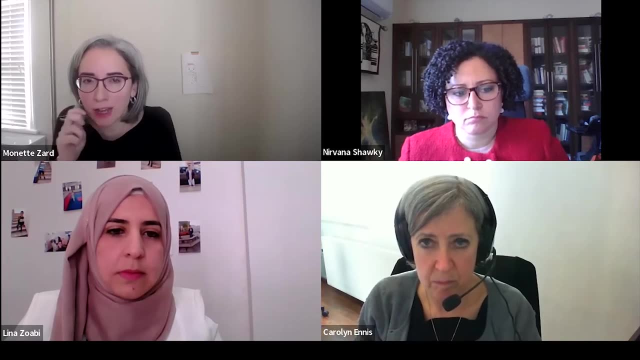 Very interesting. Thank you, And just perhaps to round out your initial comments, could you give us just a flavor? Yeah, I mean, I think it's really interesting to hear what UNHCR's programming on the ground looks like. Are there one or two sort of emblematic initiatives that you hold up as what you would? 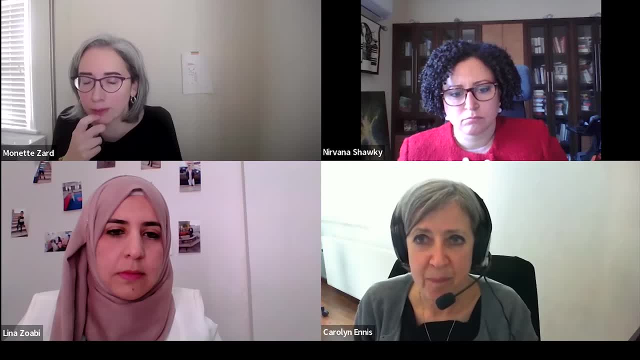 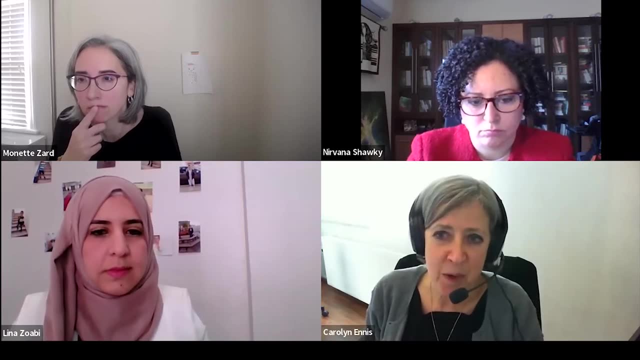 like to do more of in the livelihood space for refugee women. This is actually really exciting and we're really proud of it. I think maybe the most emblematic one is the groups of women plumbers who were working in Zaatari. This is an unconventional 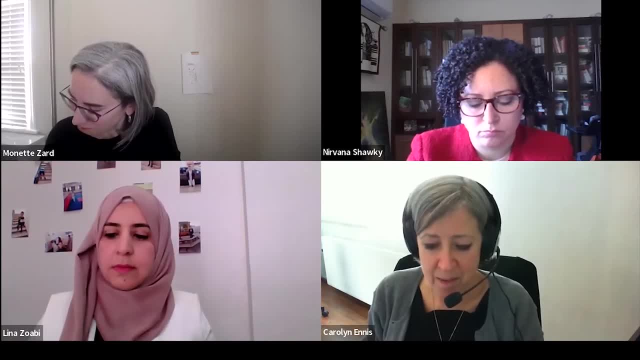 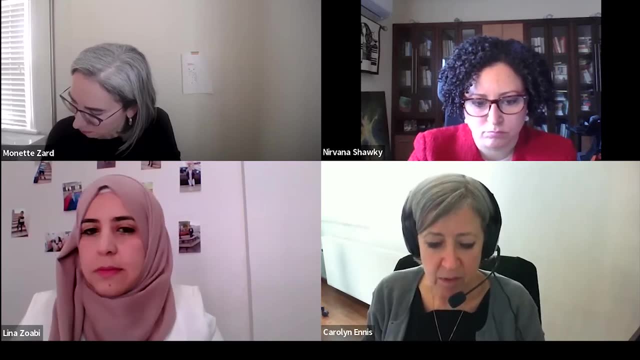 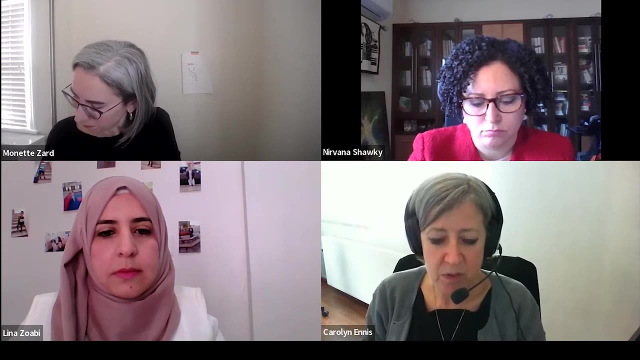 non-traditional area where there's a huge demand, But we have identified young women, qualified architects. There are refugee UN volunteers working as engineers and we've had refugee contributions, including as healthcare professionals who contributed to the Jordanian government's response during the COVID pandemic. 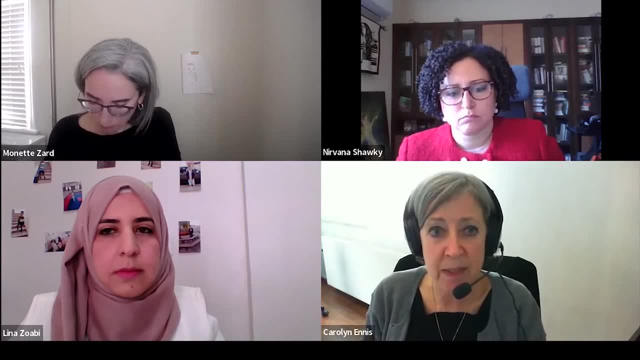 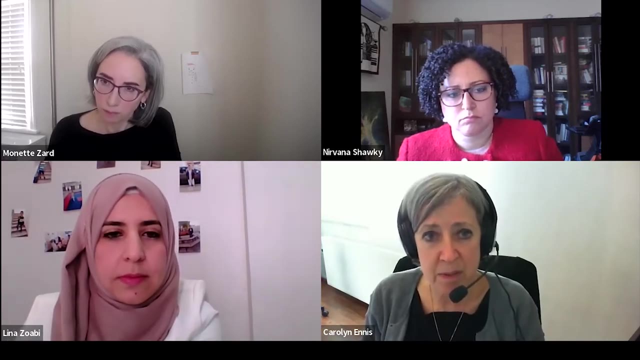 And this is something where we really welcome the government's inclusive, inclusive approach to including everyone in their territory in their COVID response And, at the same time, we were really proud that there were highly qualified medical professionals who were refugees, who also participated in and were employed by the Ministry of Health. 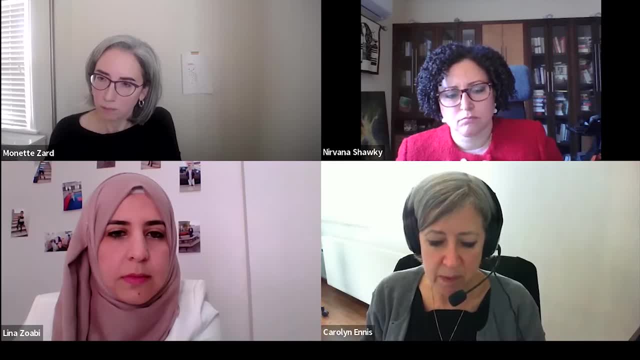 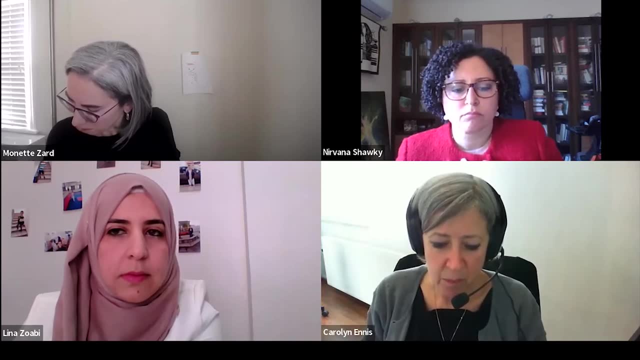 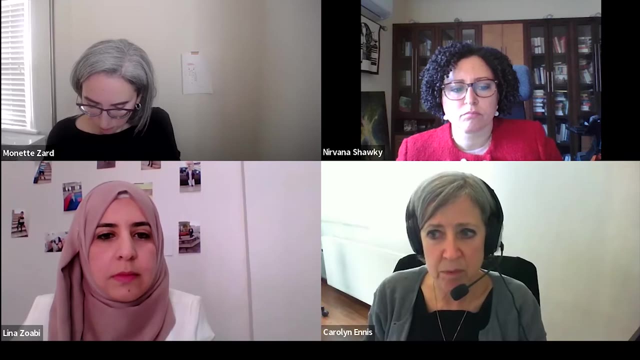 But across the board, we've been trying to support women in home-based businesses, because many, particularly Syrian refugee women, are more comfortable in these areas, And we're also trying to look at ways to strengthen women's empowerment and look at the challenges that confront both. 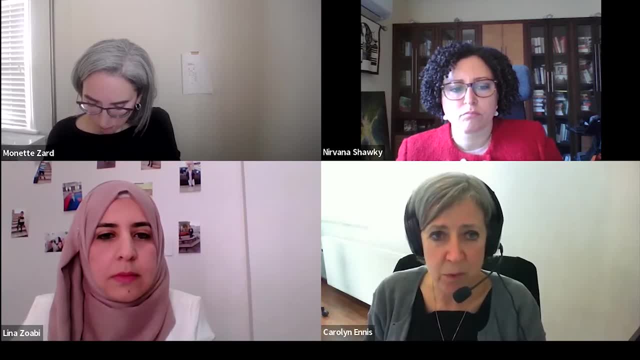 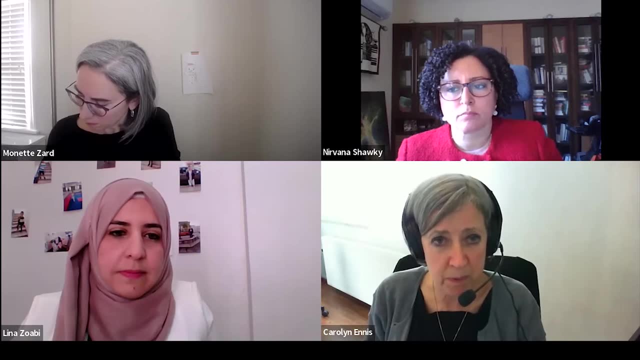 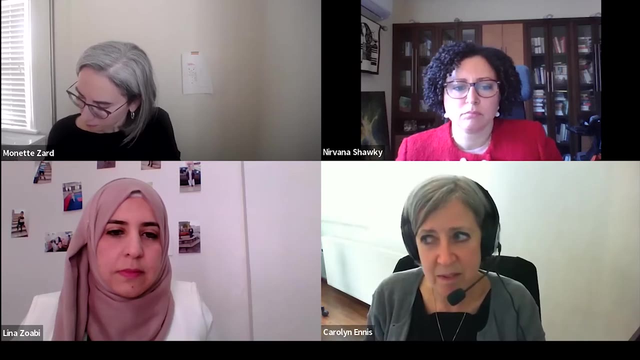 refugee and Jordanian women, difficulties in transport and problems with sexual harassment- which, of course, is something that's very hard for people to report and talk about, but is a reality, And so we're really trying to support, you know, this very promising and energetic population that. 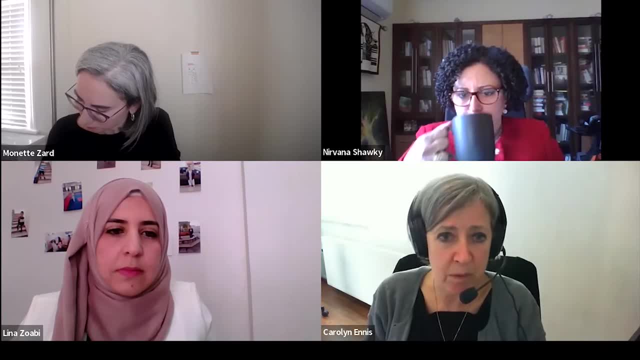 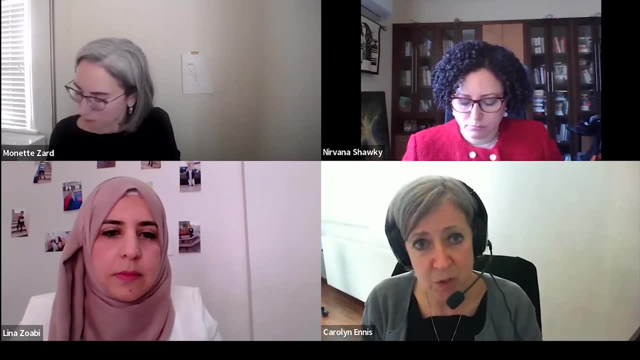 is eager to work and contribute. So we're trying to look, with our partners, at as many different entry points as possible, both for the less skilled and also for the more highly skilled refugees And, if I can just mention, the Global Compact on Refugees. 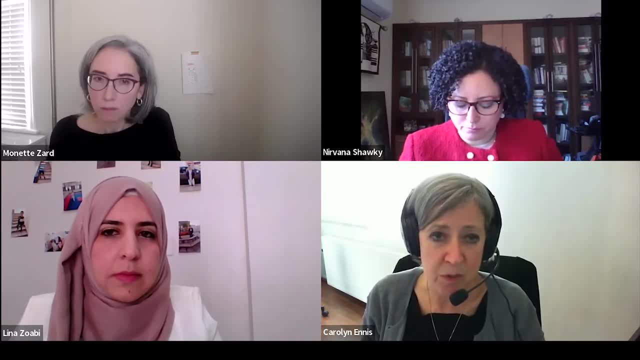 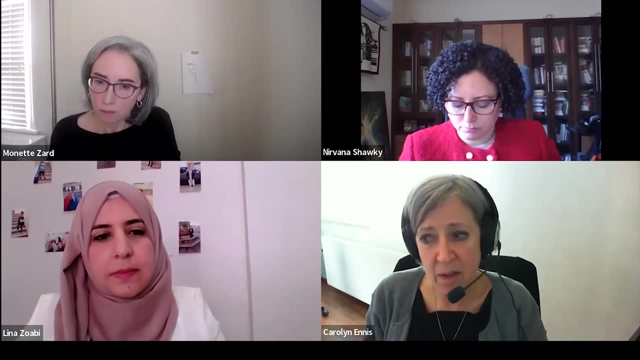 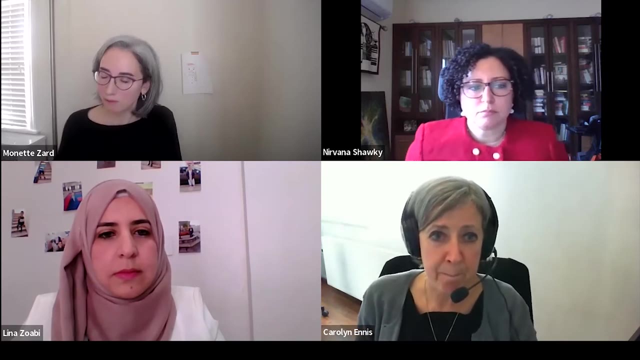 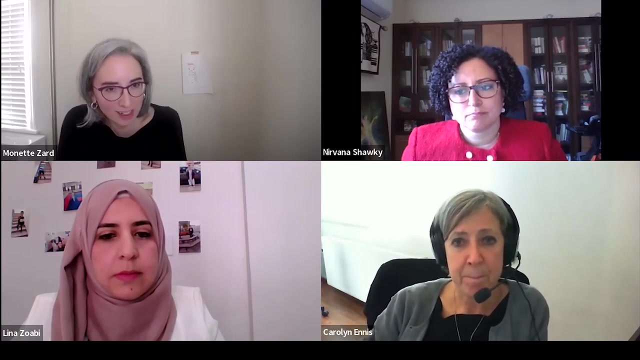 our commitment to support governments who host refugees, but also to look for more places for resettlement and complementary pathways, because these again provide opportunities for refugee women and girls amongst others. Really really encouraging and interesting initiatives. Thank you so much, Carolyn. If I might, I will move to Nirvana now And Nirvana. 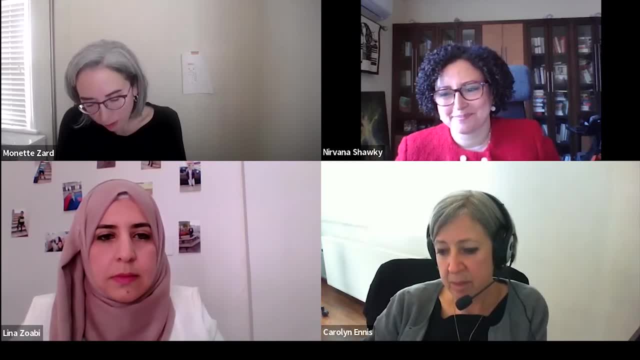 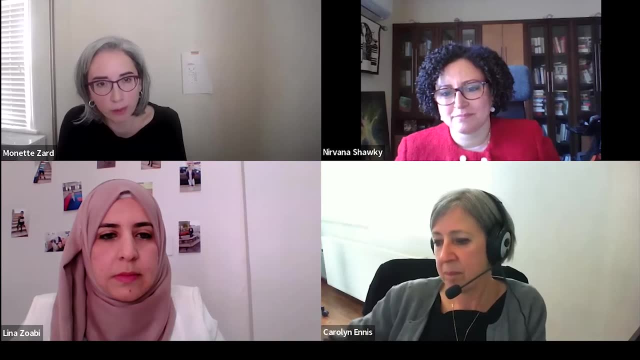 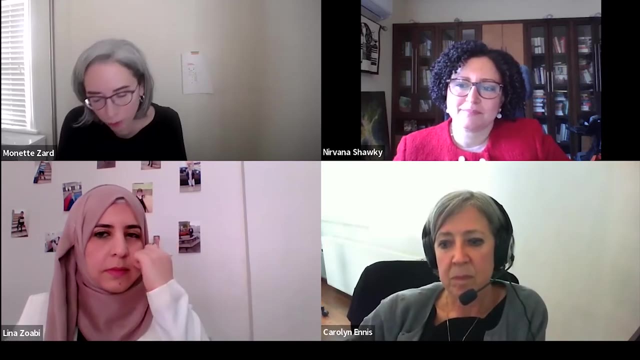 welcome. Ask you perhaps to reflect a little bit on what CARE has been doing through its programming to enhance women's workforce participation in the MENA region. Syrian refugee: women's participation in the MENA region: What strategies have you used? What sectors are you targeting through your work? 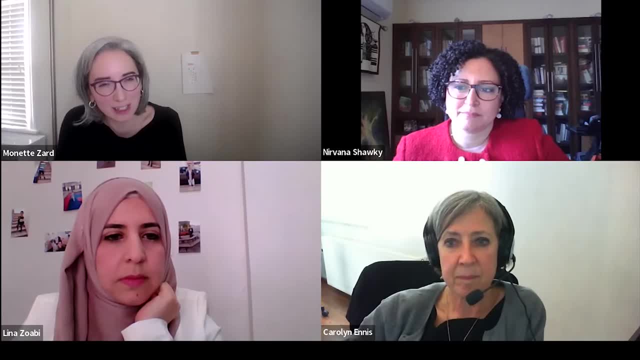 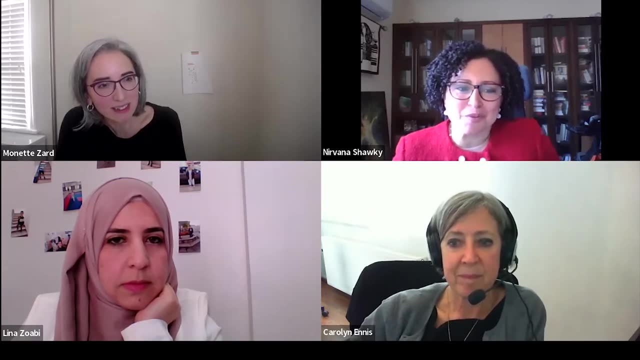 And really, if you can, what does success mean and look like for you? Sure, sure. Thank you, Moneta. Thank you so much to Columbia Global Center for this workshop and this partnership. It's an absolute pleasure to speak to you today. 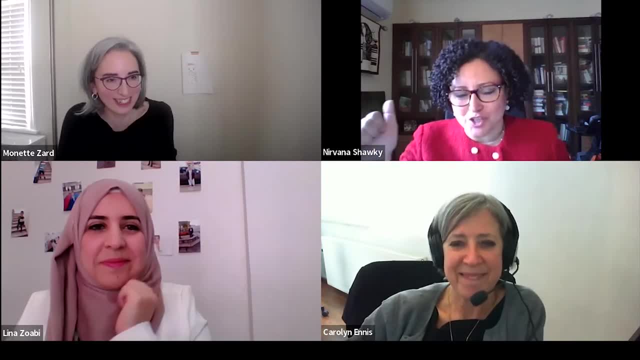 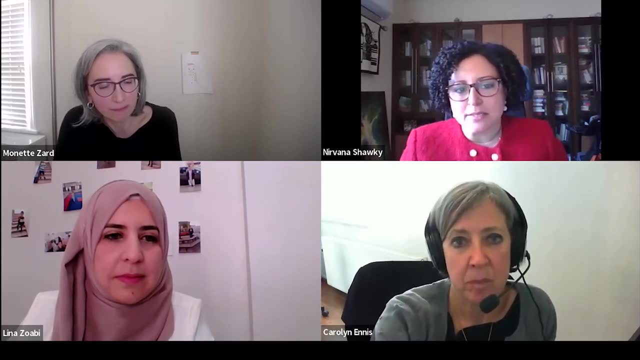 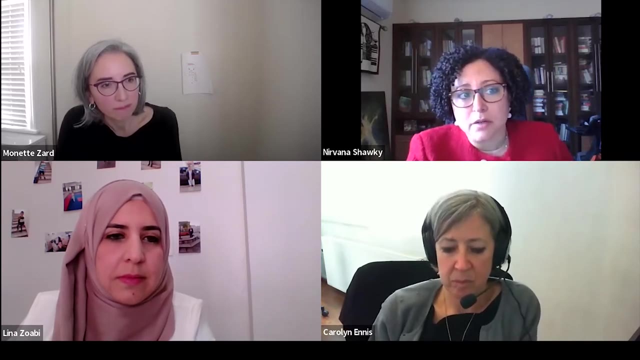 Can you just confirm that you can hear me well, because I mean, the voice was shaky. Thank you, Perfect, Perfect. Allow me to start by By stating that care actually has been working on and on the Syrian crisis since the beginning of the crisis. 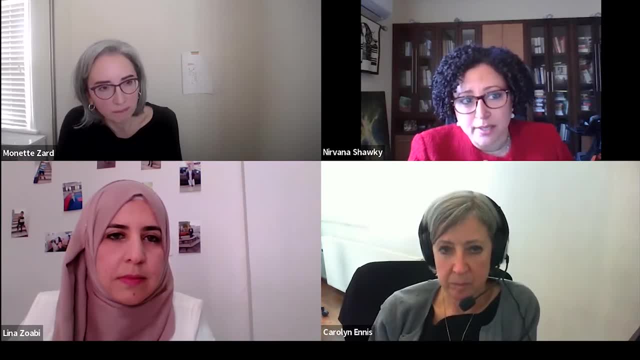 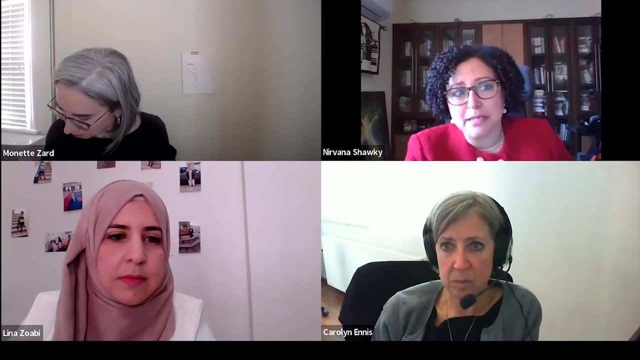 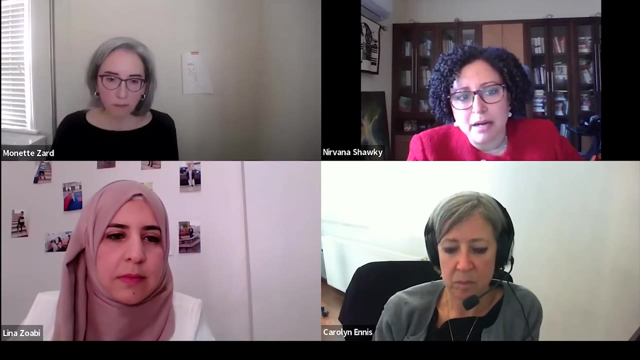 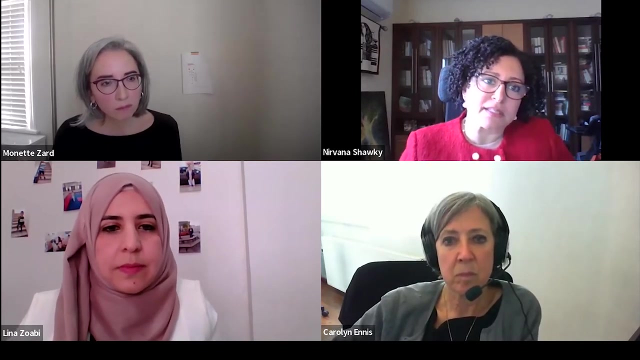 And it's been really an uphill journey for caregiving. I mean the fact that it is the crisis of our generation and especially here in the Middle East. this has been actually one of the defining shifts for our programming after many years of mostly focusing on our development work in the Middle East. 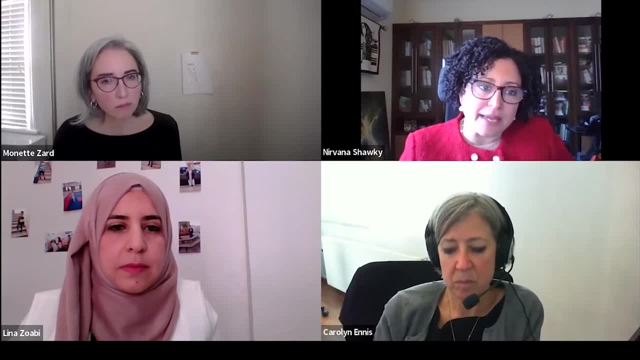 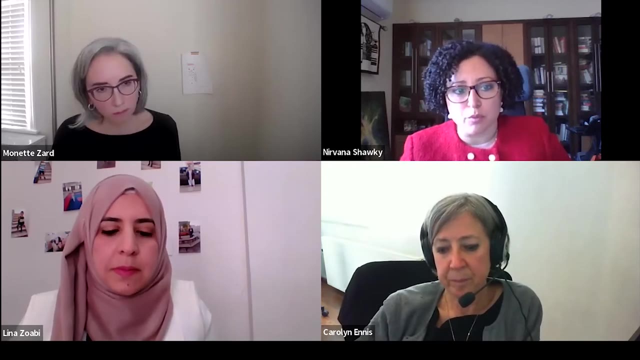 giving. I mean the nature of the needs we had in the region. We had to really shift our gear very, very rapidly when the crisis took the uphill and we had to really shift towards a more dual approach focused on both humanitarian response in addition to long-term engagement. 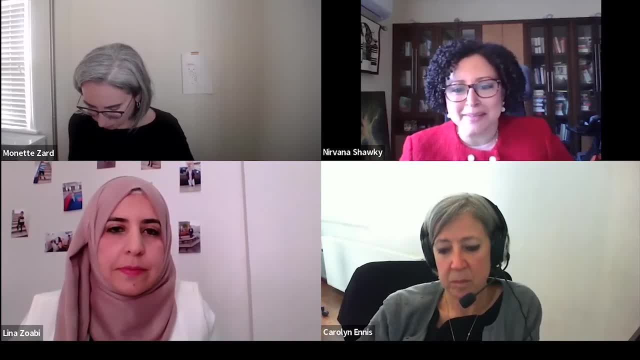 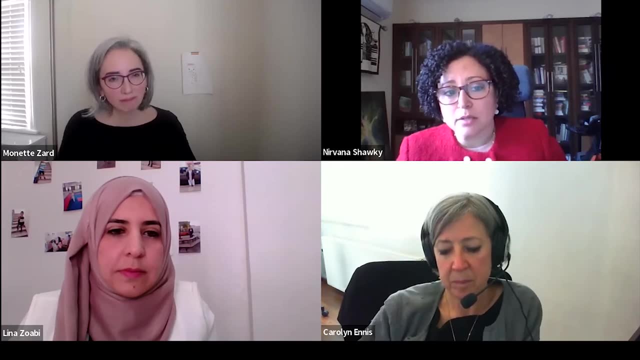 And the conflict, as you all know. I mean, I assume that some of the facts and figures I'll be sharing are already known to a lot of people on this webinar, but some of them are also particular to care's work. So, as we all know, the conflict in Syria has displaced 12 million people. 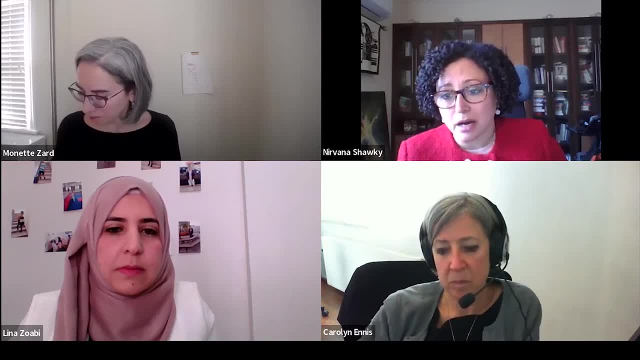 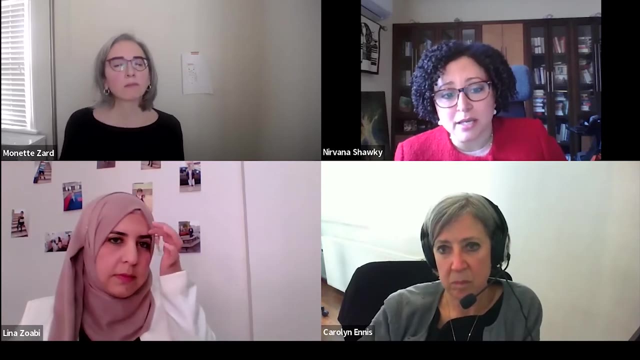 and more than 65% of the population are- I mean currently- in need of humanitarian assistance. Allow me to start- I mean thank you- By a quote from a Syrian woman who lives in Northeast Syria after being displaced. who she says, and I quote: Life is mentally and physically exhausting. We can no longer go to hospitals because health care and medicines are so expensive. My children eat less. They no longer have milk because I had to sell my cows and we no longer eat vegetables because they are expensive. 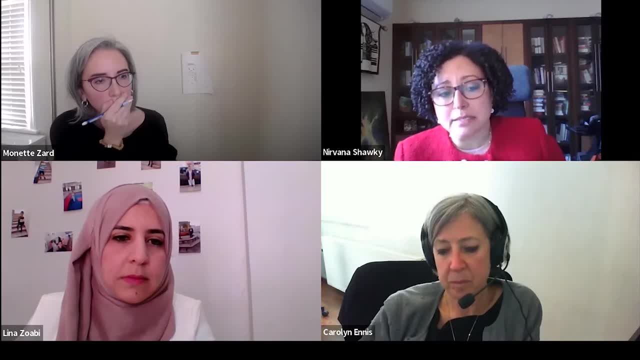 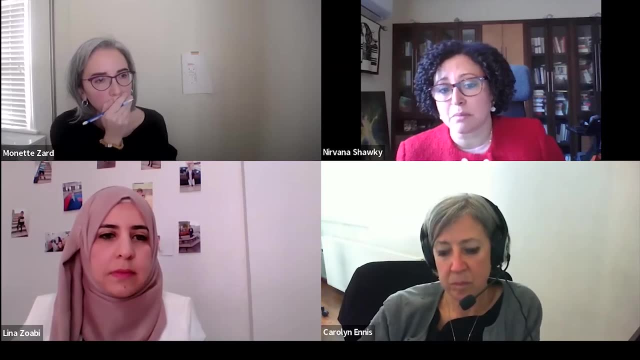 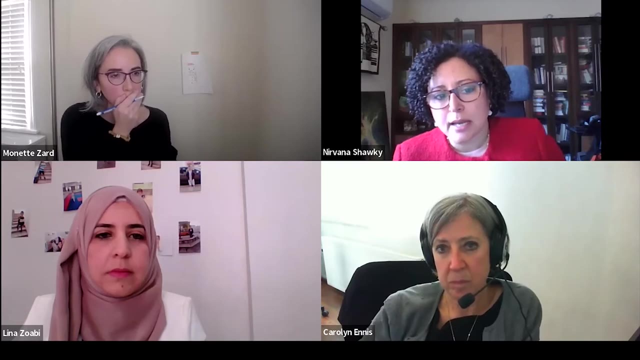 End of quote. We, as CARE, have interviewed this woman as part of the rapid gender assessment analysis that I mean CARE is very known for, and we had to do one before the Ukrainian crisis, and it was actually collated in a report. 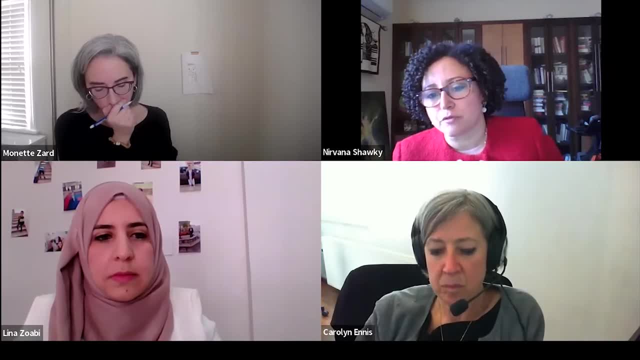 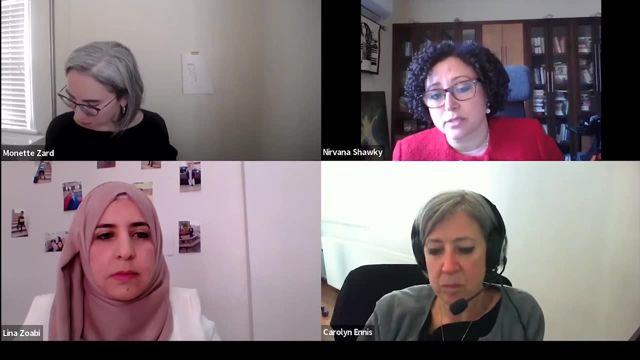 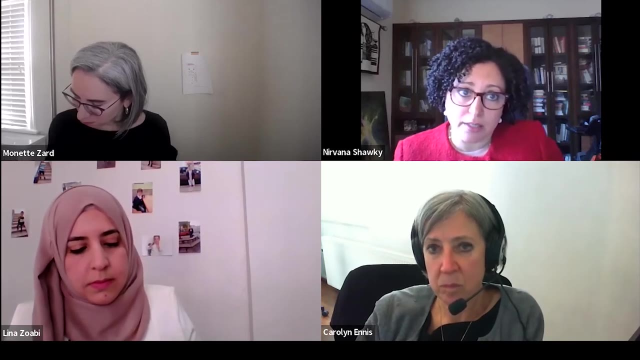 And this report shows how families have had to reduce their food consumptions and one in five children faces malnutrition in Northeast Syria, And I'm sure if we meet this woman again, she will tell us we can no longer eat bread today because of the Ukrainian crisis. 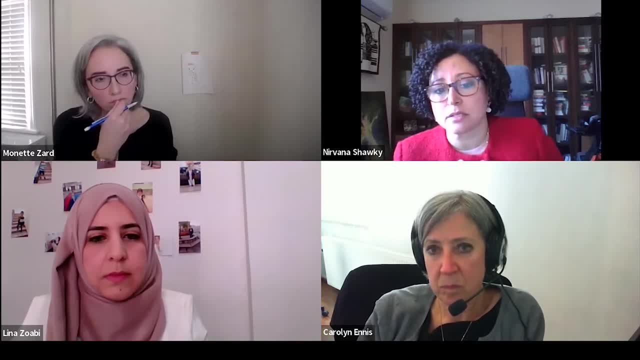 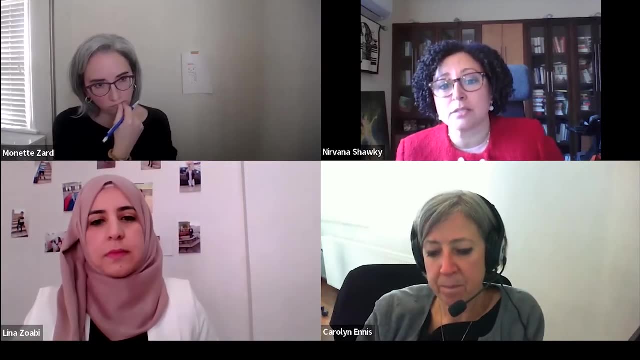 CARE has been working in the Middle East and North Africa since 1948.. And actually, when we say MENA for CARE, it also includes Eastern Europe. So we are working the Caucasus and the Balkans, and now working also, I mean, on the Ukrainian crisis. 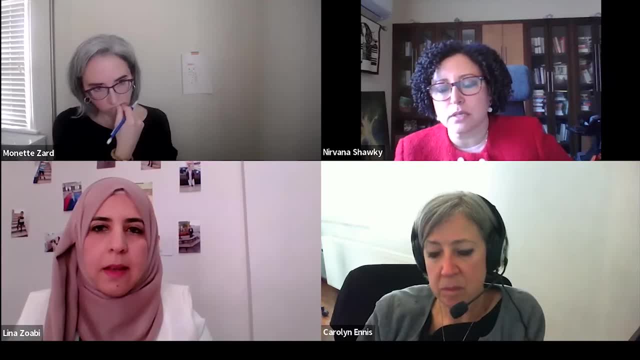 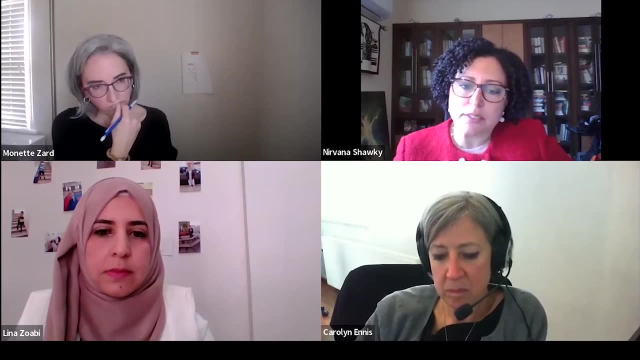 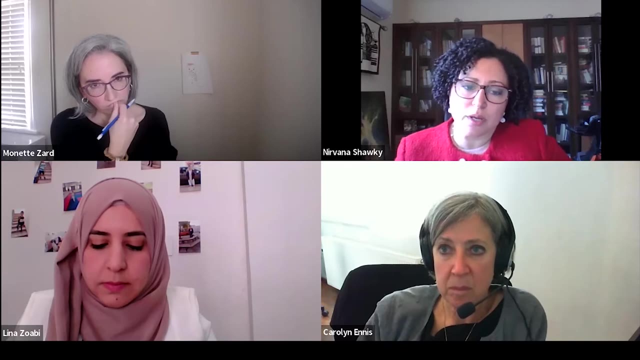 And the region is home to the world's most and worst humanitarian and refugee crisis in the world. Our program delivers emergency aid as well as longer-term support, working through partners and with direct action as well, And we focus on strengthening people's resilience. 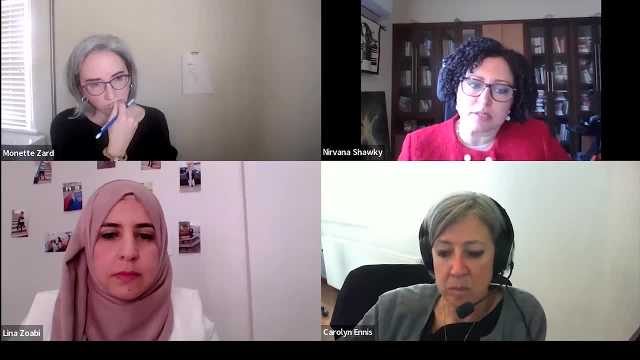 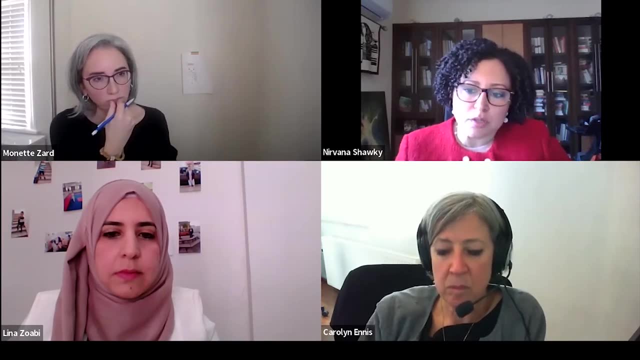 supporting them to absorb and adapt to recurring shocks and stresses, And our expertise lies in gender responsive emergency response, food security and livelihoods, water, sanitation and hygiene, support, women's economic empowerment, as well as protection of vulnerable groups, with a specific focus on women and girls. 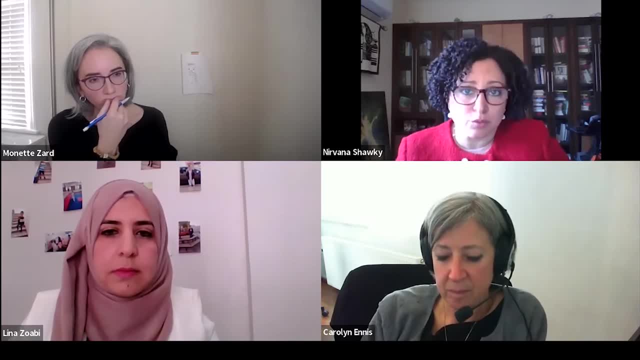 across our programs in Jordan, in Lebanon, in Turkey and also inside Syria, And I mean to answer you, Monette around the strategies we have used. CARE delivers emergency assistance as well as longer-term support, And we believe that emergency and humanitarian aid should be complemented with development work and objectives. 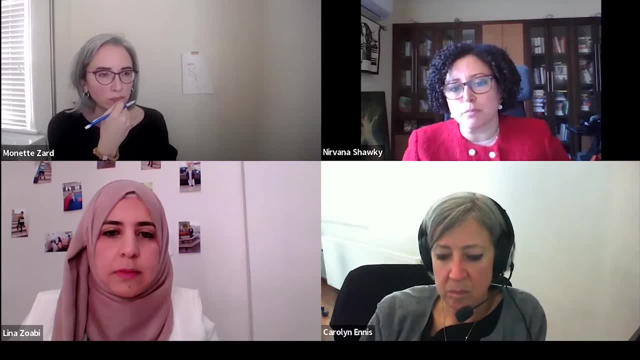 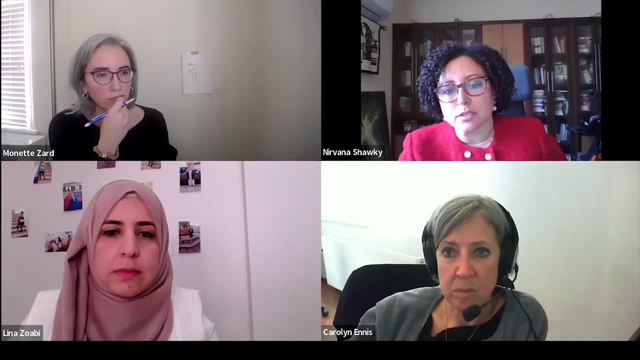 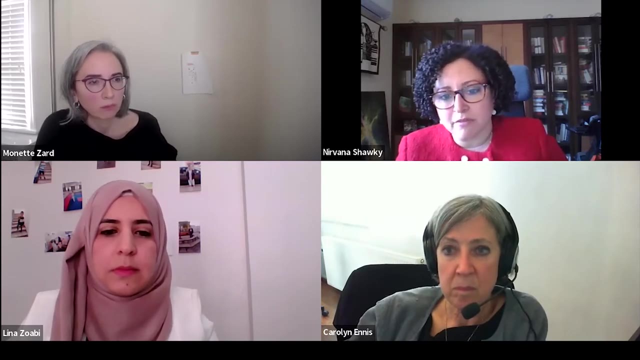 And so using a resilience building approach embedded in value chain programming that is integrated across sectors and provided alongside emergency assistance, is fundamental to CARE's success. We help Syrian women and vulnerable families to become economically empowered and self-reliant, And we prioritize the most vulnerable households based on size and assets and income, and 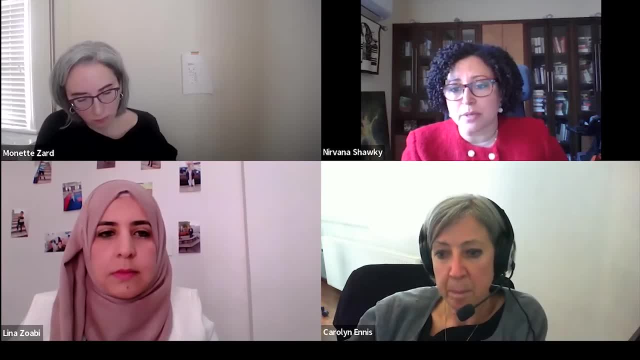 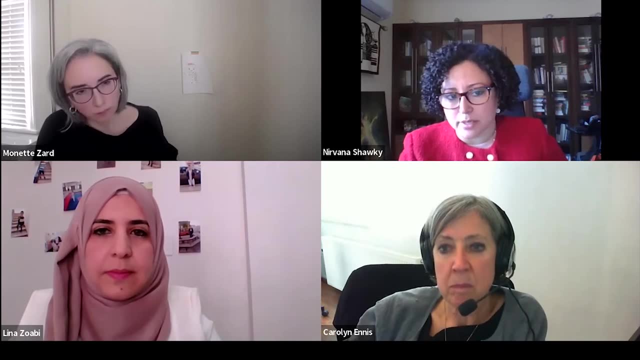 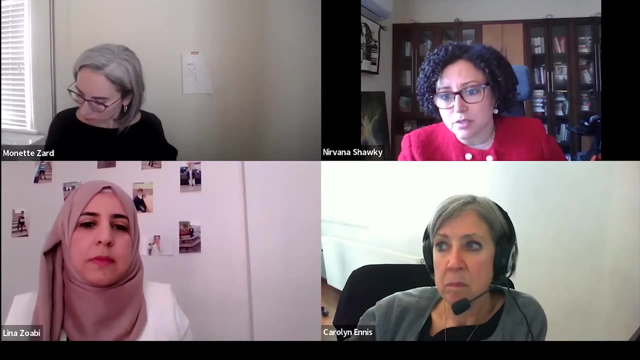 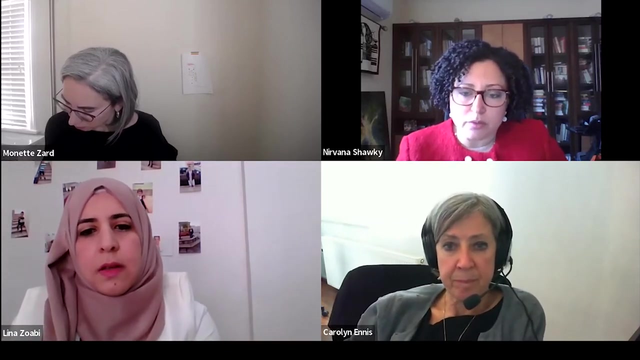 and and gender and their risk to gender-based violence, disability and age, And we build community accountability around that. And CARE support includes training, job placement, such as apprenticeships, awareness campaigns, promoting fair business practices and prioritizing- and I'm so sorry. 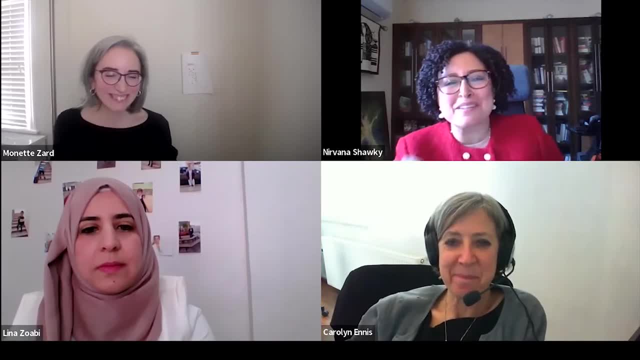 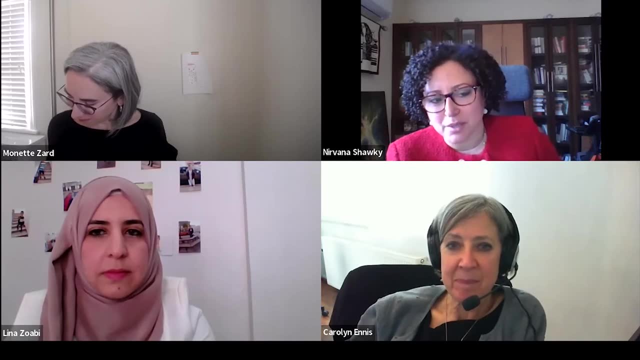 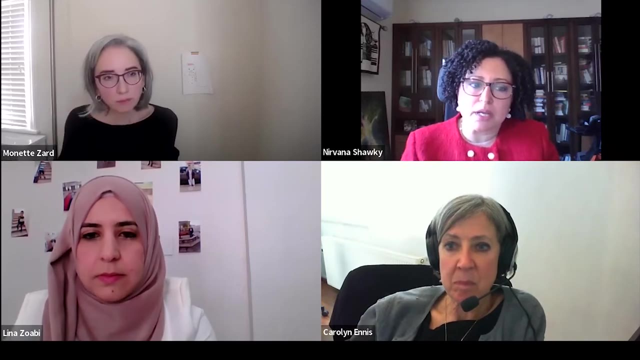 I mean sometimes the English words get very difficult to pronounce- it's prioritizing value chains that enhance linkages between producers and buyers, And sectors we target are actually four key sectors, because I mean there are four gender and livelihood trends and relevant sectors that we are focusing. 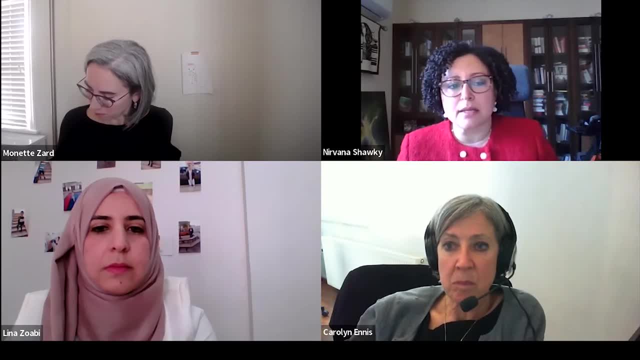 on across the region. We start with the gendered impact- And the crisis in Syria, of course, continues to have a gendered impact with women and SNL adolescent girls. We have to start with this sector to address employment support early. 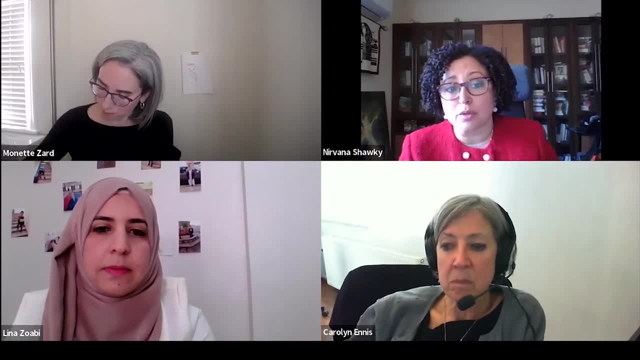 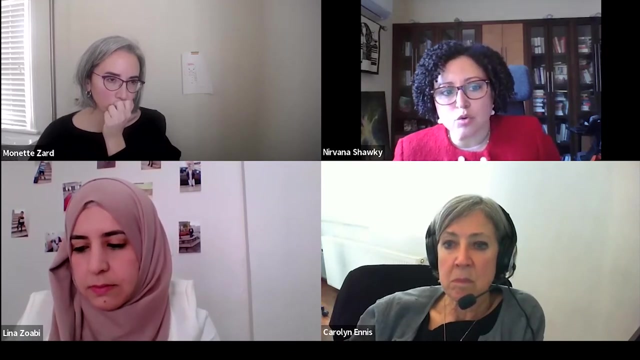 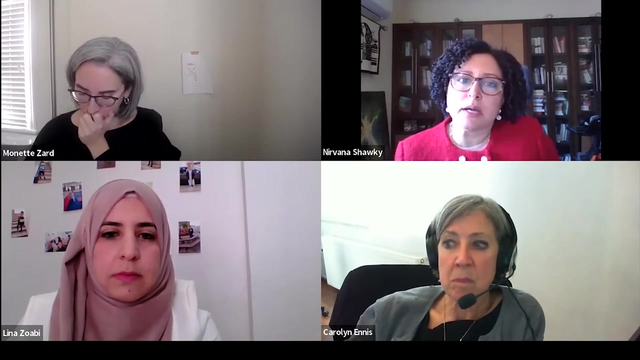 girls paying a high price due to the harmful and discriminatory gender norms and prevailing and widespread gender-based violence, including early and forced marriages. And the economic and psychological stresses are driving an increase in domestic violence, as most of the data tells us. There is also a focus on nutritional deficiencies, where 60% of people in northern Syria report. 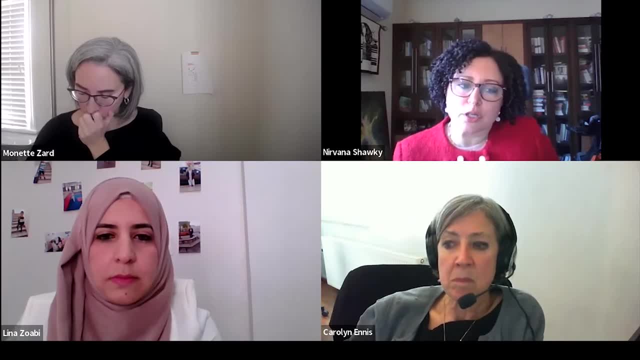 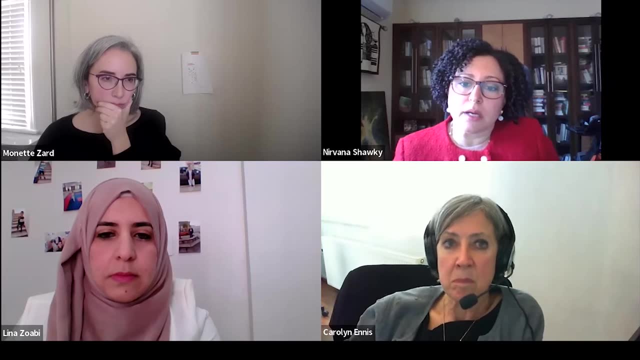 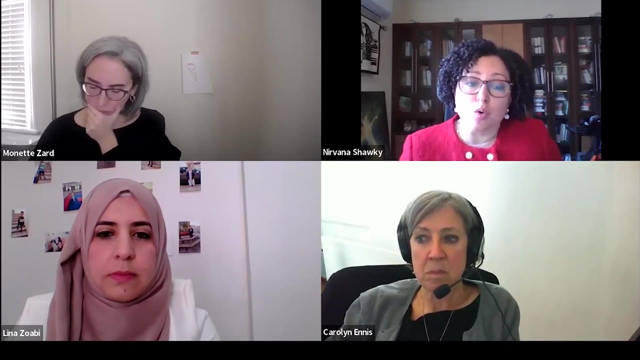 reducing their food intake to ensure their children are fed, and people compromise the quality of food and are unable to buy vegetables or even basic oils. The third focus is the changing role of Syrian women as breadwinners And, since the beginning of the conflict, many men, of course, have died and disappeared. 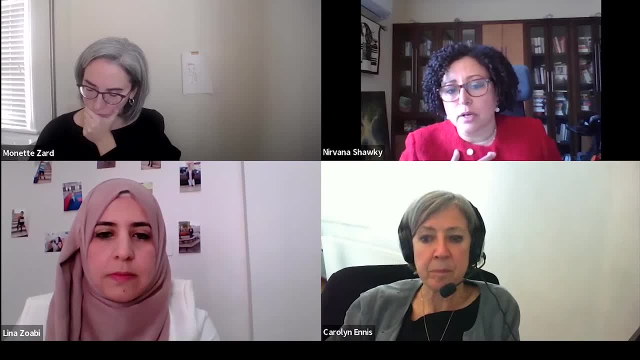 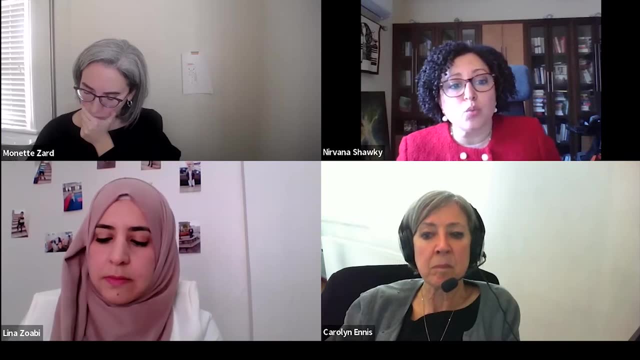 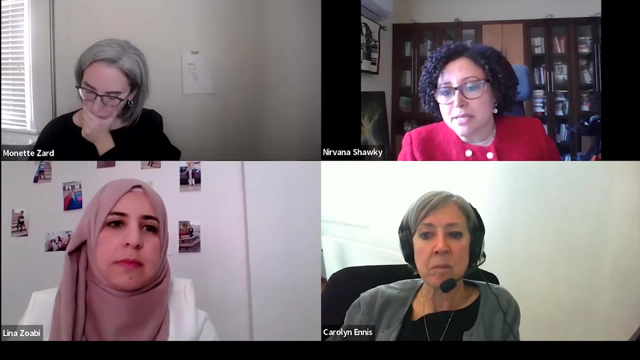 and have been forced to migrate or have been injured during the war, And this has resulted in 22% of the Syrian households are now headed by women. Not only do women bear the burden of household responsibilities, but they also have an additional role to play, that of the providers. 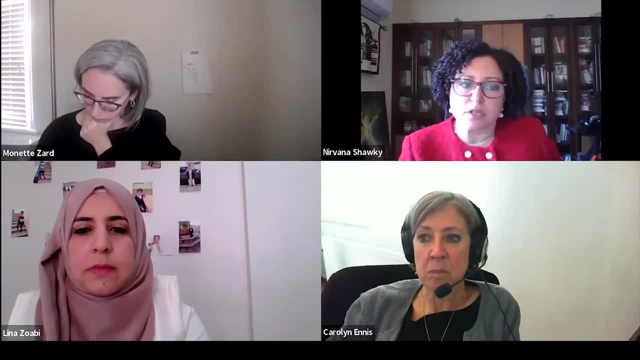 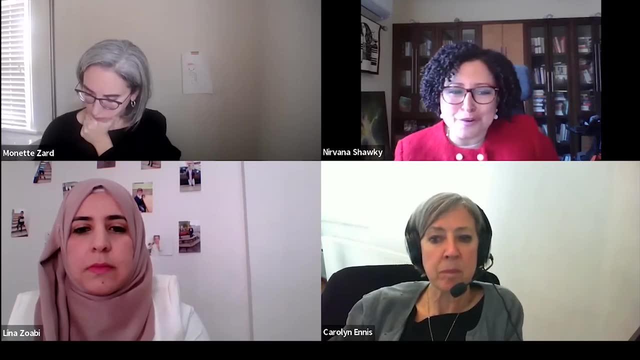 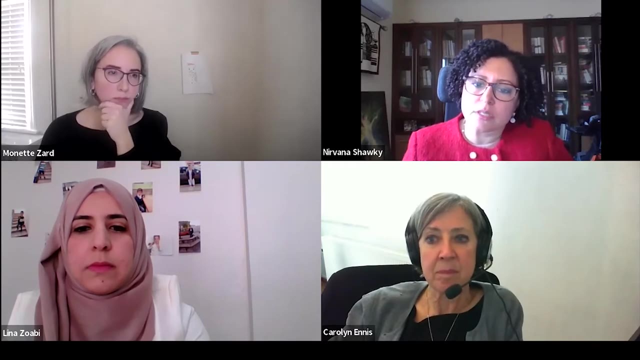 And the final focus is the distress and feeling of insecurity which incurs recent annual needs assessment of conditions in Jordan that you have all already, I mean, have received copies from it. It demonstrates the severe distress among thousands of refugees and vulnerable Jordanian. 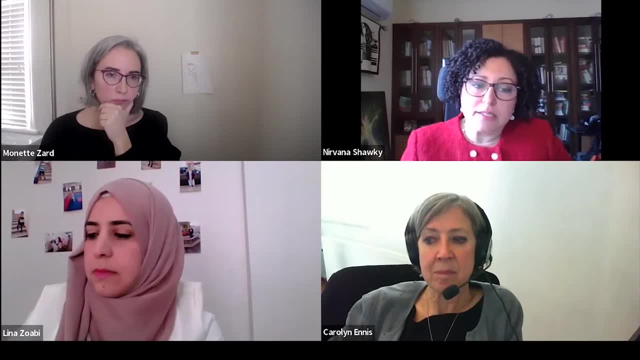 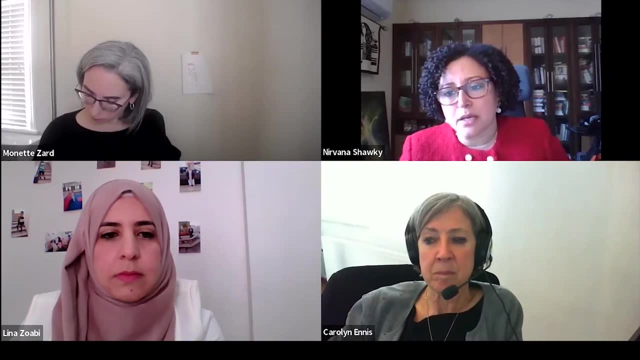 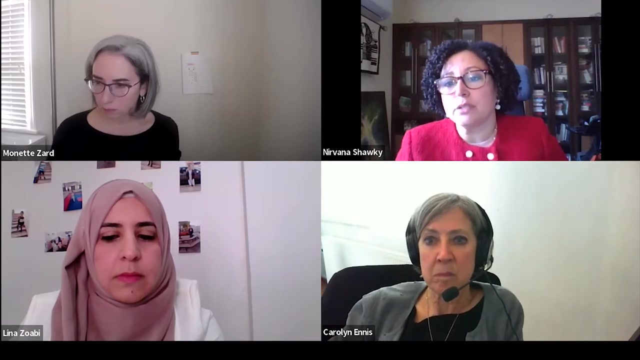 families interviewed across the country. As we've seen over the last two years, particularly the economic stress and the impact of the pandemic are driving an increase in violence against women and children. Even with more women taking up the role of providing for their families, few women have any control over how their earnings are spent. 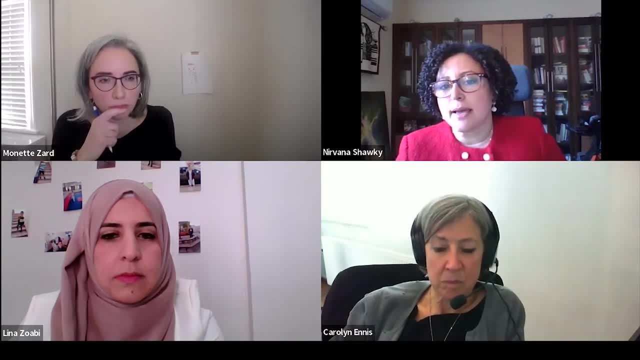 And compared to last year, the number of respondents facing verbal and emotional violence at home has risen by more than 30%, with reports of gender based violence having also increased And, compared to last year, the number of respondents facing verbal and emotional violence having also increased. 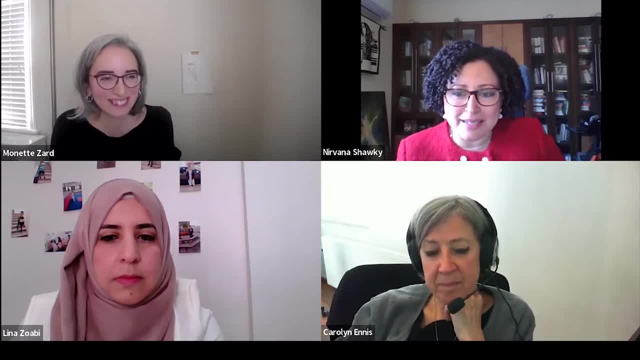 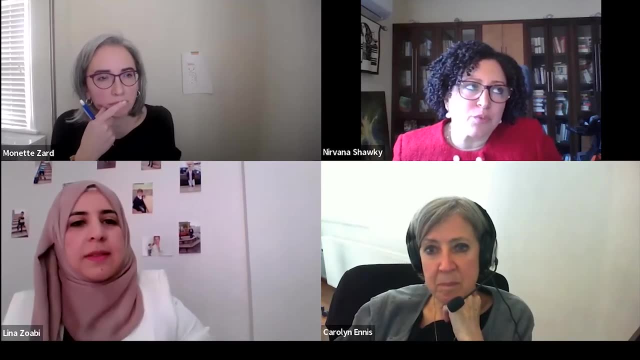 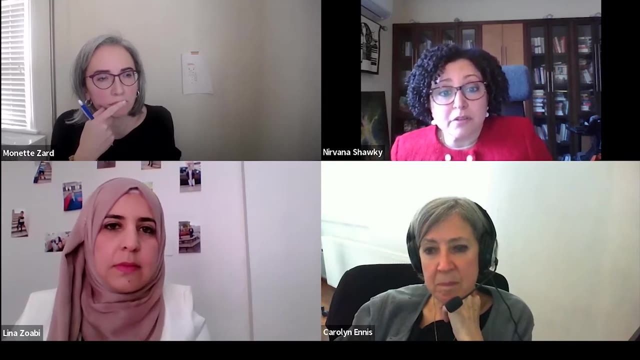 To answer the last part of your question about what does success look like for us and what are the some emblematic projects that we are, I mean, focusing on? CARE is currently actually piloting innovative approaches that support more inclusive communities and marketplaces. 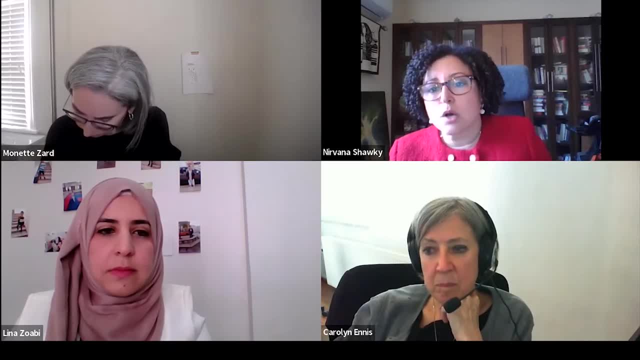 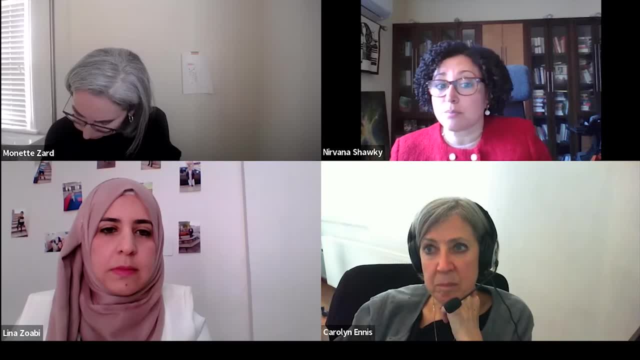 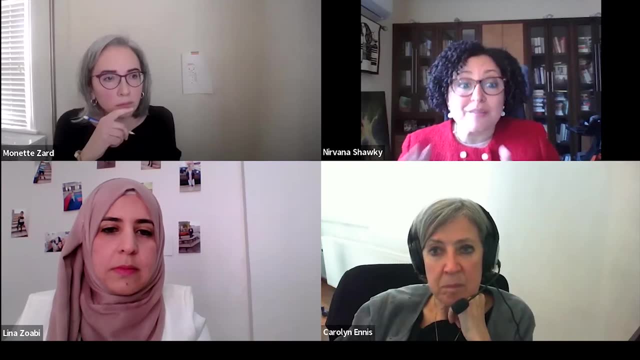 And we are testing new approaches to inclusive livelihoods, with a particular focus on women and persons. And we are testing new approaches to inclusive livelihoods, with a particular focus on women and persons. Our projects support people to restart their livelihoods and protect existing productive assets, which are vital in increasing the capacity to absorb new shocks. 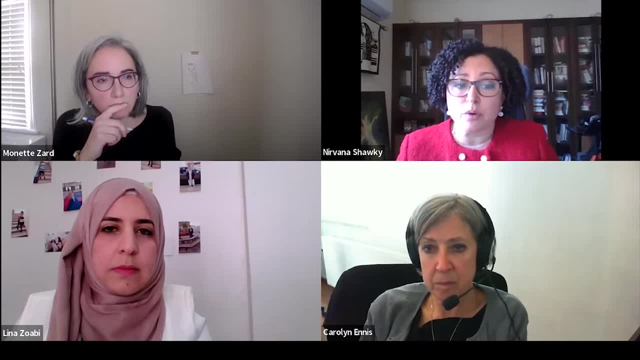 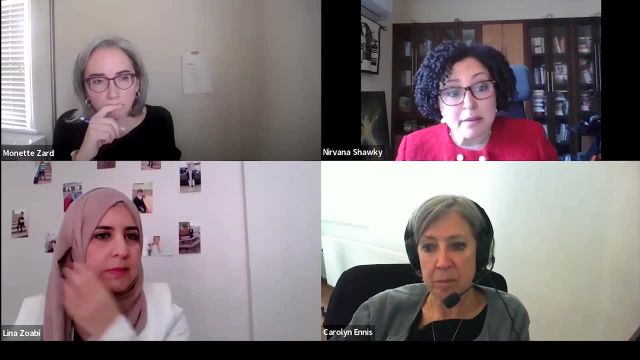 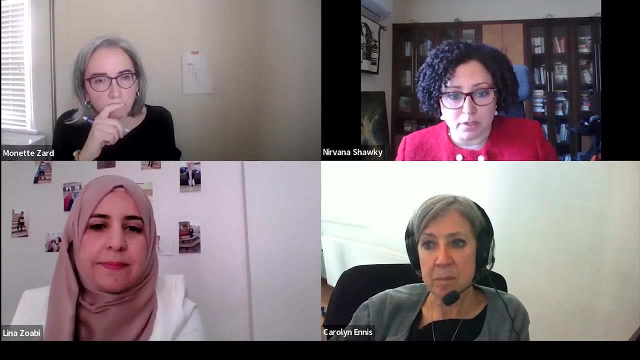 And CARE provides vulnerable men and women and persons with disabilities, and marginalised groups as well, with access to livelihoods, inputs such as fodder and certified seeds and fertilisers, sterilizers and vaccinations, and even tools, And we try and care to build skills in agricultural. 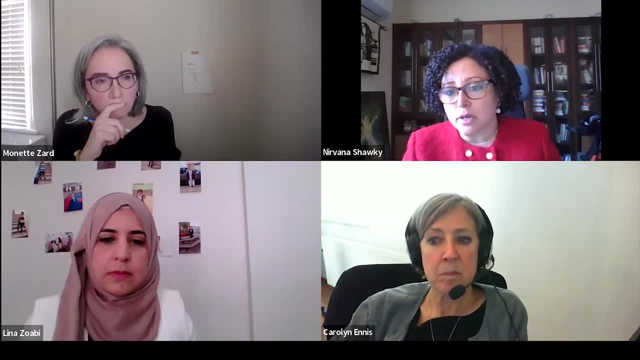 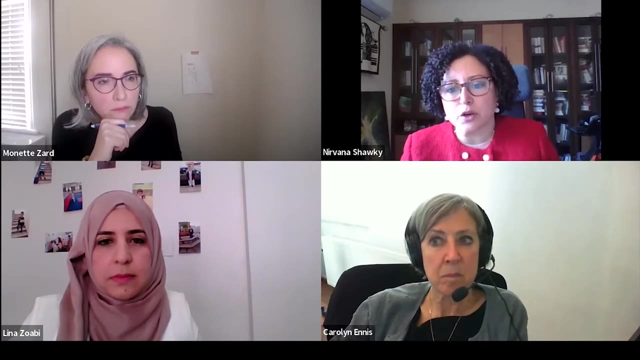 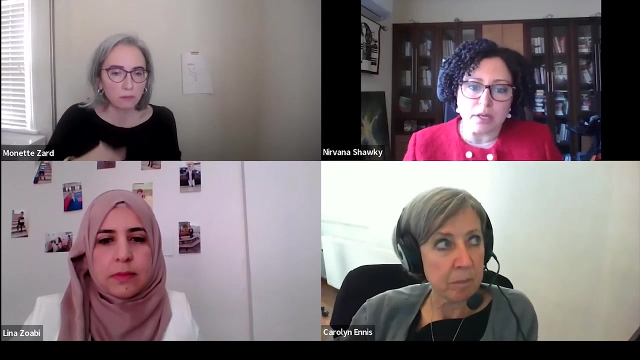 production, particularly including using the farmer field school approach to train farmers or herders in techniques to improve the quality and quantity of the food they produce using less resources- And this is critical given the recurring issue of water shortages and drought in Syria- And this training support covers both plant-based and lively stock. 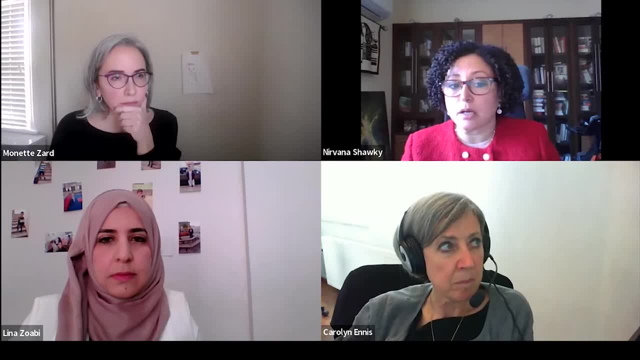 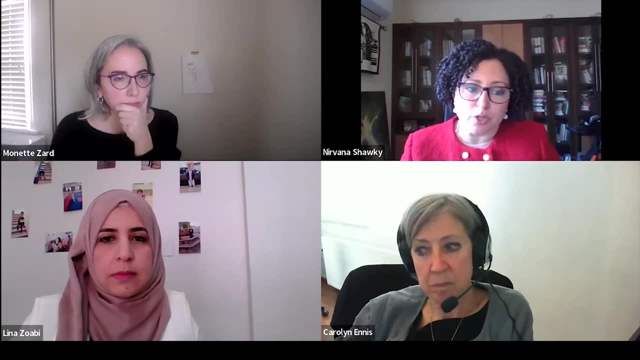 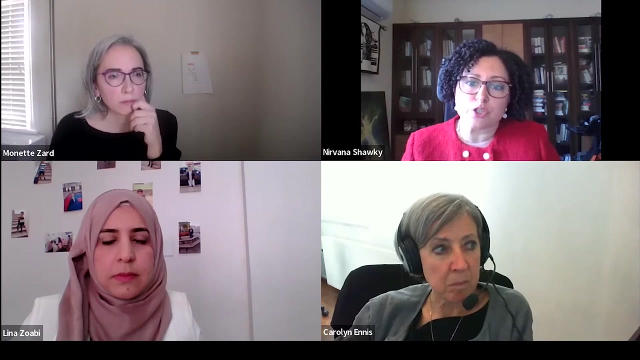 agricultural value chains, including climate-smart agriculture and venetary skills and fodder production and biogas production. And furthermore, we actually focus also on cash for work opportunities, which both provide vulnerable people with temporary income and help restore essential infrastructure upon which the entire community relies And the entrepreneurs receive. 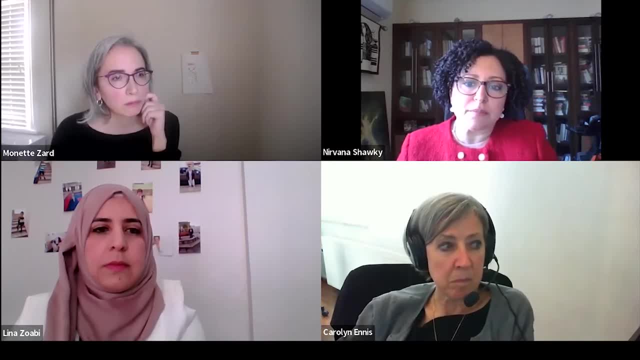 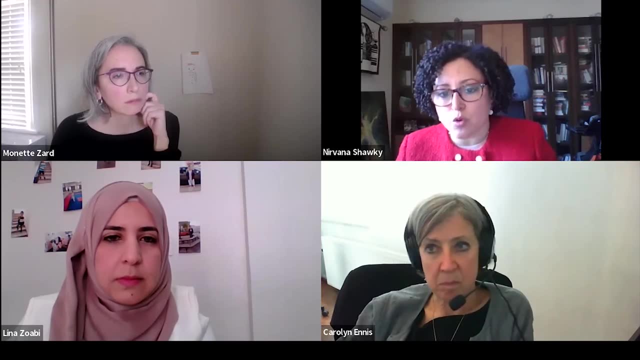 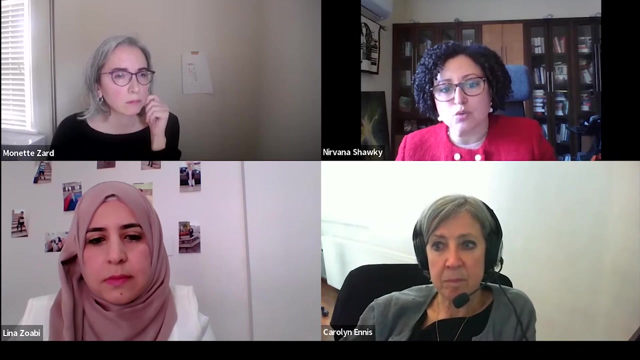 grants or inputs to start or expand small and medium scale businesses. And finally, many of our projects across the region also focus on the gendered impact of the shifting social norms by increasing engagement of men and boys in psychological support and gender-based violence prevention and response, and these strategies to increase women's voice in the public sphere. 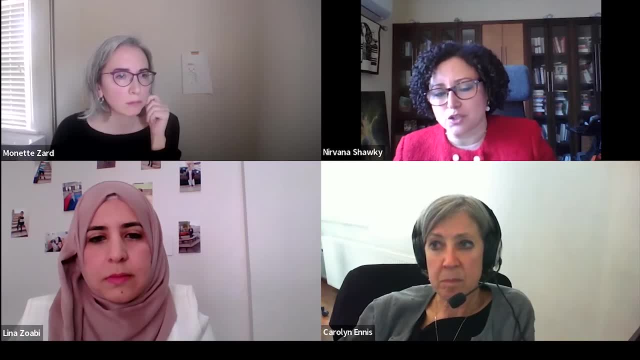 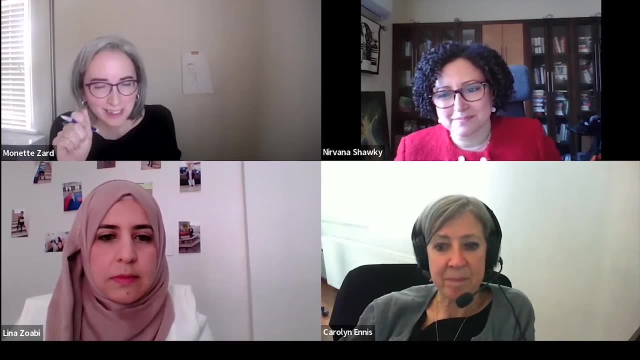 in the household as well as in community decision-making. Very interesting. Thank you, Nirvana. In fact, your last point takes me into the direction I wanted to go in my next question, But perhaps briefly if you don't mind. 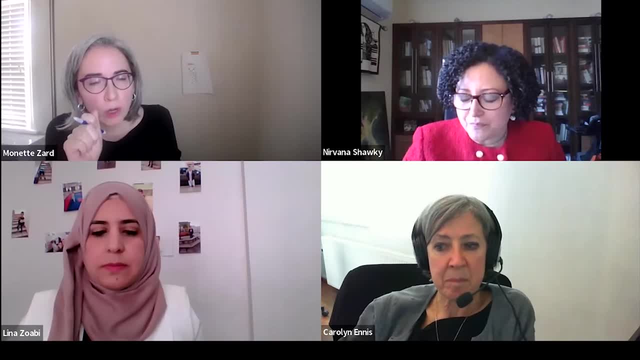 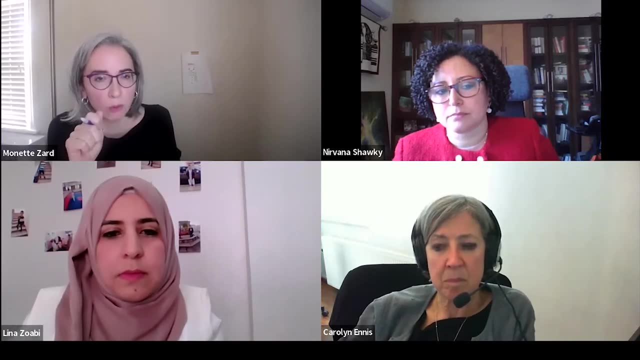 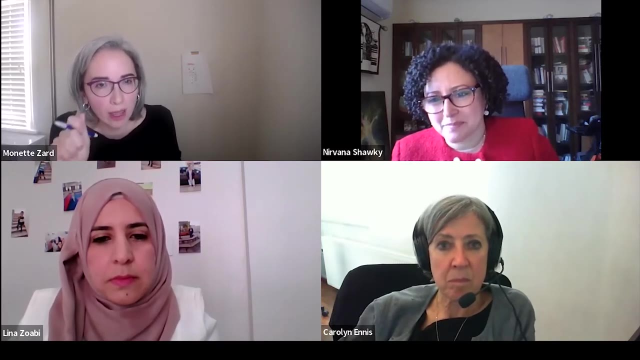 can you talk a little bit about what you're doing to address some of the barriers to more active engaging women in the workplace? You talk there about one strategy which is engaging men as a way of sort of impacting gender norms and perceptions. Perhaps you could talk about one. 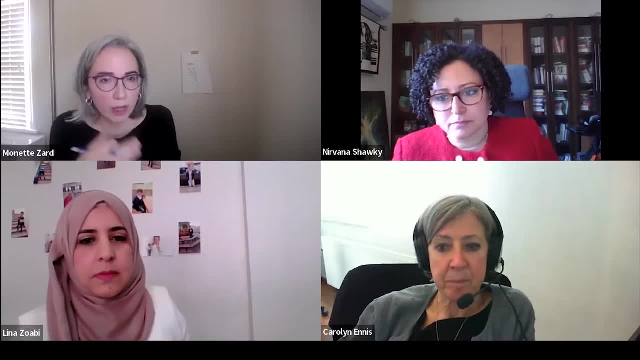 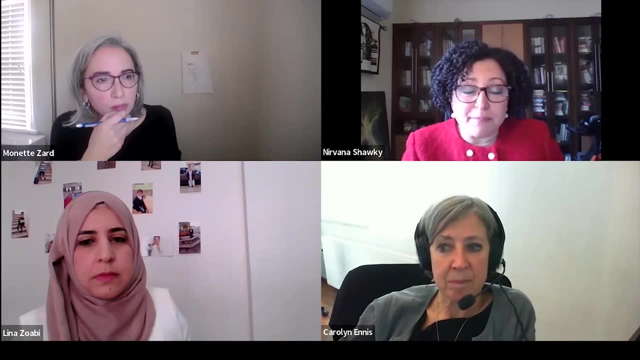 or two other barriers, and how you're approaching them through your engagement or your advocacy. Sure, Thank you. Thank you, Monette. Actually, I mean, our approach to include men and boys has started since the Balkan wars And this has been really, I mean. 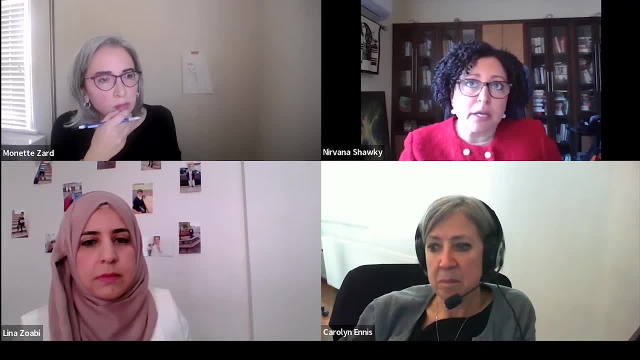 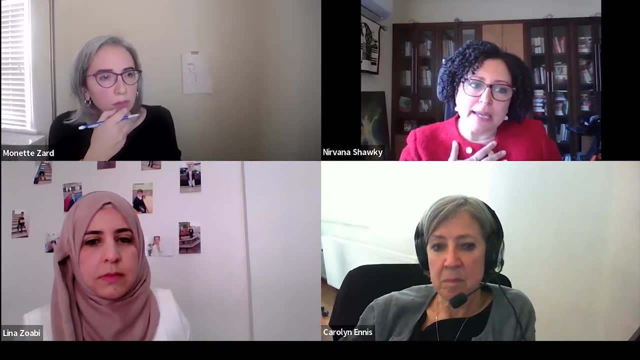 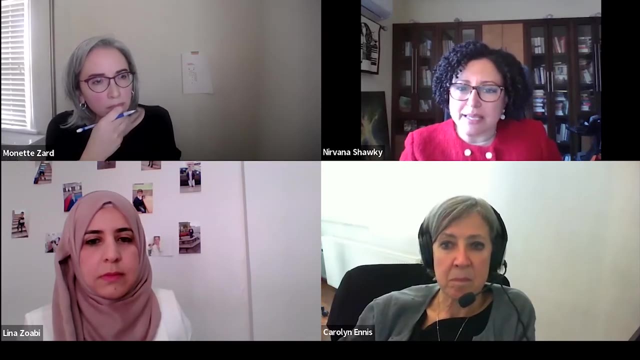 a big shift in gender programming globally to focus really not just on one side in the community but actually to have a balanced approach of the engagement. And I mean to focus on your question. sustainable and longer-term funding is a major constraint on our programming, as you can imagine. 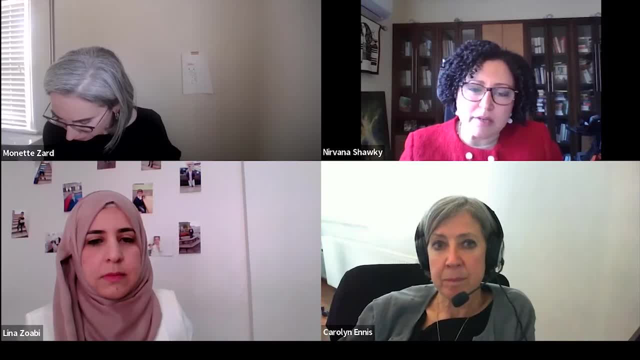 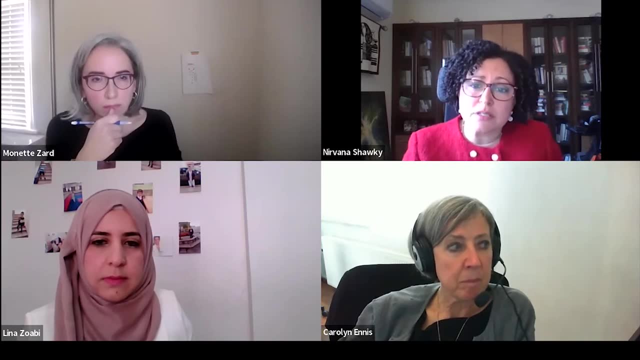 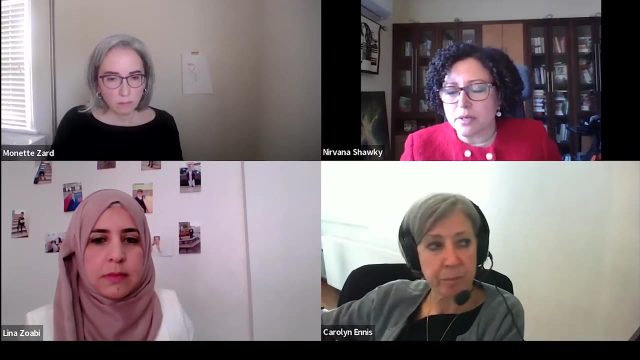 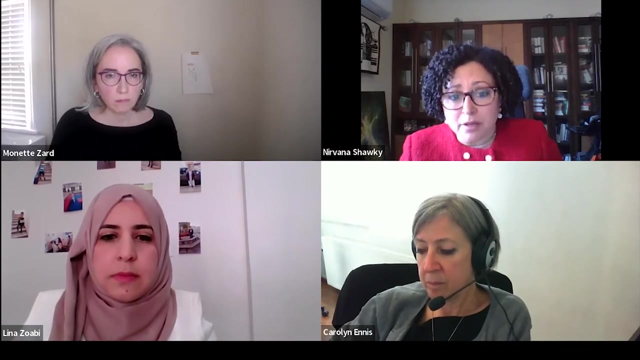 We therefore need increased humanitarian funding for the Syria crisis across the MENA region that co-currently support life-saving interventions and early recovery and resilience programming, And I think that that focus- I mean looking at the humanitarian regional response- sufficiently the funding of the forthcoming two-year for the HRP, with a balanced approach. 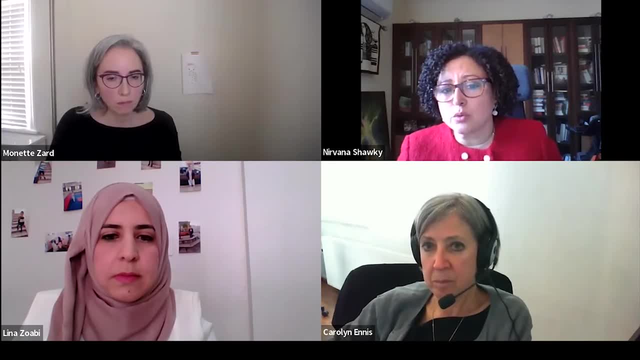 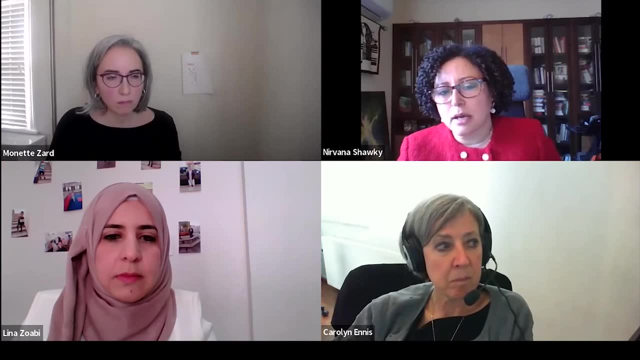 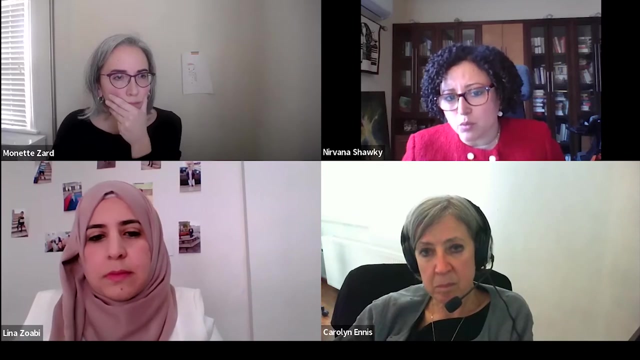 to funding activities across the three pillars, including redoubling efforts to increase the life-saving programs. to increase funding for multipurpose cash assistance will enable individuals and households to prioritize the needs they would like to address. The other big constraint or burden is actually, in Syria, about 70 percent of people working on farms. 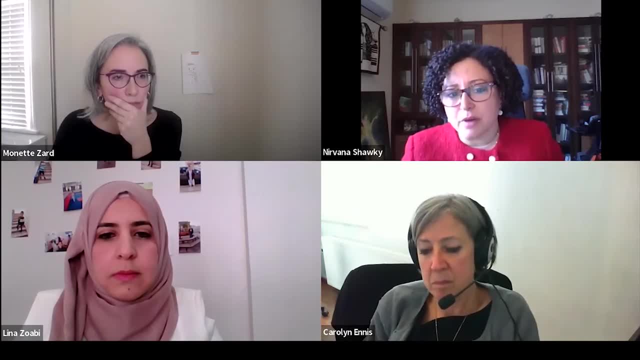 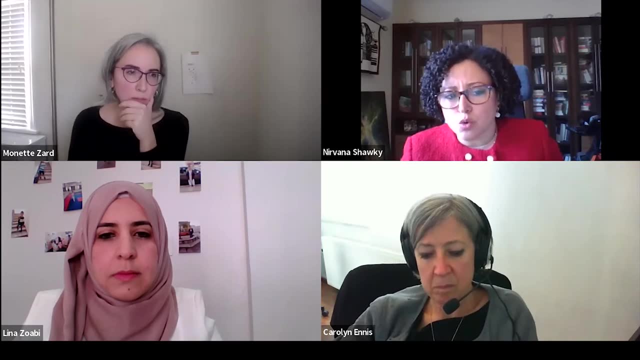 are women and many of them are the main breadwinners in their families, as men I mentioned are injured or deceased or missing. And without water there are no corpse, and without corpse- I mean without corpse crops- sorry- there is no income and there is a. 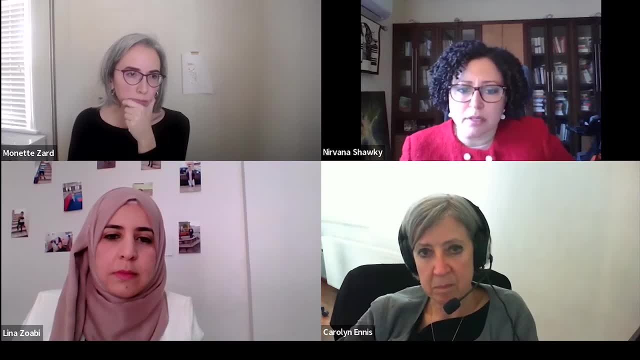 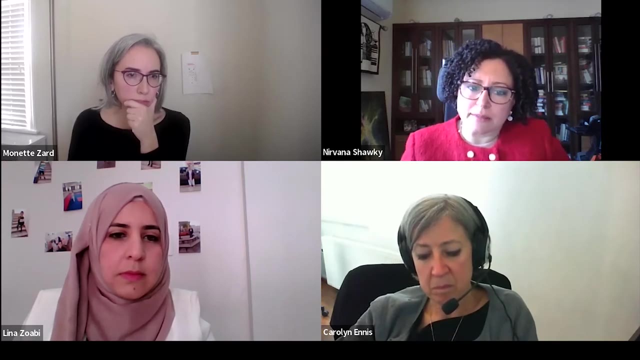 decreased availability of food, which means that a lot of women and their children are spiraling deeper into both hunger and poverty. and- and there is I mean there is no time to waste, because the situation demands that authorities in the region and the government would act now to save these. 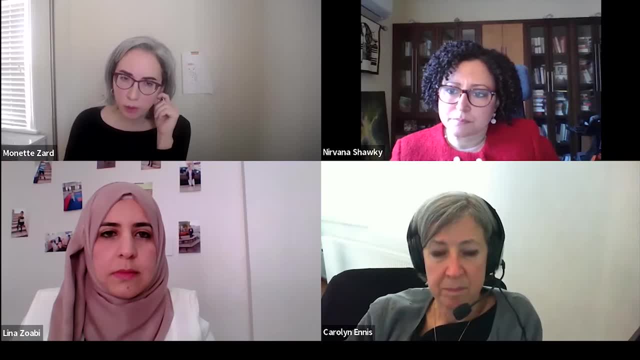 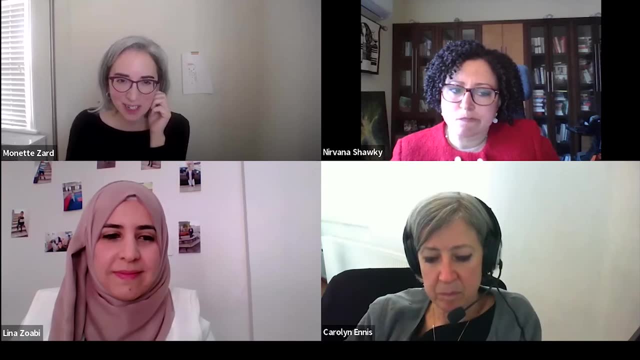 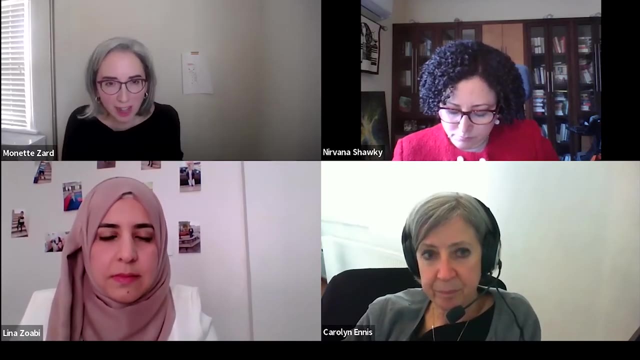 lives, Thank you. Thank you, Nirvana. We will definitely circle back to some of these themes, but I'd like to move on to Lina now. Lina, welcome, I'd like to turn to you. I mean, you know, as a Syrian woman yourself and someone who's worked, I know, extensively in Jordan, in 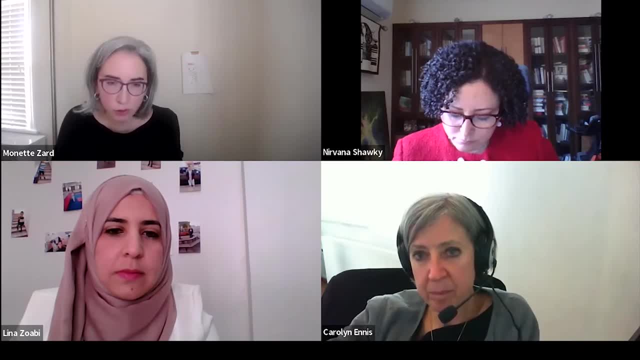 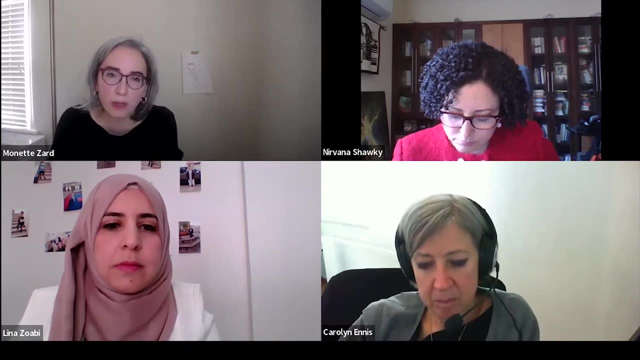 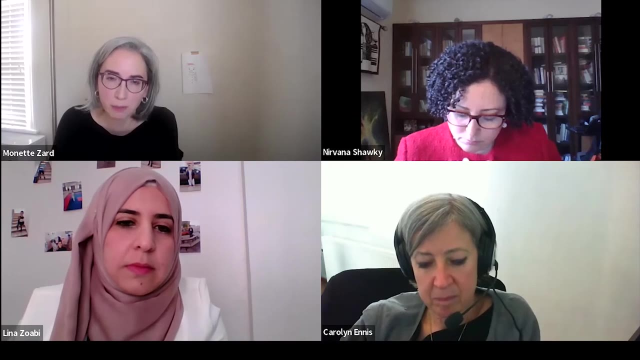 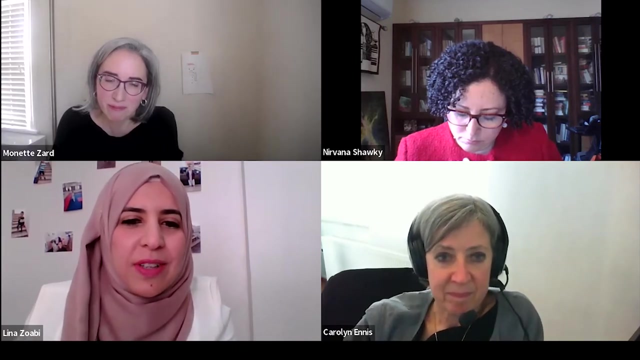 particular with refugee populations. could you share some reflections on how you feel from what you've heard, what how Syrian women themselves reflect on the livelihoods issue and what some of their aspirations might be in this space? Okay, thank you, Manas, for the invitation being one of the penalties. Thanks for also the introduction. Basically, last year it was a heavy. 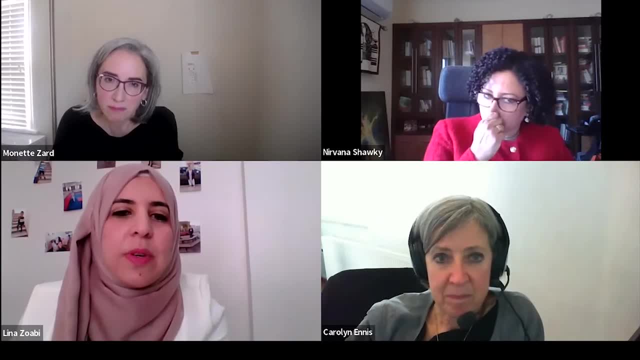 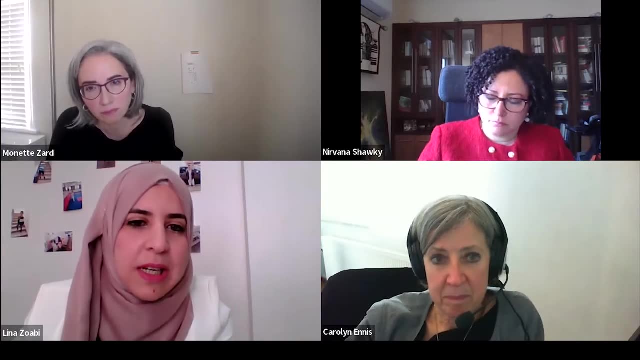 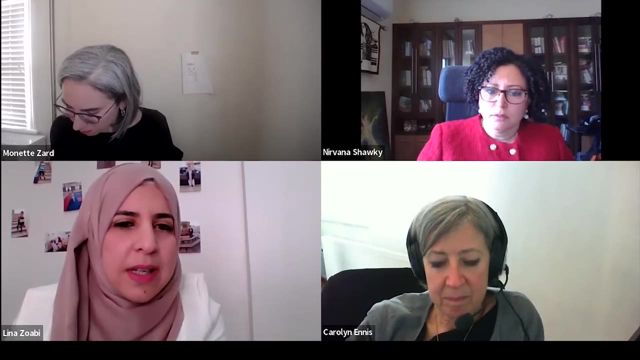 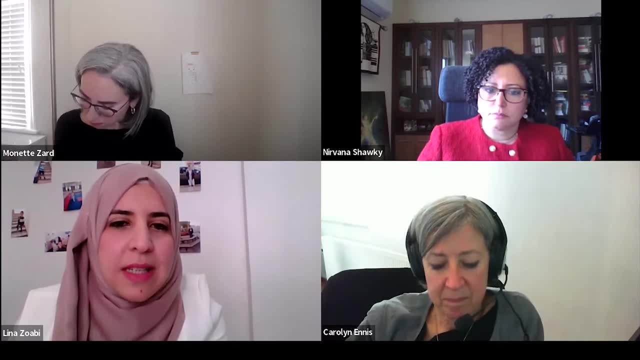 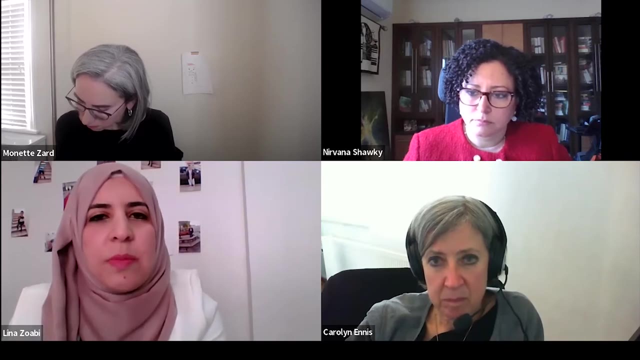 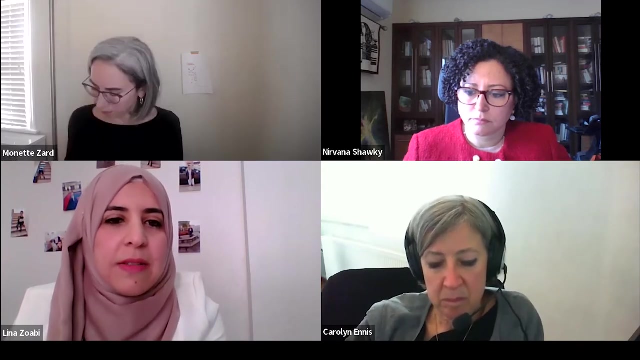 said like in a report. like like death for Syrians. 90 percent of Syrian refugees who live in the extreme poverty for they rely on debt or borrowing just to survive. So Syrian women in the country of neighboring Syria they live in very difficult financially, Basically the because of the loss. 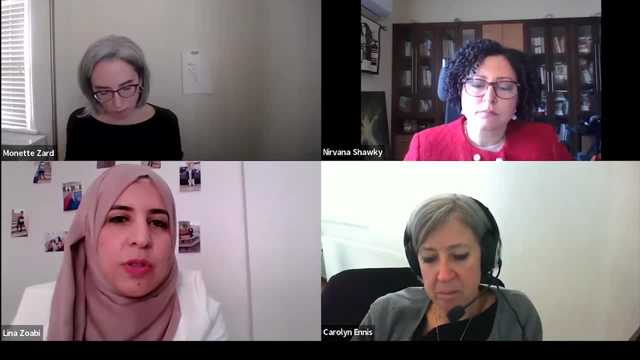 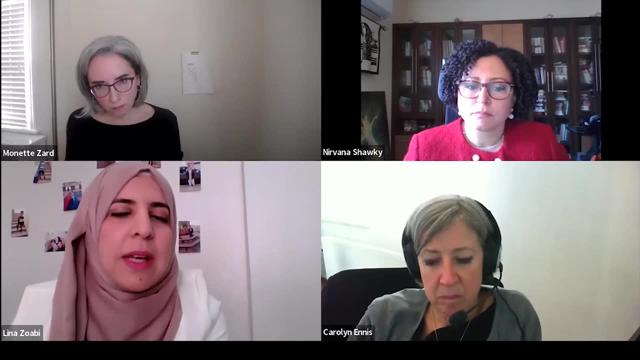 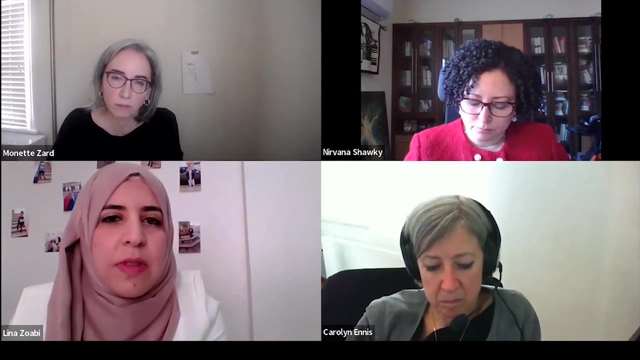 or the absence of the bread winner during the war, which they are basically. according to the tradition, as a Syrian, one of them, the bread winner used to be the male figure in the family, So the the absence or the loss of the breadwinner make it's very difficult for them. Also, the decrease of the job opportunities which 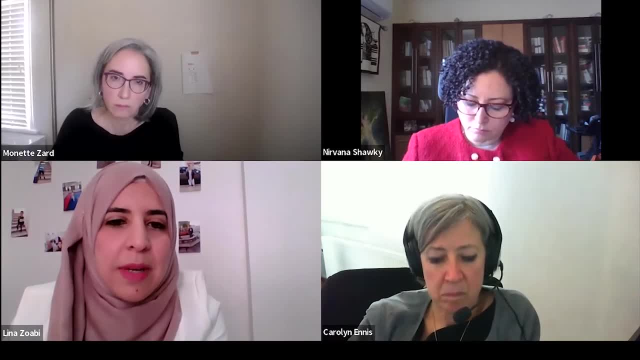 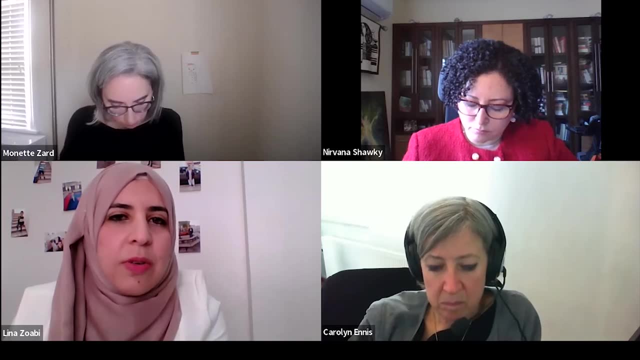 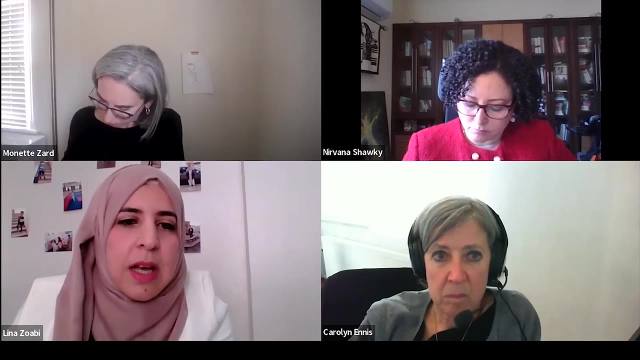 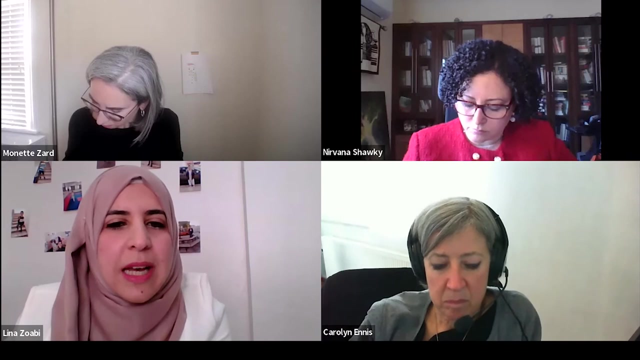 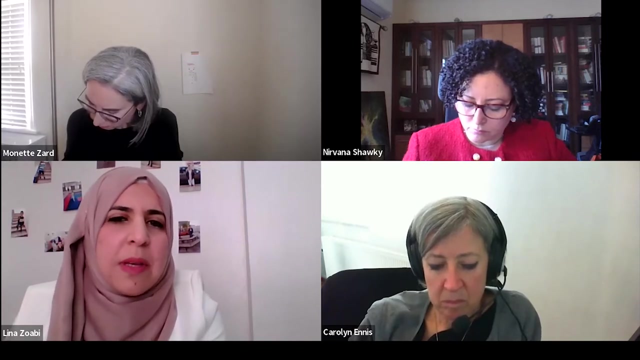 intensified during the corona pandemic. all of that increased for Syrian refugees, and women particularly, who are especially the breadwinner and their families increase the poverty rate. Also, women, as I met them, they view the livelihood aspects for them as one of the difficult situation They believe it will be. 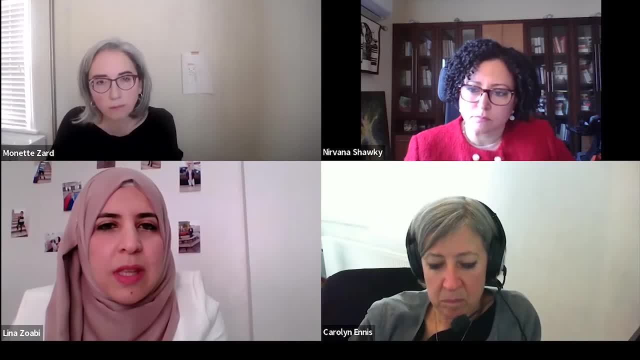 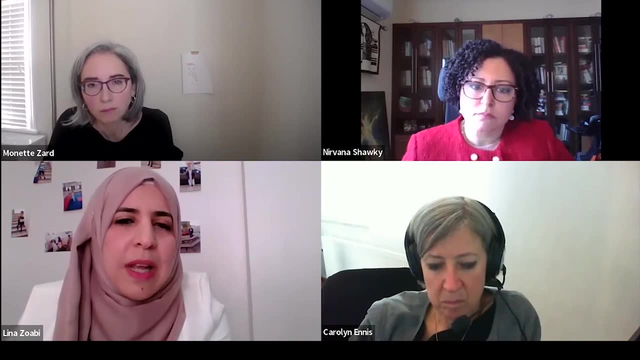 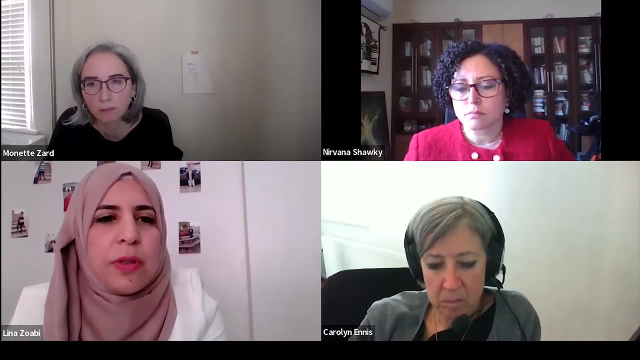 worsened in the future, especially with the decrease of the support that was provided to them by the response plan for Syrian refugees in the host countries They view like bitter livelihoods or the access to formal work to support themselves basically, and their families in turn. 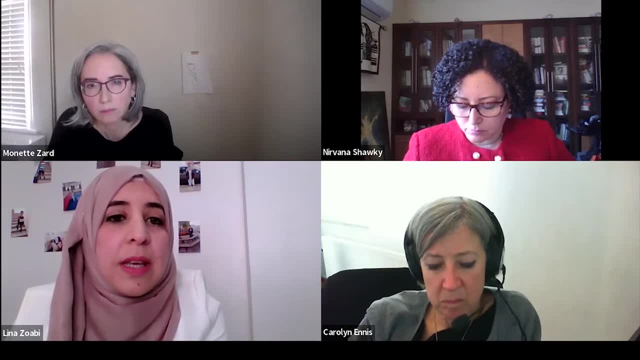 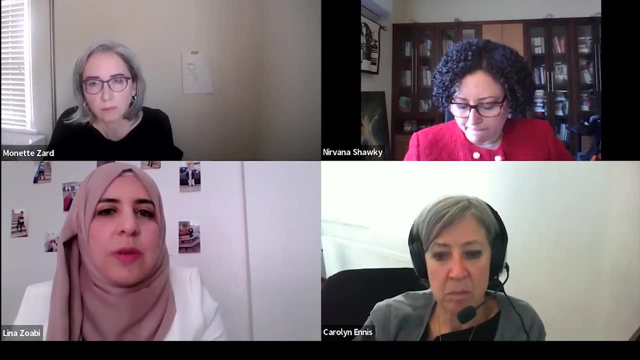 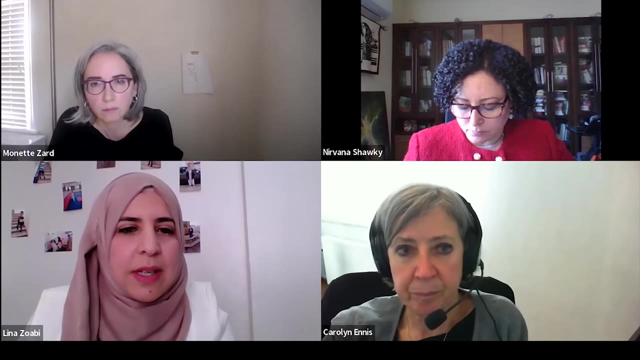 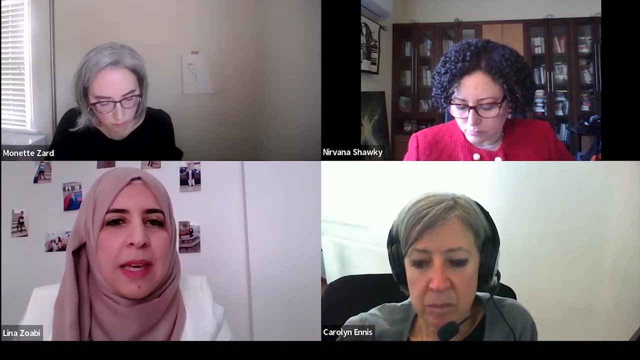 This is was one of the foundation for the empowerment for them and the also the integration, the the equality with people in the host countries. So they try to find ways to support themselves by finding economic opportunities, but in a long term they also have to make or to support sustainable livelihoods for them and their families, and even 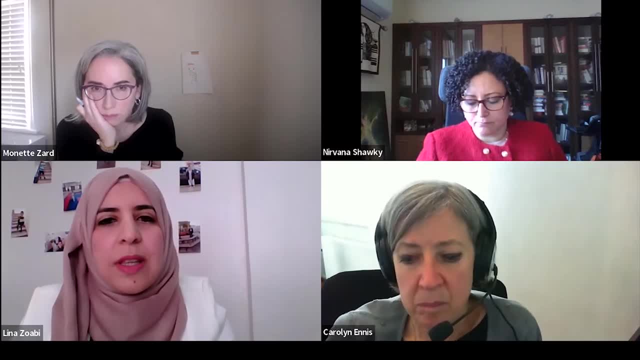 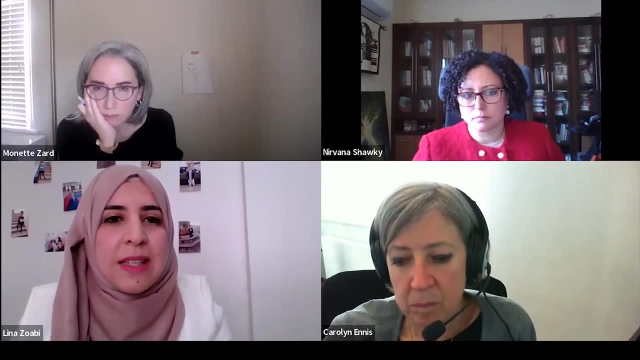 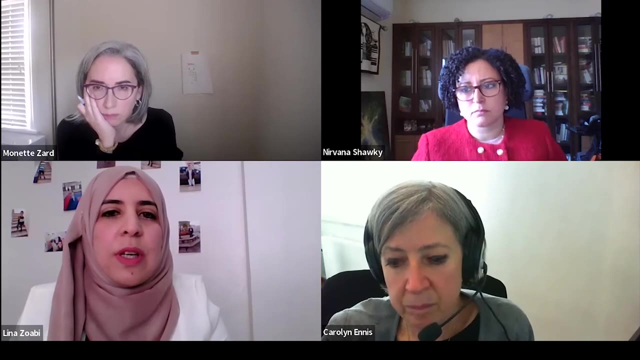 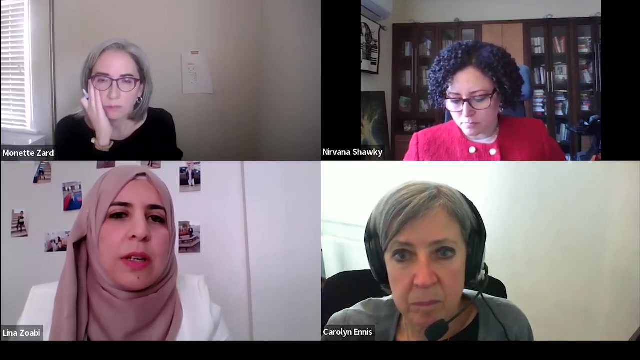 the integration in host countries. So this necessity required women to transgress, as Nirvana said, the traditional norms, gender norms they used to live on, and to go beyond the private domain to seek like for aid services, for example, or informal work in the host country to support their families. 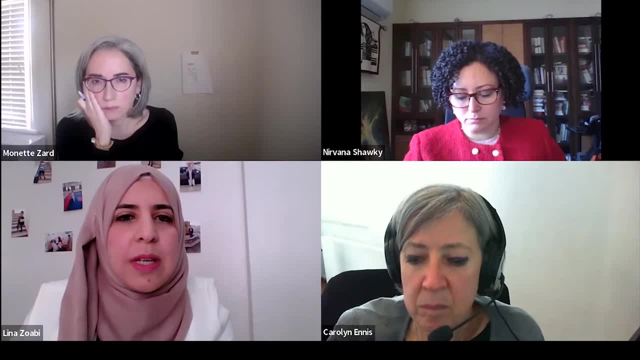 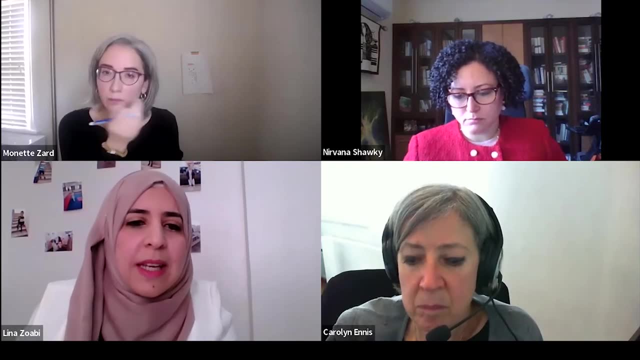 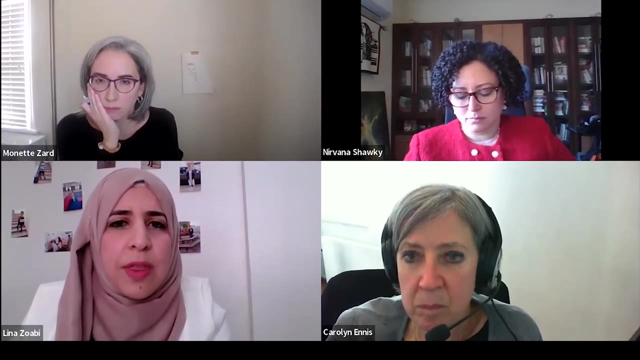 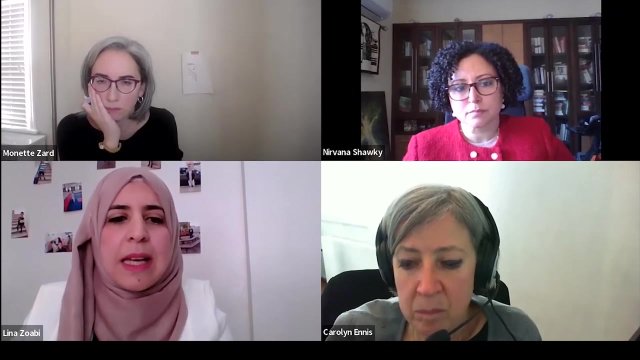 So they desire to work to to sustain a respectful livelihood for them and their families, but the increased responsibilities within their households put them into a higher place of some sort of a position. In the end, they are left with the responsibility of their families, and their families are. 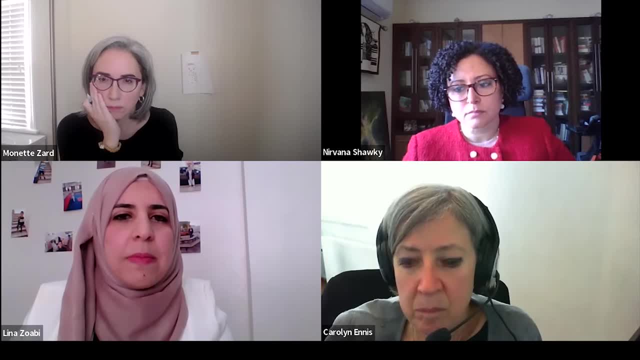 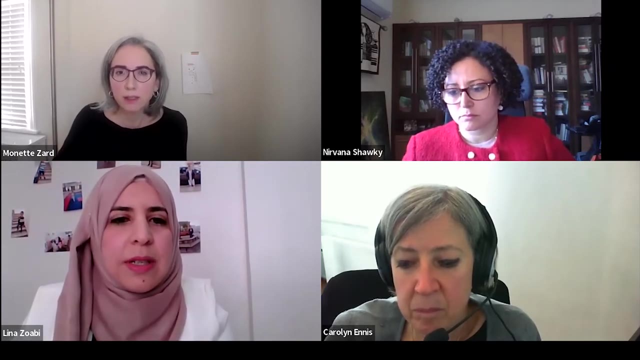 the ones who are the most vulnerable and the most vulnerable of the working class. So the women have to take part in the work and also the women have to play a leading role in their work. This is also a very important issue at the moment that we have with the women in the host countries. 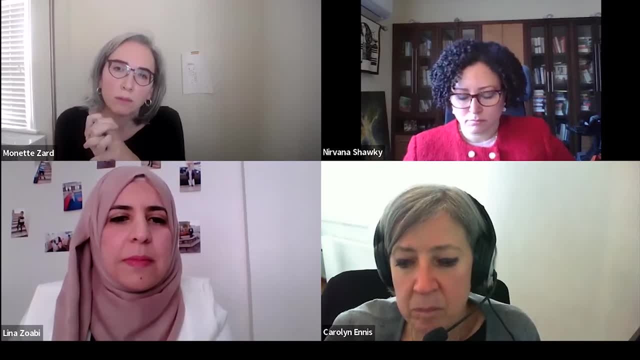 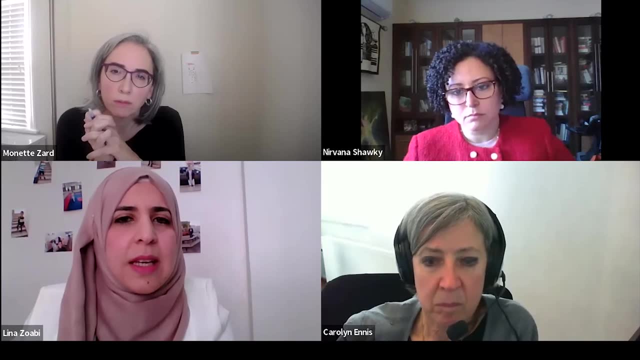 and also with the other countries, in the host countries as well. So we have to have support and we have to be able to support them in their own way And for the refugees they are targeted, the male dominant, let me say it like that: 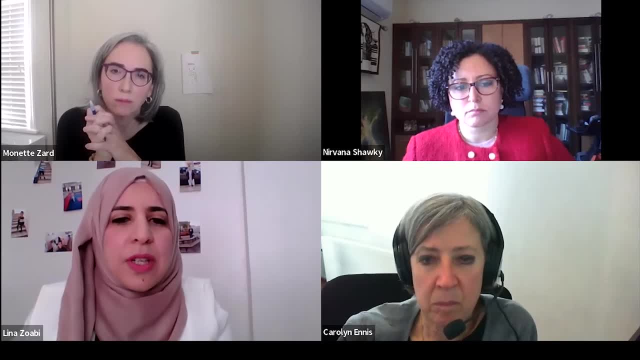 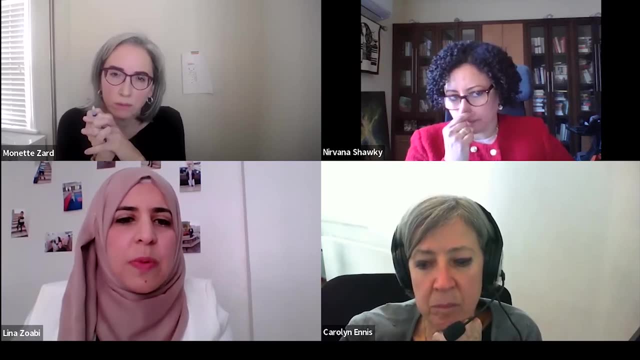 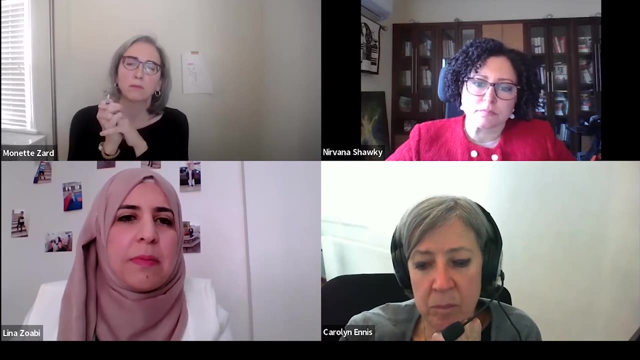 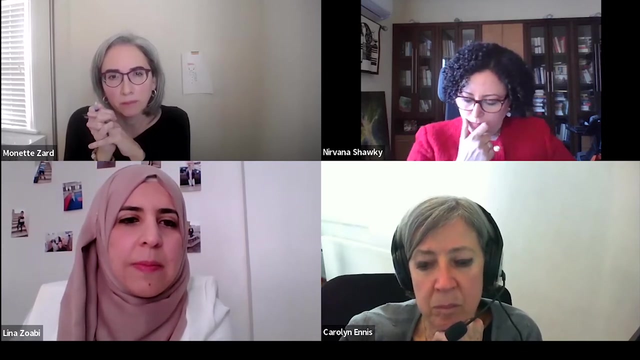 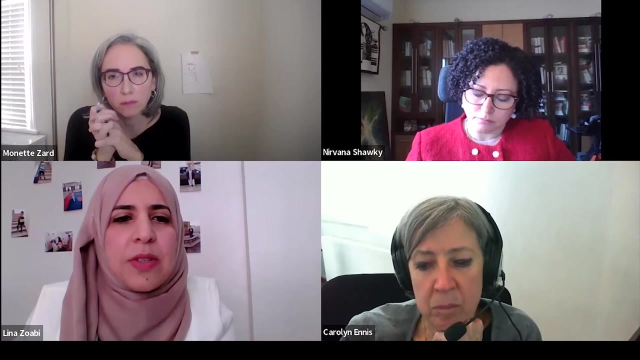 It's not available for more traditional female occupations or sectors, So the works opportunities tend to be like agriculture, domestic and textile appears to be for women, without needing even the permits. So their aspiration for a paid works they try to find a providing legal and social. 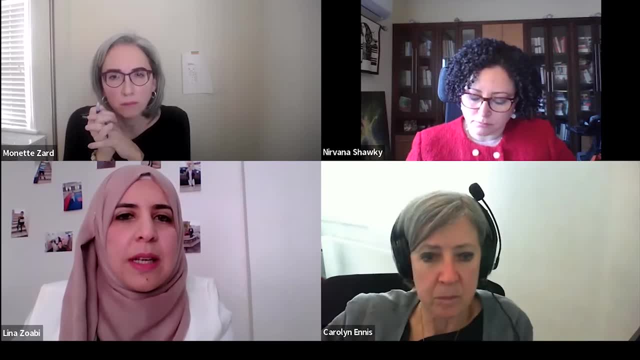 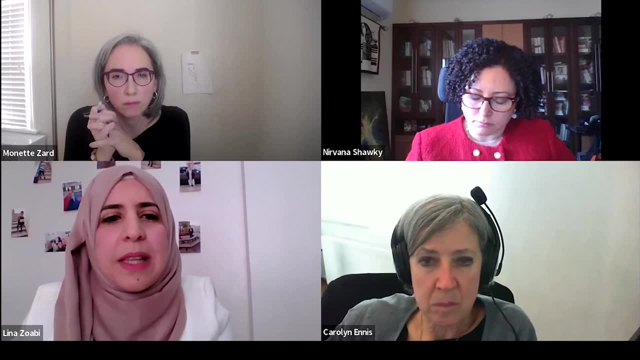 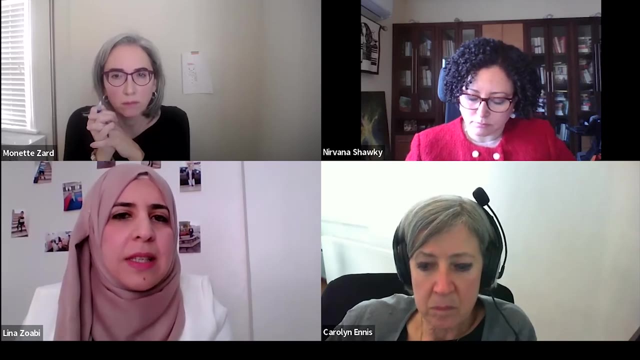 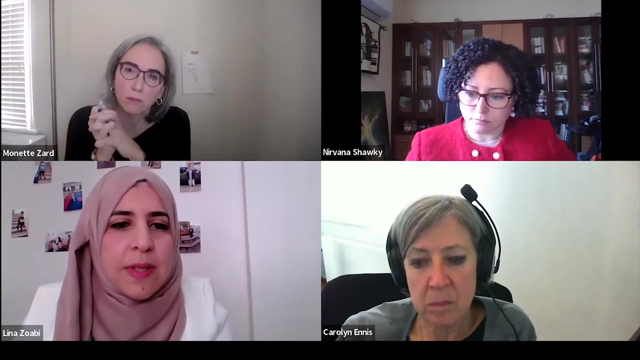 Protection so that they can work without any restriction, without any securities. Also, they can build a livelihood support. They can find the programs that they can support them and address the barriers for their jobs. Also, they aspire to find a temporary jobs opportunities, maybe through the community projects or the trading. 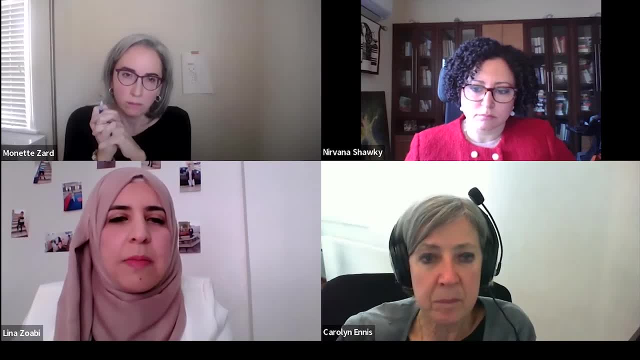 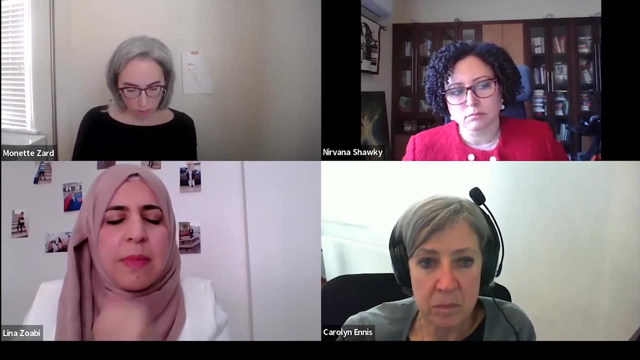 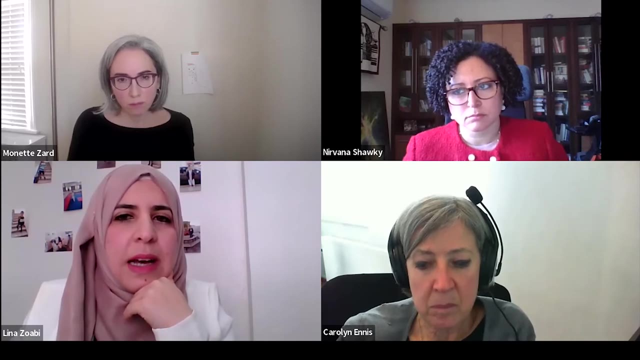 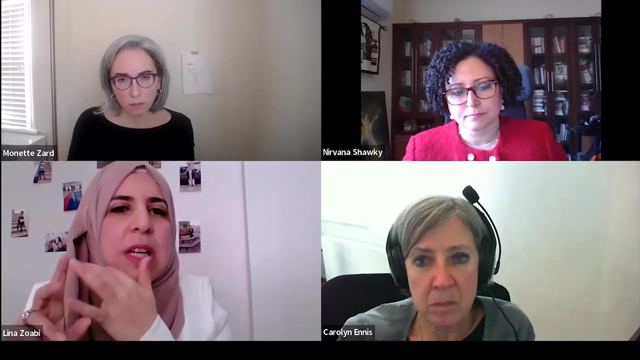 The leadership training, the pay job could also offer them a respectful life that they can live easily with their families and without being feeling insecure, As most of the women I interviewed they were. it was reflected on them psychologically, even socially, and from the financial situations also. 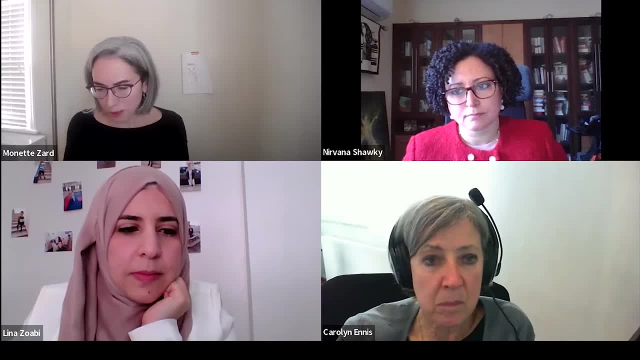 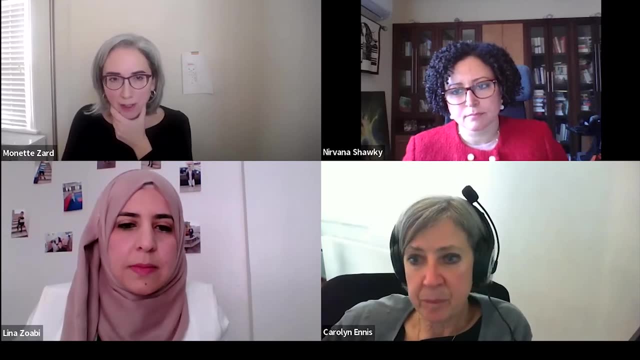 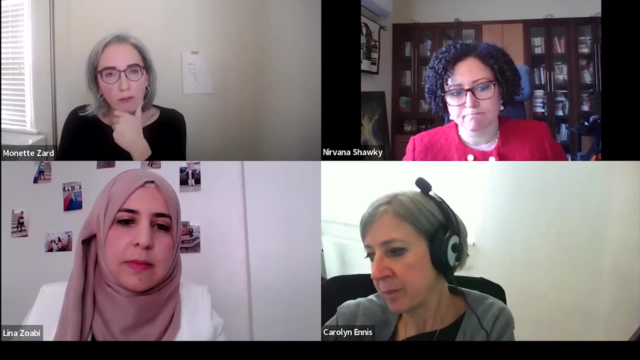 Thank you, Lina. That's an important perspective to add to our discussion today And I'd like to open it up to the whole panel. actually, I mean one of the we've been focusing largely on formal avenues for work. 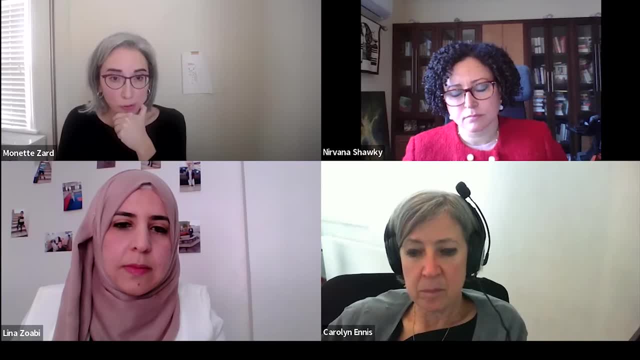 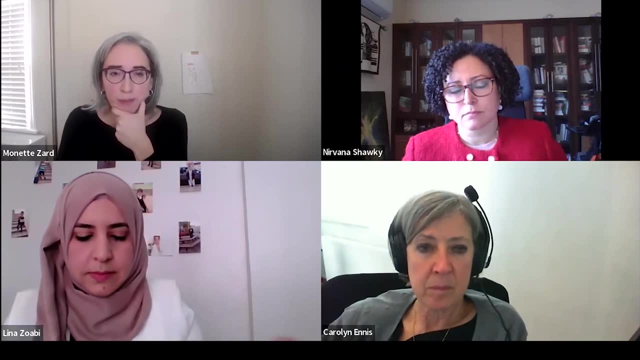 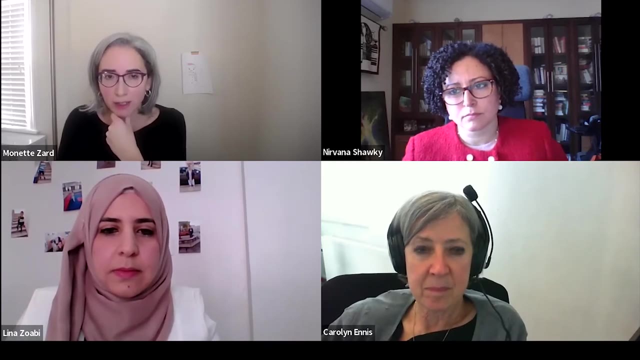 And the reality for refugees in general, but also for women, is that what often will be most available is work in the informal sector, And I'd be interested to hear your thoughts on that. I'd be interested in hearing sort of your reflections on how to engage with that aspect of the labor force. 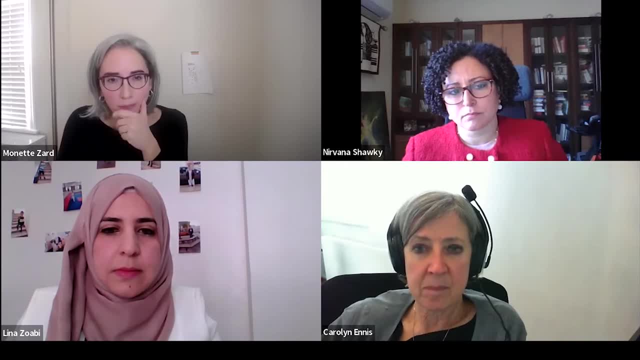 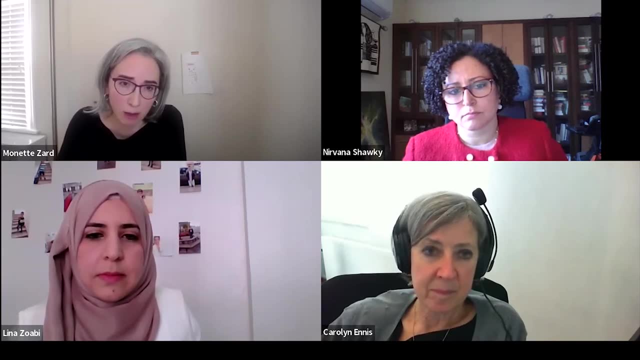 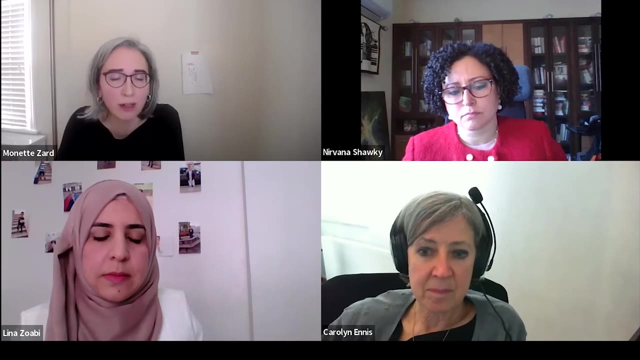 Because there the sort of aspiration of work, and work with dignity, is particularly challenging to ensure, you know, given the enhanced vulnerability that sometimes exists in the informal sector. So I'd be interested in hearing about any initiatives, either from HCR or CARE, around the informal sector. 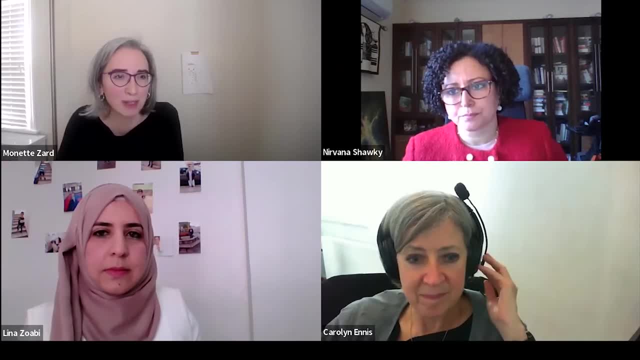 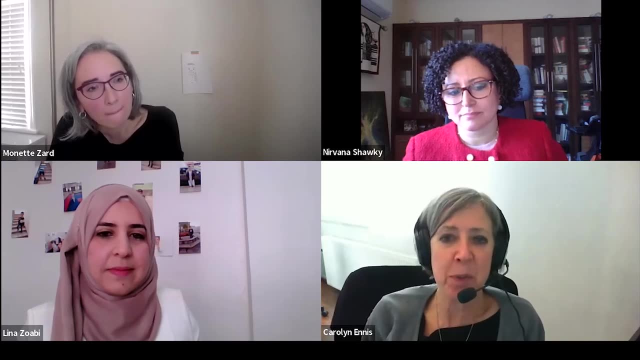 Carolyn, absolutely Yes. One of the things that we do that's really important and I also really enjoy is we meet with refugee communities all over the country constantly And they come and they talk about their problems And they're frequently not the problems you expect. 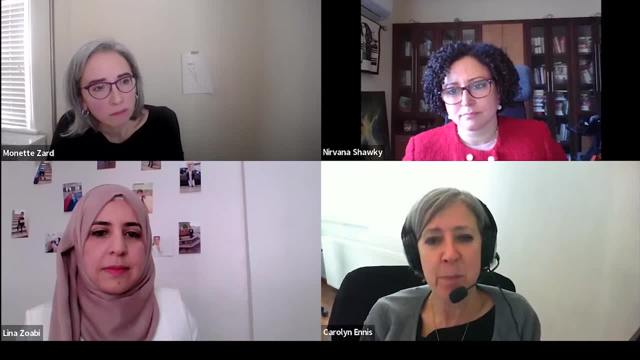 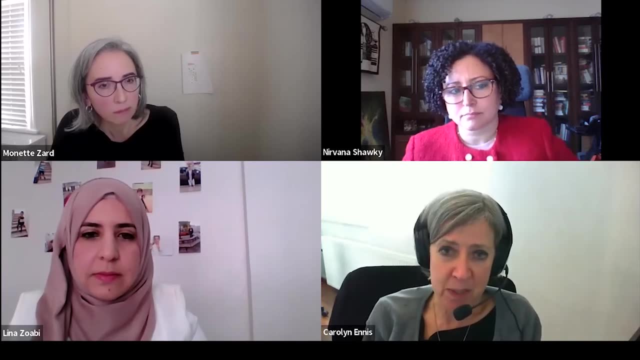 People will come and talk about the low wages in the informal sector And so we can talk to them about how that's exploitation and what they can actually do about it And and really talk to them about what they can do about it. And and really talk to them about what they can do about it. 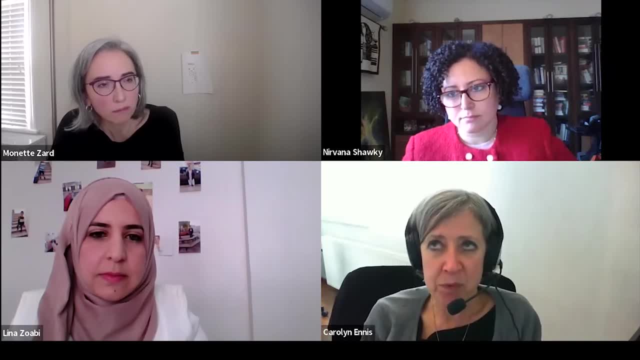 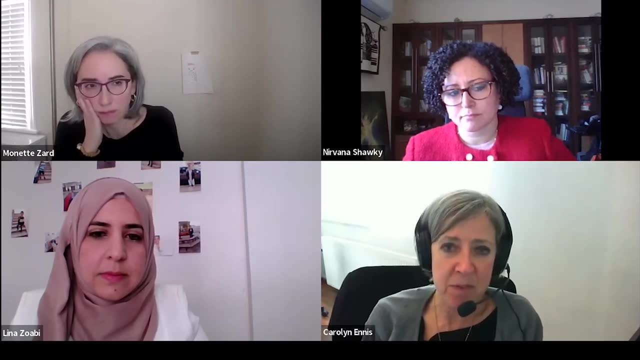 And and really try to support them. We also just listen to the refugee women regularly, And one factory was frequently factories advertised for women aged 18 to 30. And so we've discovered this like ageism in access to employment, and women who are in their 30s and 40s tell me: we want to learn coding. 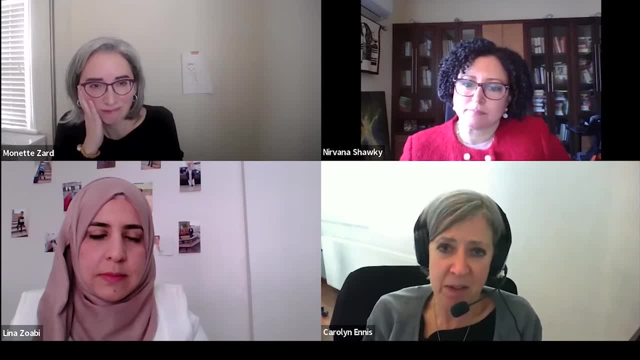 We want to be eligible for these factory jobs. Our kids are grown up or they're in school, And we don't have little kids at home who need babysitters, whereas the women in the younger age group actually have more trouble getting babysitters. 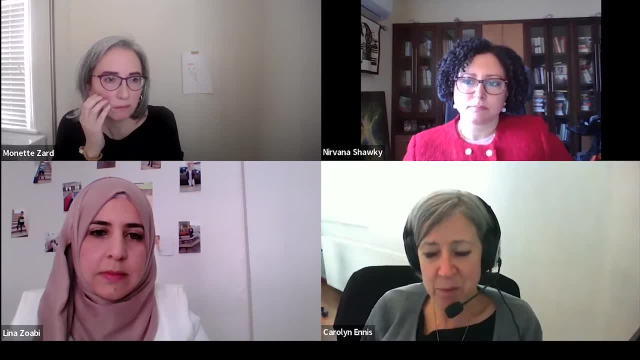 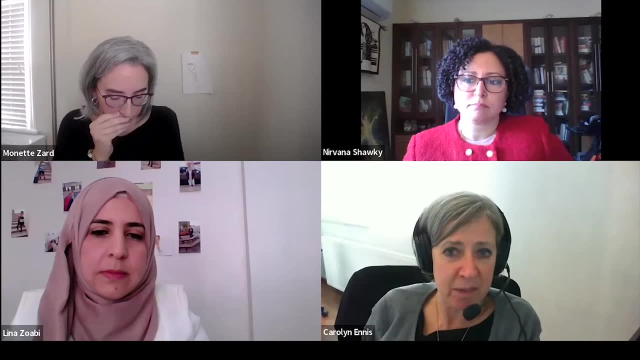 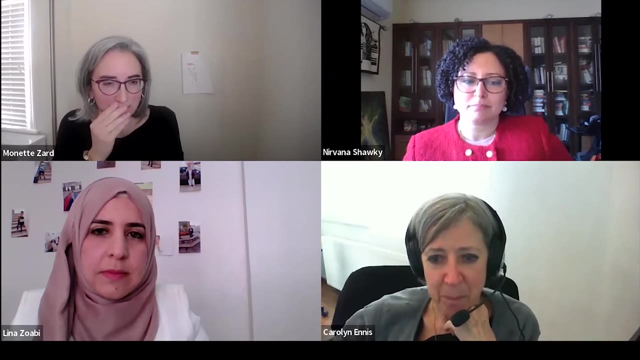 So there are a lot of ways whereby- listening to the community about wages, transport, access, job requirements- we can just find some quick, quick solutions. So those were two that sprung to mind from discussions in the last year or so Really really important. 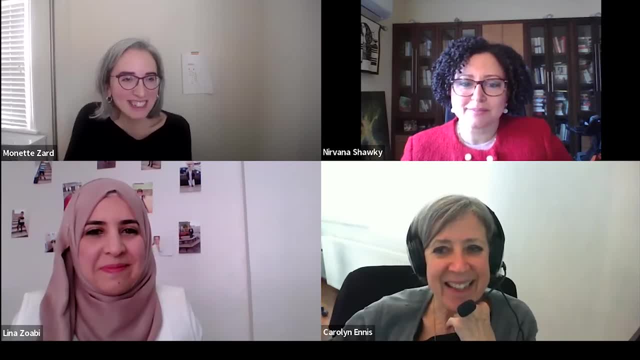 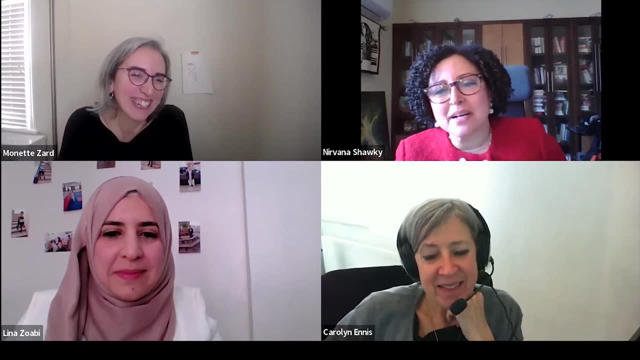 And Nirvana. I love how polite you're all being with the hands. Yeah, exactly, We don't want to. I mean jam the scene, Thank you, I mean, Caroline. you have actually raised very, very important examples. 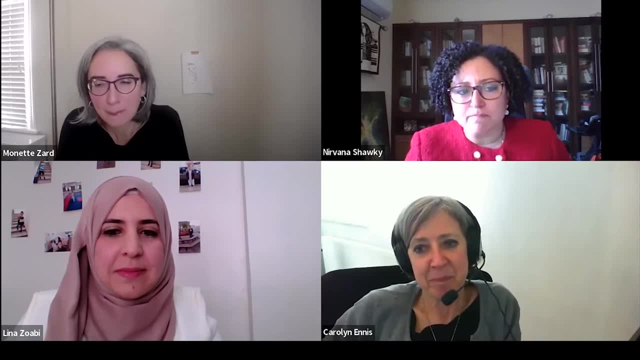 And I think that I mean looking at the informal sector and women. doing jobs that were previously held by men carries increased risk and fewer protections, And this is really one of the key points. I think that women are becoming more and more vulnerable. 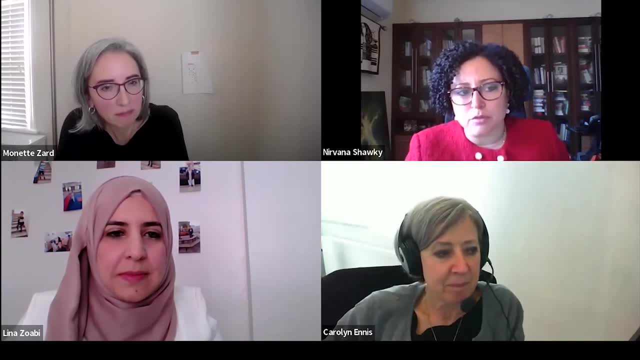 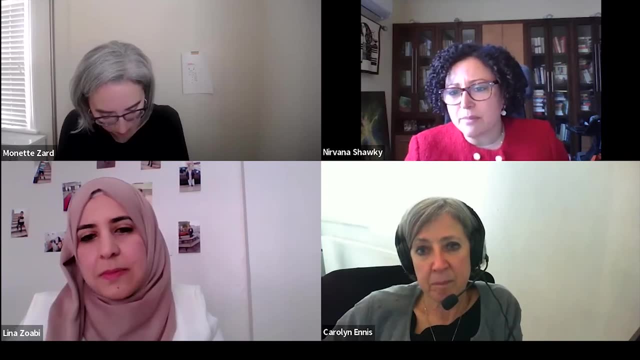 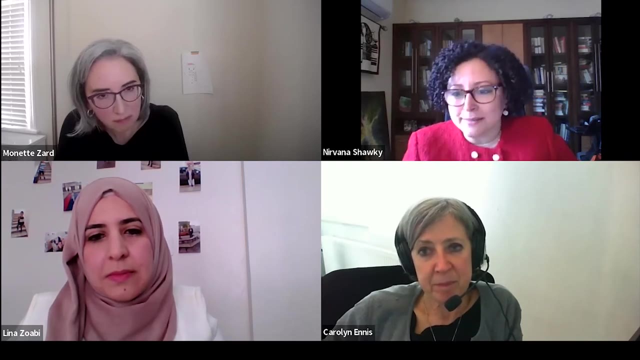 And I think that's one of the key points that we try to look at from CARE's perspective in our livelihood focus, Especially- that women are becoming now primarily responsible for the resilience of their families and communities in all aspects of their lives And have also gained new decision-making power, confidence and independence along the way. 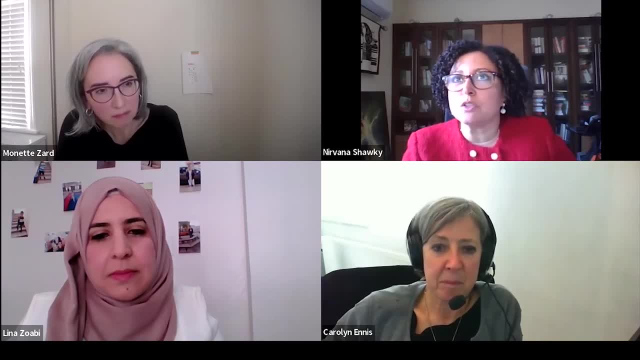 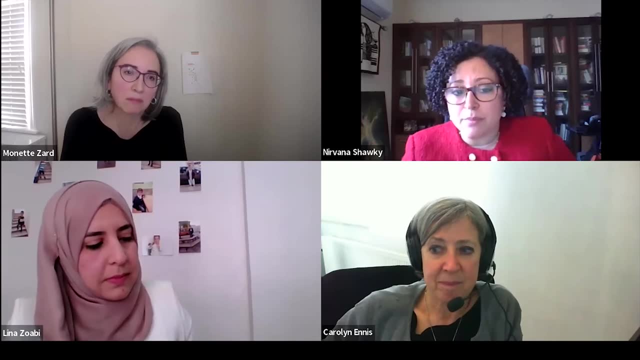 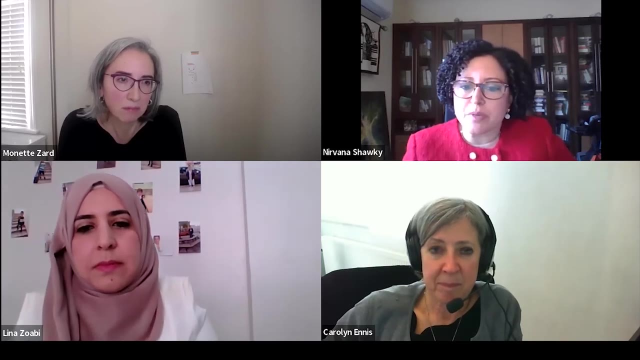 I mean- one quote I would like to share with you, As I mean, one of the displaced women in northern Syria told us, and I quote: these new circumstances have put me in the position of being both mother and father for my children. 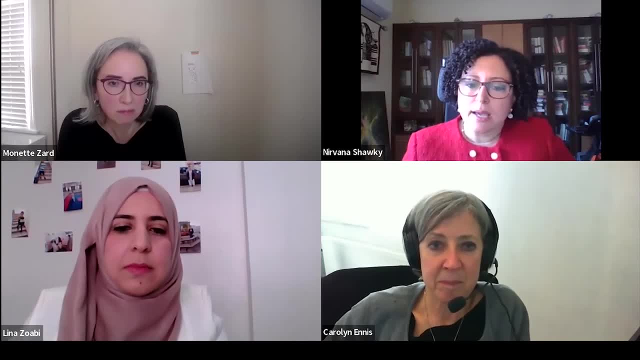 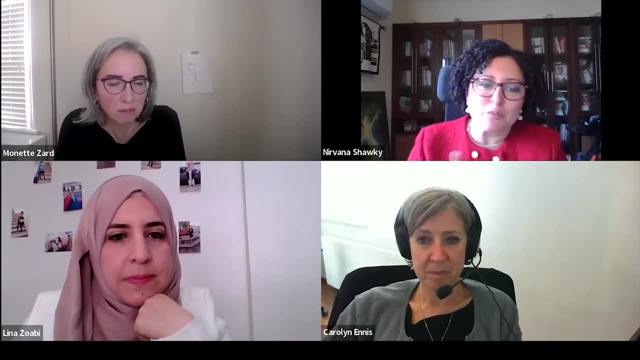 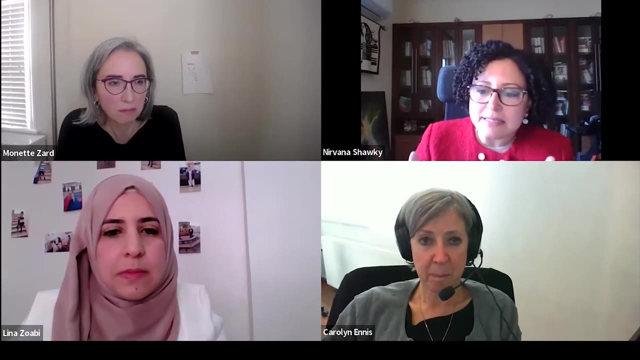 And this applies to most women in my community. The current situation has led to women's empowerment, And of course I mean with quotations and perceptions that we are now more equal to men, But the reality is that we took on the role of both males and females simultaneously. 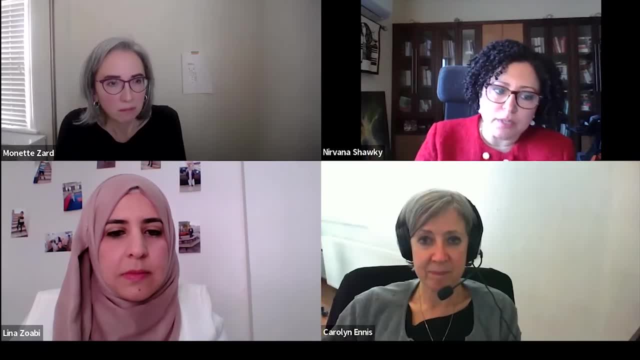 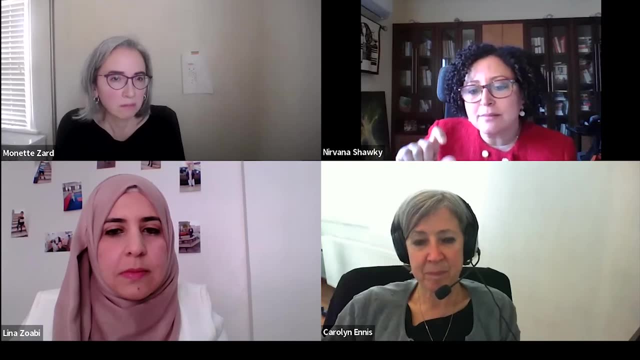 And now we do both jobs. end of quote. And I think that it is important to focus that the emerging role of women as breadwinners has meant that the overall shortage of funding for humanitarian assistance and failure to support the essential multi-year resilience and recovery initiatives. 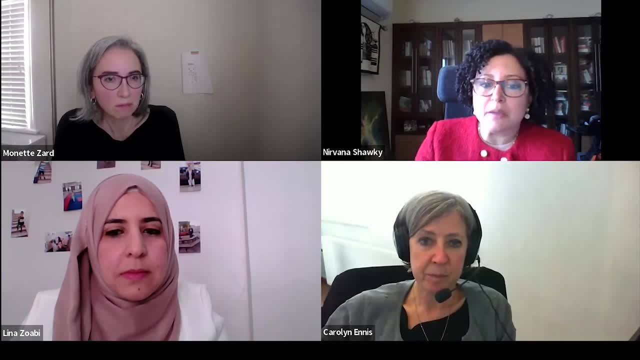 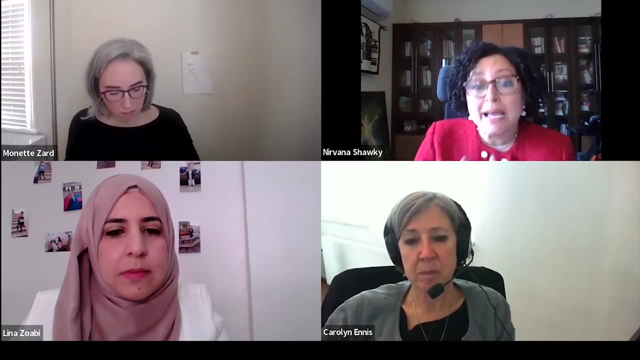 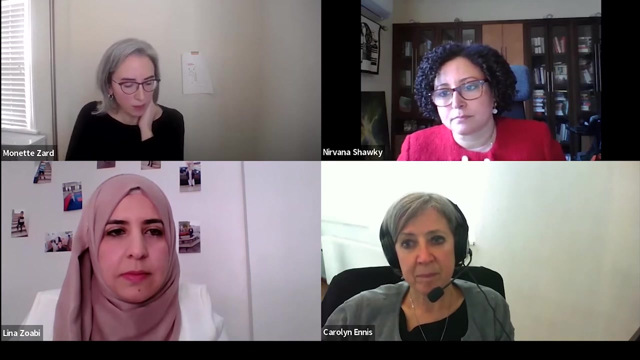 have a disproportionately negative impact on women, as it affects the ability of families to access the basic necessities for survival and jeopardizes the fragile yet potentially transformational changes in the authority and independence of women within their communities. Thank you, Thank you, Lina. I take it you do you want to jump in? 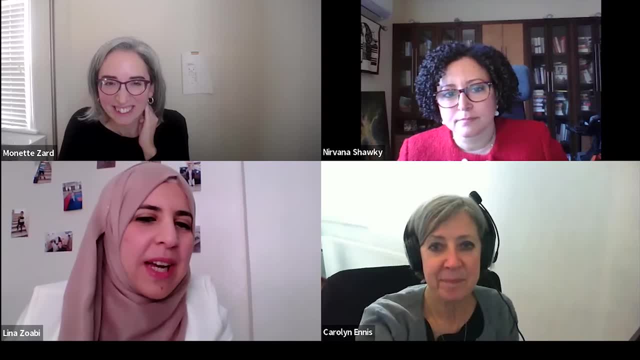 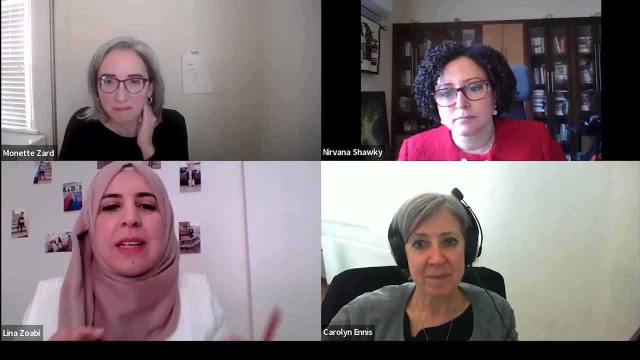 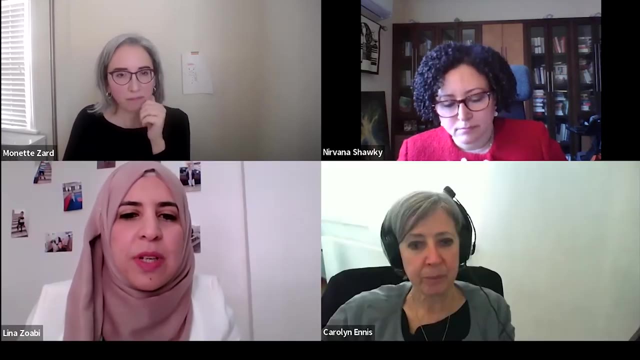 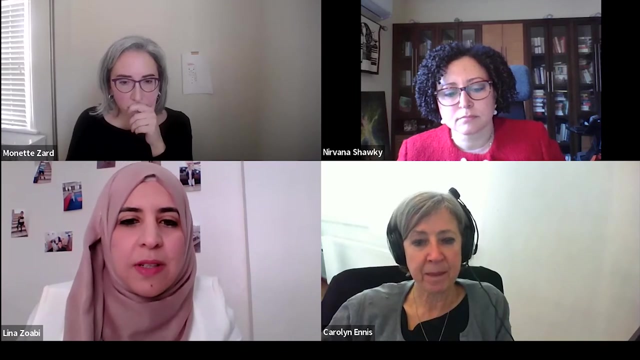 Yes, When I interviewed Syrian women, there was like a discrepancy between what they say. the women who has a family as a female breadwinner and their families, the women who are responsible for their families, The shifting rule and the double responsibilities that they had to supply for their family. 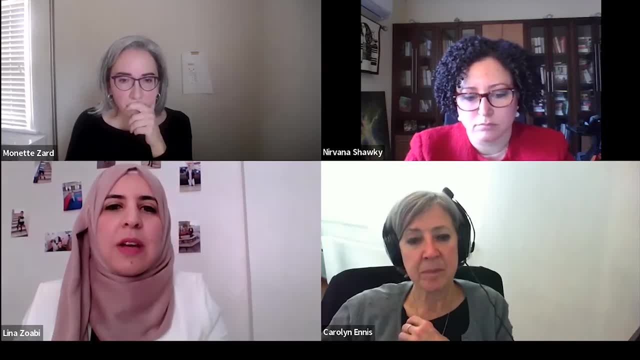 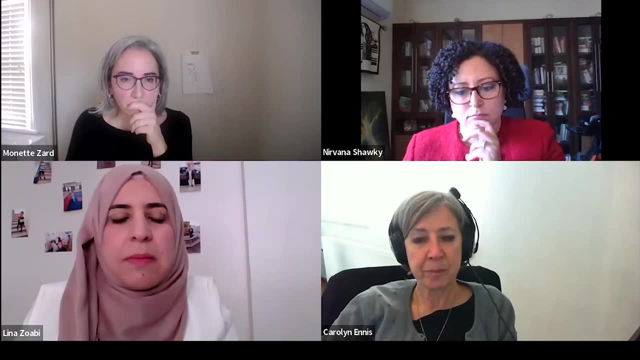 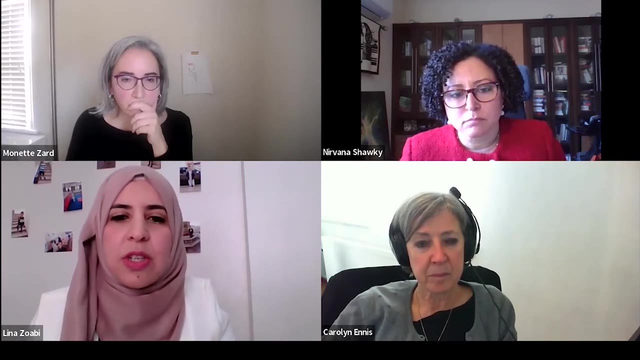 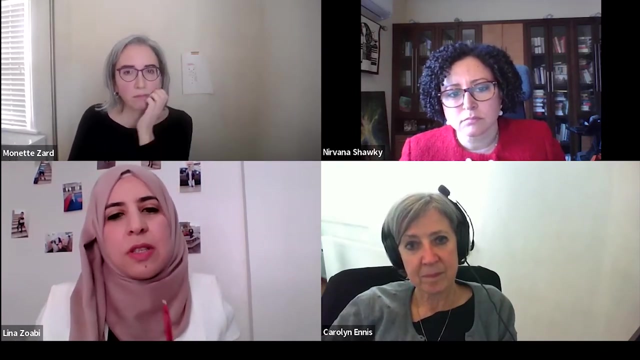 for them what they need for making a good livelihood, to be honest, affected them a lot, especially the mother. So I think having more attention or taking their situation more into account by the organizations or the different institutes, not only from the psychological or the social perspective, but also from the financial sides. 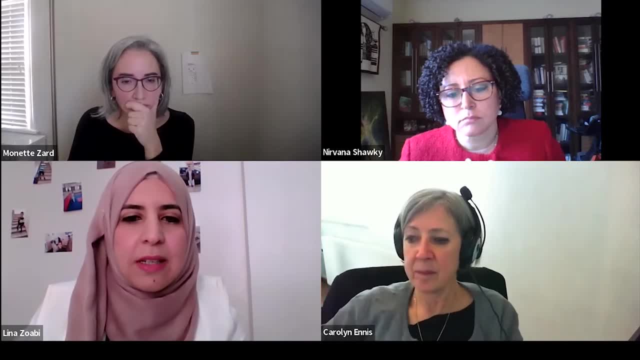 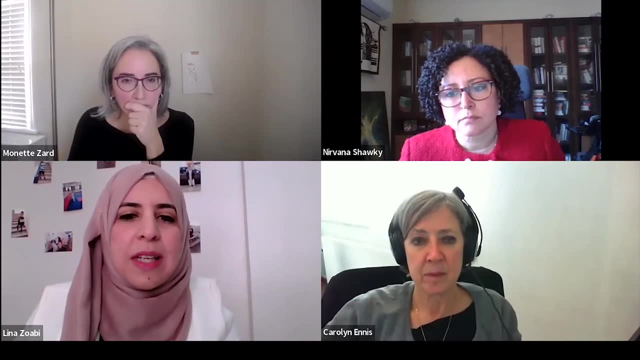 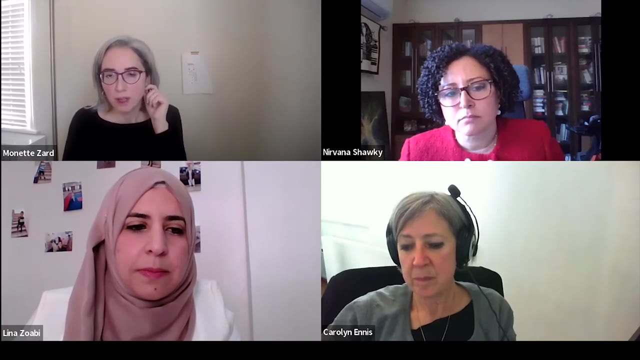 I think will not only affect her as a person or as an individual, but also the whole family. I think this will decrease the pressures on her from different levels. I can see the questions coming in quite fast in the Q&A box, which is great. 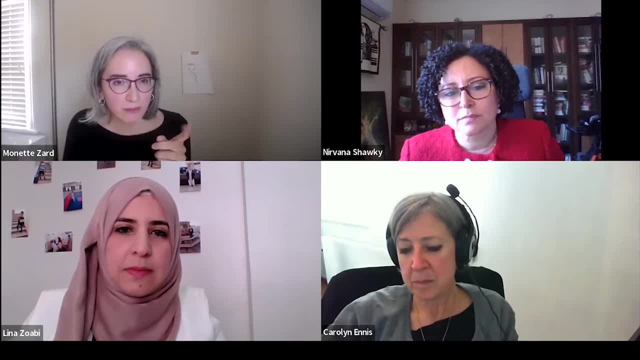 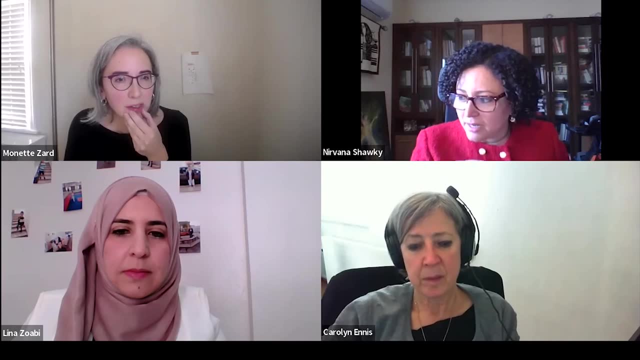 Nirvana, I see your hand went up. Do you have a final reflection on this particular question? Yeah, I just wanted to actually, because I mean we have a lot of questions. Yes, I mean, most of my examples, I mean, were focused on insights here. 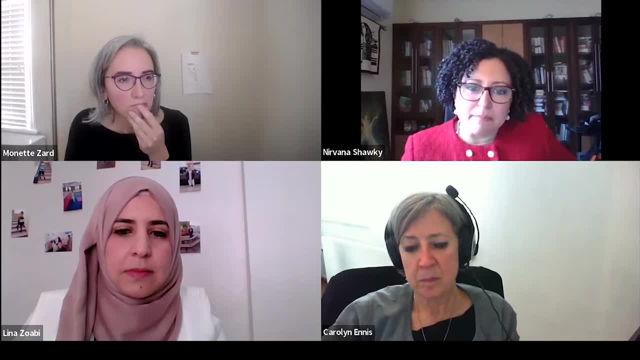 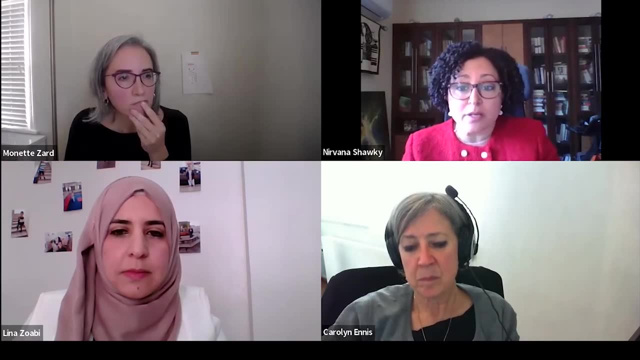 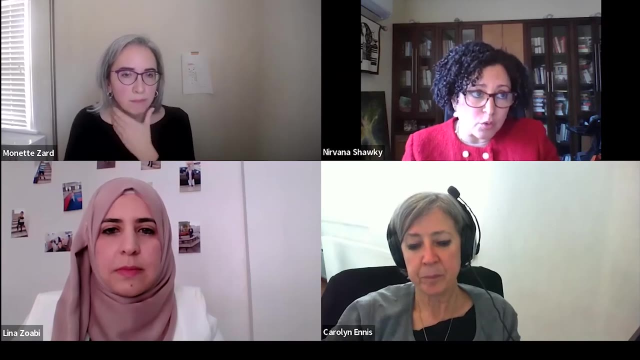 And I wanted to just give you a quick example. I mean as part of also the refugee response from our work in Turkey because, for example, I mean focusing on both the barriers wasting women and Syrian refugees in Turkey, but also I mean the solutions we have provided to overcome these barriers. 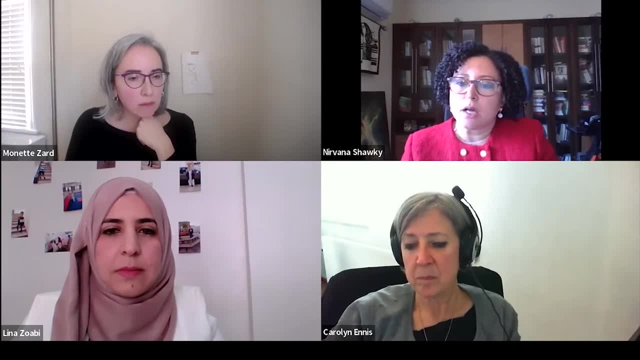 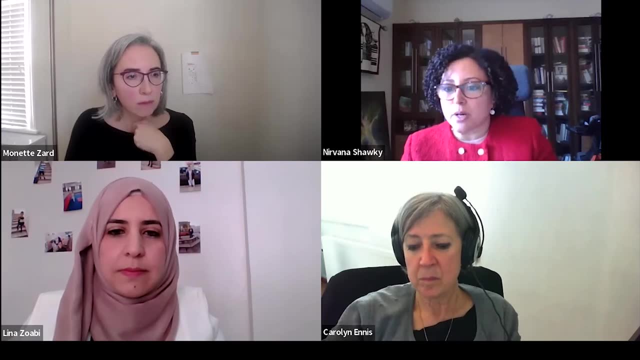 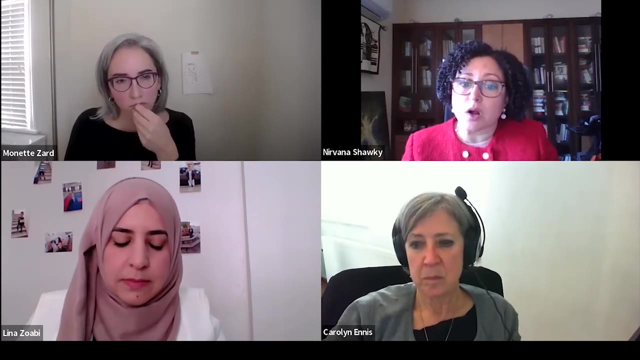 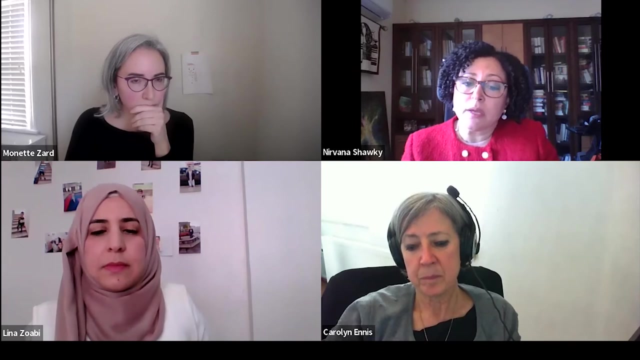 is that we have negotiated with Turkey's largest and most widespread bank to allow Syrian women to open bank accounts where they can save their money and have the required paperwork to grow their businesses. We have also worked with the garment and agriculture sector companies that can work with Syrian women on skill development. 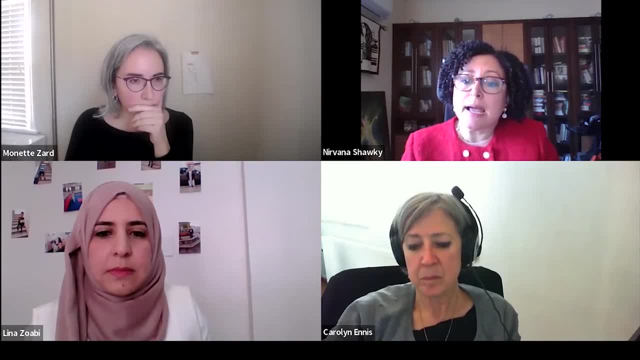 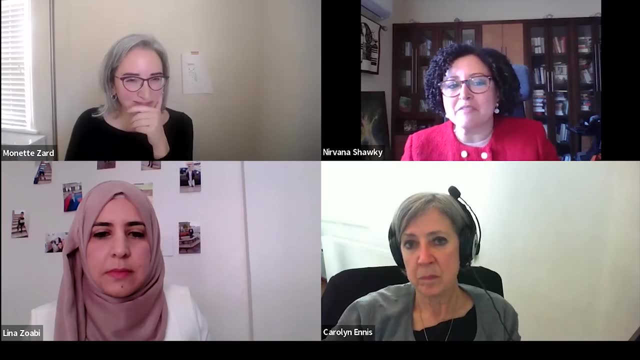 in interning with these private companies and being part of the formal productive cycle in the country. So I mean, I know that I've been trying to focus on the challenges, but I also wanted to highlight some of the positive examples as well. 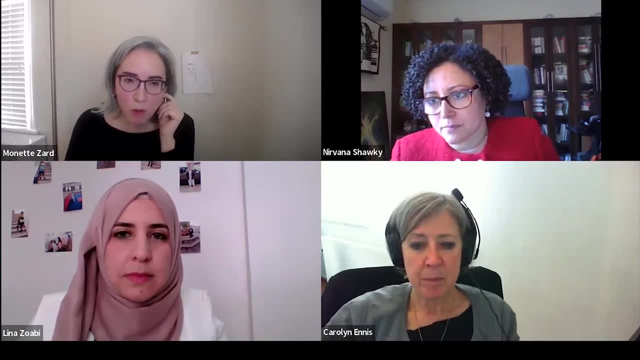 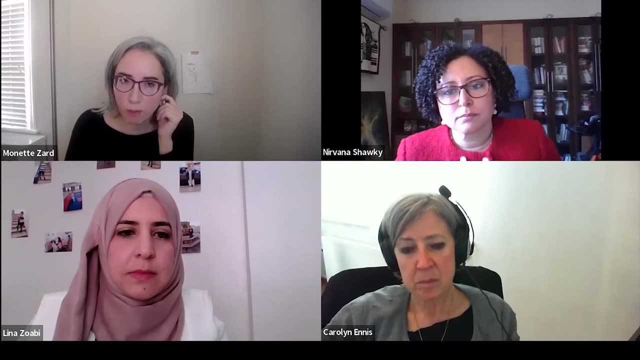 Thank you, Monette. That's great, Thank you. One final question from my side before I take the Q&A questions. A number of you alluded in your remarks to the importance of transportation as a key facilitator of, you know, women's ability to engage in the workforce. 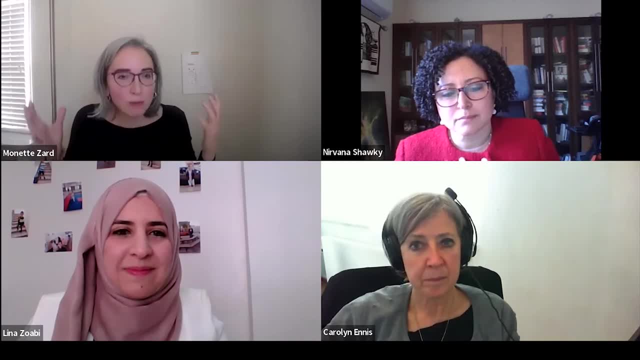 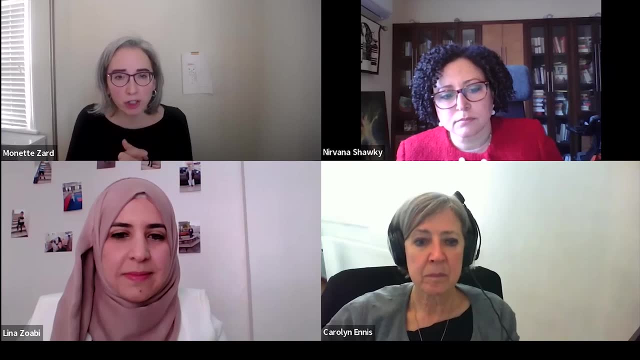 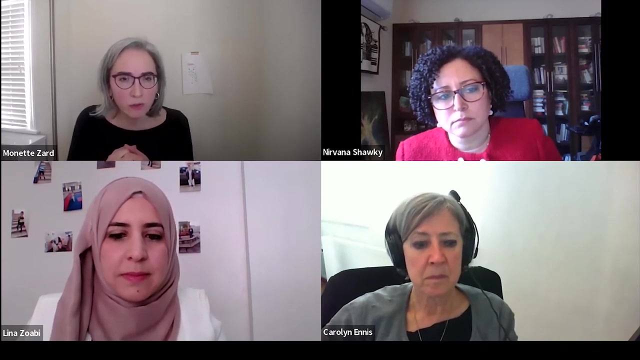 Obviously, transportation is bigger than any livelihoods portfolio or even refugee protection portfolio, So I wondered whether any of you would care to share some strategies, that are probably multisectoral, that allow you to tackle this particular aspect of the challenge that women face to more meaningfully, sort of engage in the workforce. 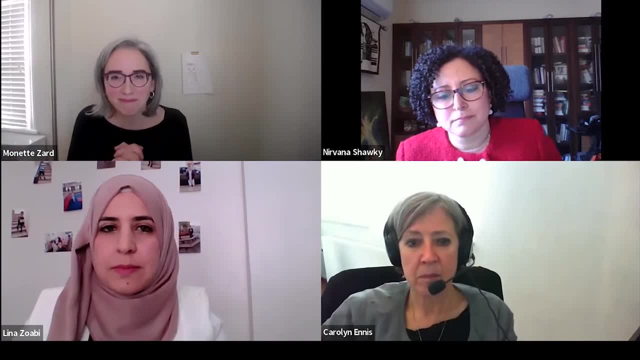 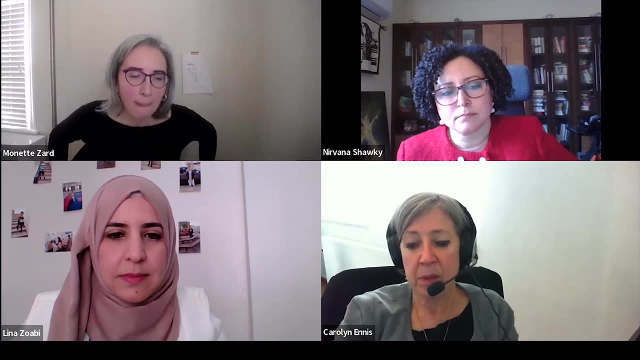 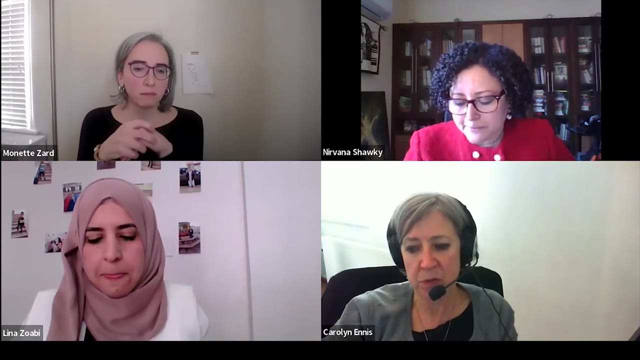 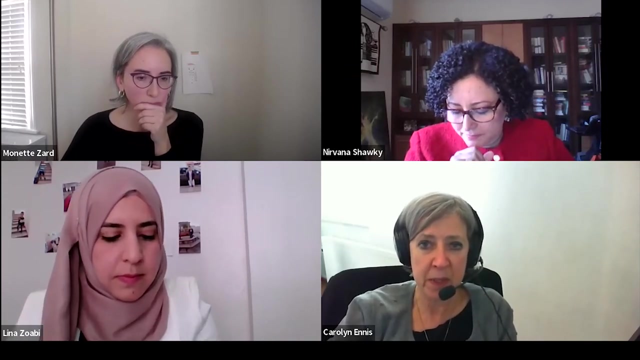 I'm happy to throw it open to anyone. It's huge just because of the safety, the cost and the safety for women in general, but especially for Syrian refugee women. So there are some garment factories that actually provide buses that take women in. 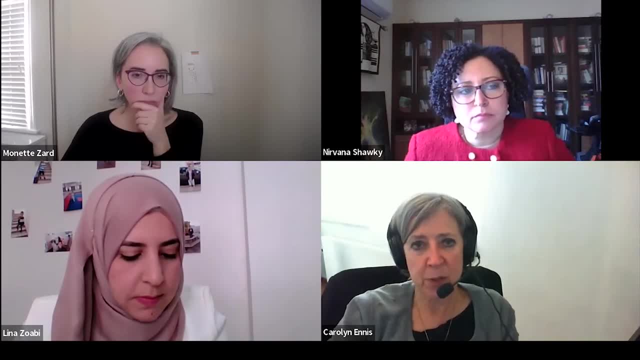 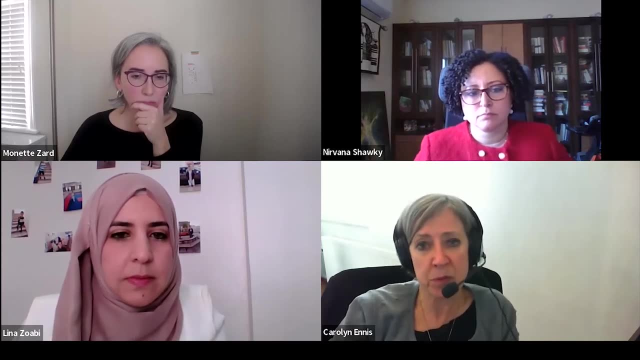 And some employers will actually provide money for transportation. But having safe transportation where women won't be subject to harassment and where daughters can go and get to work and then not, you know- face the shame of being harassed and having their families finding out. 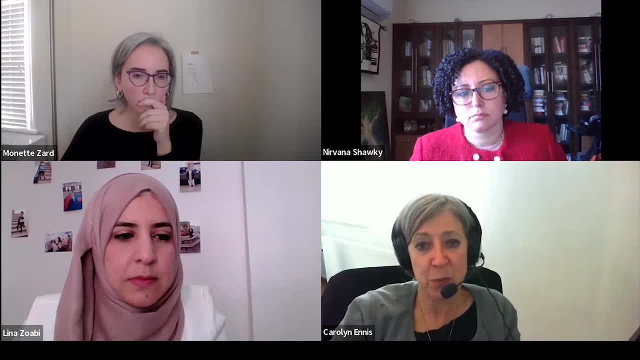 it's a huge challenge added to the, you know, the challenge of transport in general. Amman is a huge city and we have a map of where most refugees are And the highest concentration are actually in Amman And some refugees will actually travel. 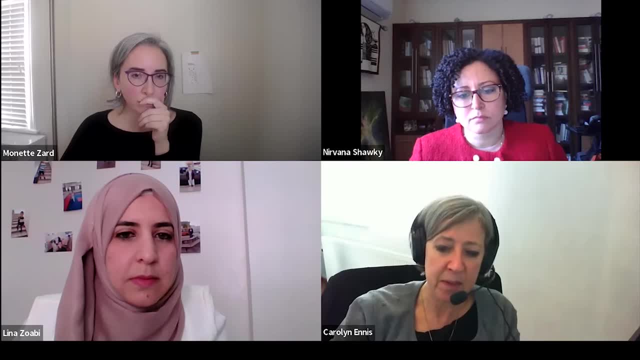 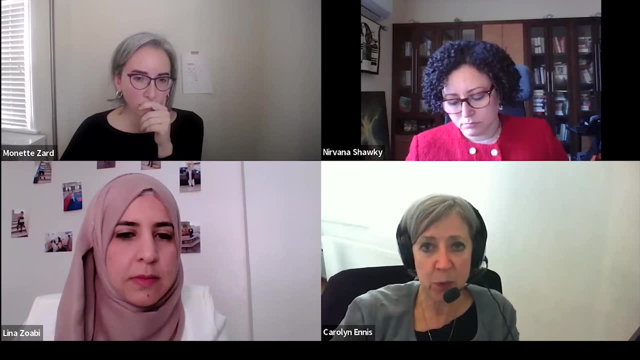 Some will actually try to, you know- live on the farms, where they work in tents, and that's illegal. So safe transport for women is really, really key. Allowances for transport and buses provided by larger employers are the best coping mechanisms that we've seen so far. 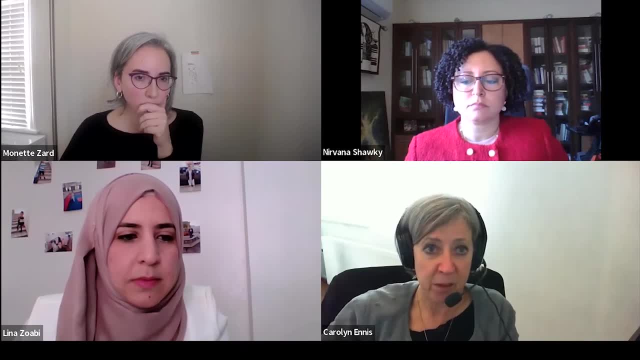 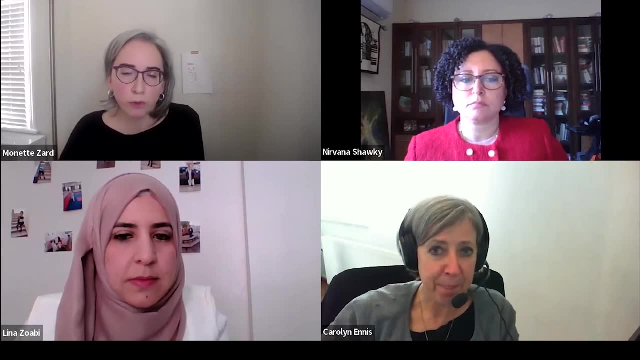 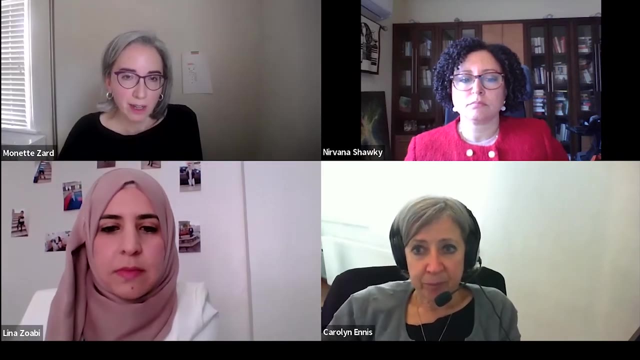 But it continues to be a huge challenge. Great Thank you, Very helpful. So I'm going to move to some of the questions in the Q&A And I see, looking at them, that there are a couple that come back to this question of working in the informal economy. 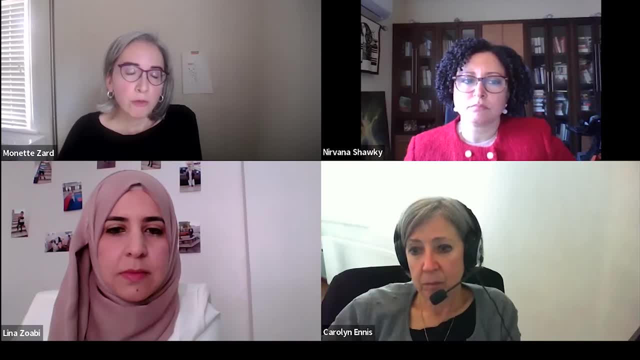 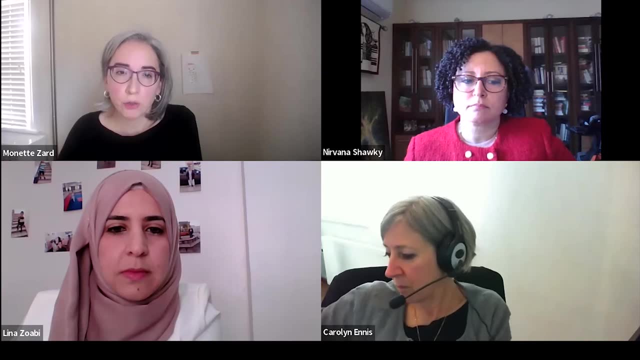 So there are three questions that I think sort of resonate with each other. One is: what is being done to advocate for refugees who are working, though not legally allowed to work in places like Jordan, So outside of the work permit system again. 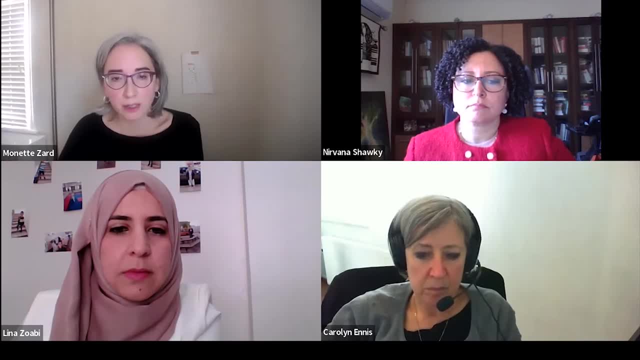 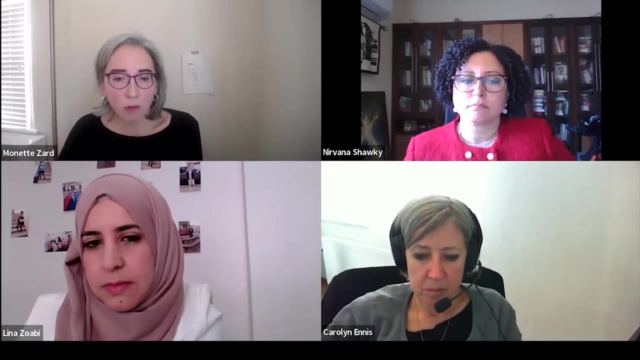 I think women are likely in a position of some vulnerability because of their engagement in the informal workspace. So what's being done to advocate for those refugees? That is one question. A second one that I would like to roll into that is: well, how do you support women in the informal economy other than conducting FGDs? 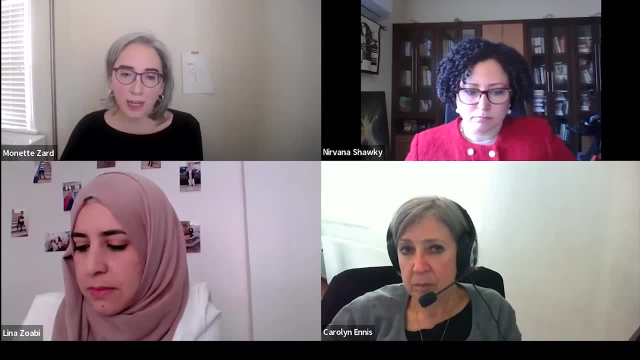 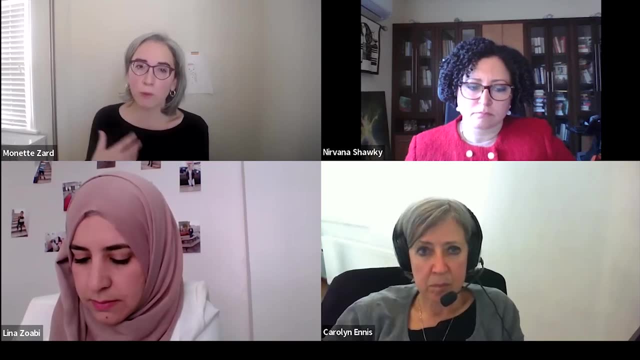 Are there any concrete solution examples? I think you know we started to hear some of that from Carolyn in terms of you know the sort of clinic-like atmosphere of talking with refugees about some of the challenges they're encountering in the workspace and alerting them to what is exploitation. 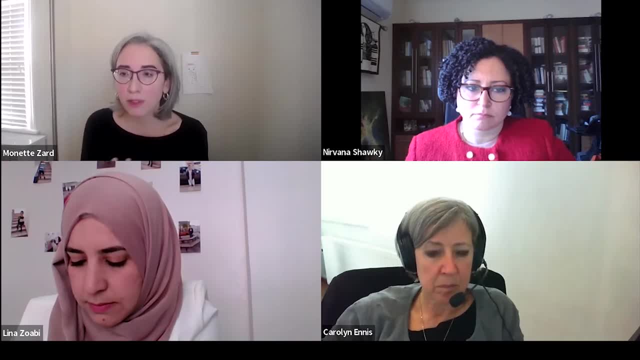 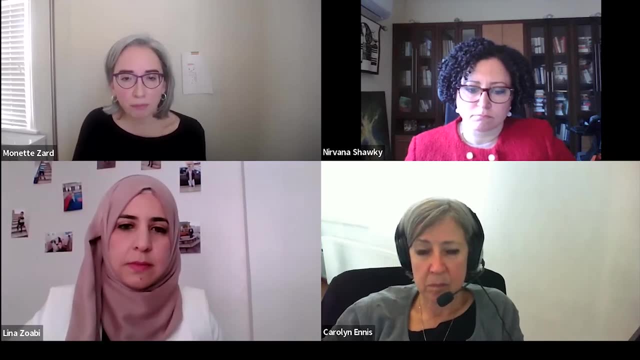 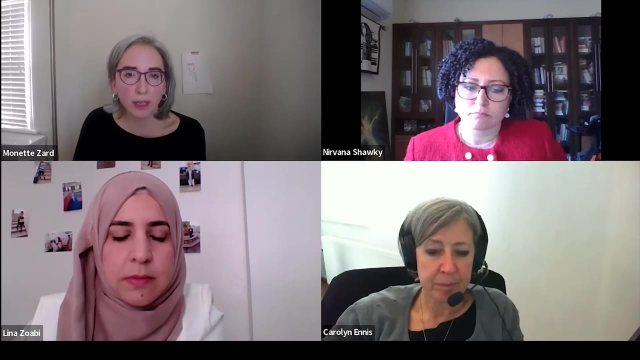 But perhaps you can build out some of the other services that might come with supporting women in the informal sector. And then let me just see That was another one that related to the informal economy. Well, there is one that relates to flexible work permits and what impact they've had and what the obstacles might be to issuing these work permits. 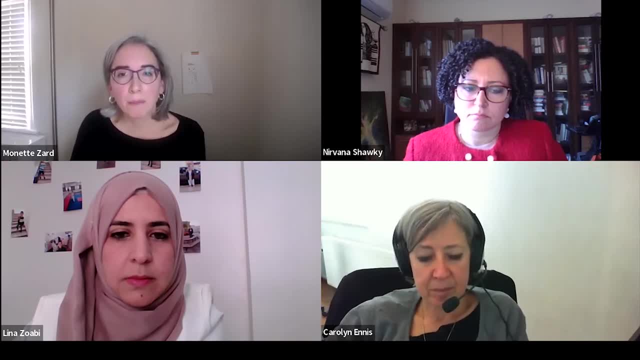 So I'm going to cluster those three which, broadly speaking, I think, address, you know, the constraints of formal work and the challenges of informal work, and see if any of our panelists would like to add to that. Yes, I think that's an excellent question. 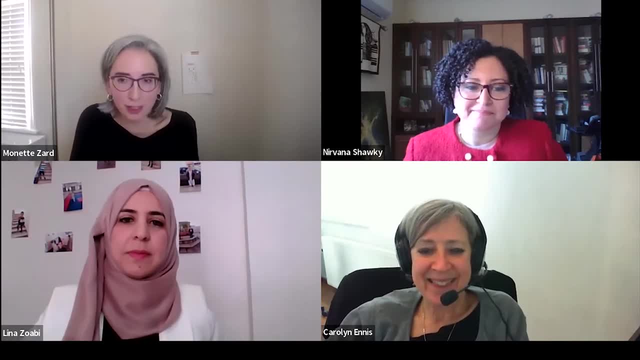 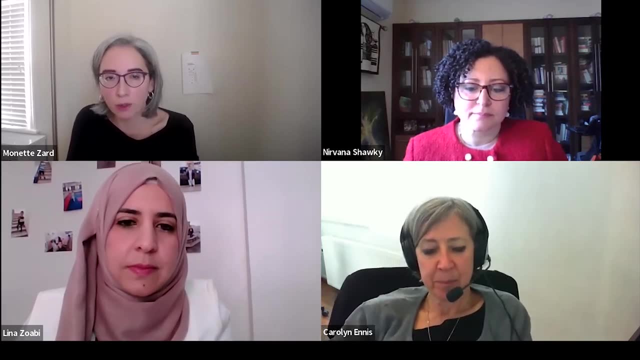 I think you may have plenty of questions there. I think we'll have time for one or two more people to think about. I think I have time for one or two more people. I think I have a couple of questions. One is from Carolyn, who I know is a professional who has worked for the ILO since 2019.. 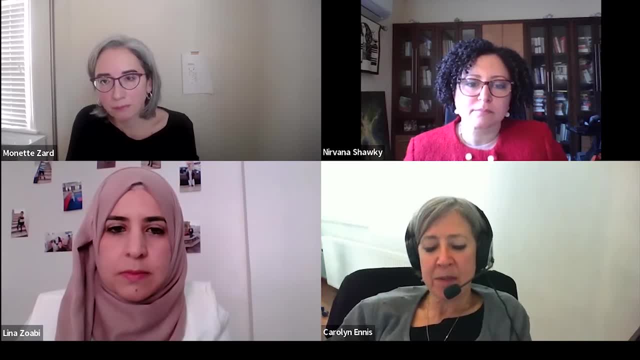 Can you talk about how those congratulations and those support agreements- and it remember, have you had anyConnell так? you can talk about, you know, describing situations of exploitation? How would you go beyond that in the work that you do with women? Well, let's maybe go back to the improvement in the management by the government and the ILO and partners and refugees of FGDs and the work they do. 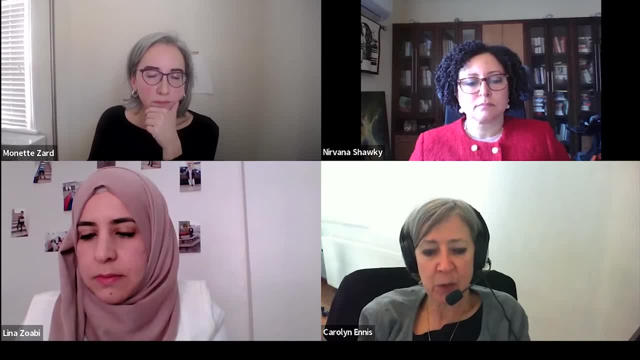 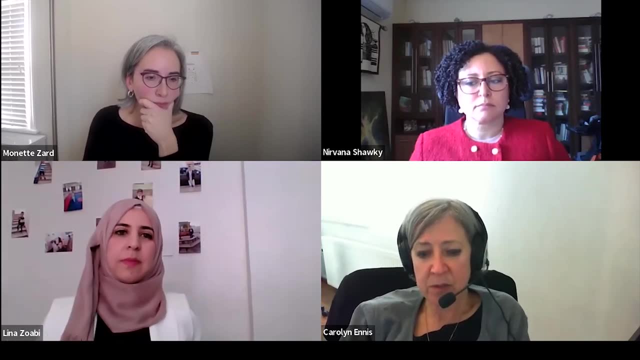 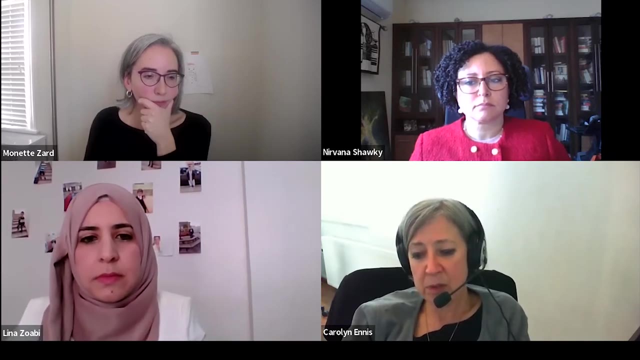 One is that there is a growing population by the government and the ILO and partners and refugees of the now flexible work permits. a total of 288,876 work permits have been issued, 271,250 to men, 17,626 to women. 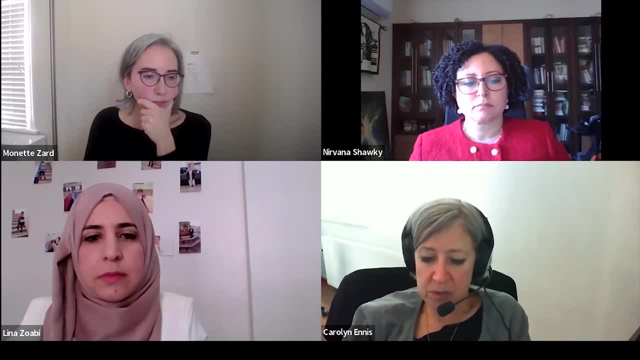 And since 2020, the Ministry of Labour announced the list of occupations allowed to non-Jordanian workers by economic activity and allowed issuance of flexible work permits for these occupations. So once you have the work permit, you can go out and have several different jobs with it. 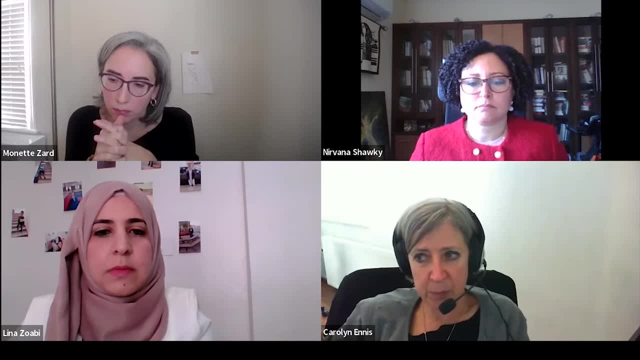 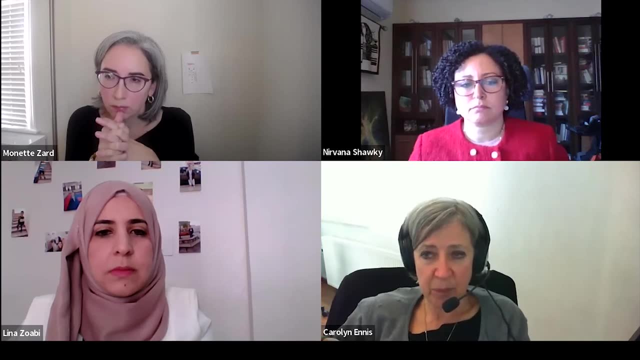 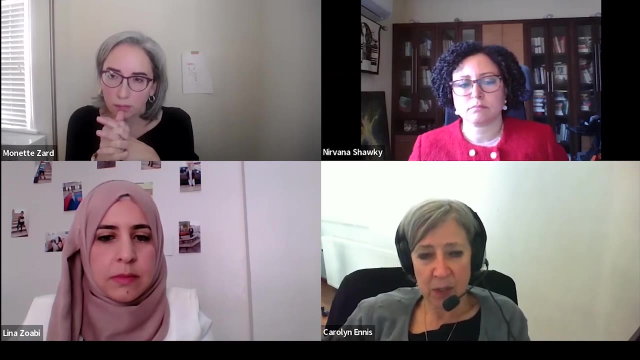 So the environment is certainly being improved. The informal job market is definitely a challenge And we can try to counsel refugees regarding the best approach would be to have a work permit, and then you actually will have something like a contract with your employer. and try. 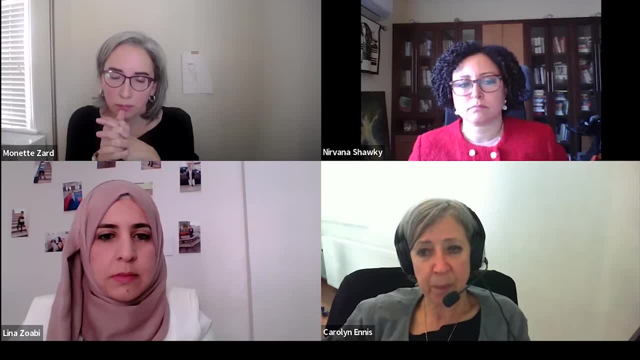 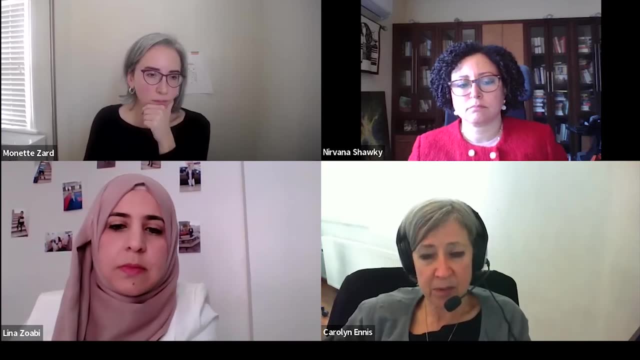 to have decent conditions So you can find ways to do that for your work permit. We have seen, and I think is one of the most important steps has been: the government has put in place this project, the international work permit, which is going to look like a 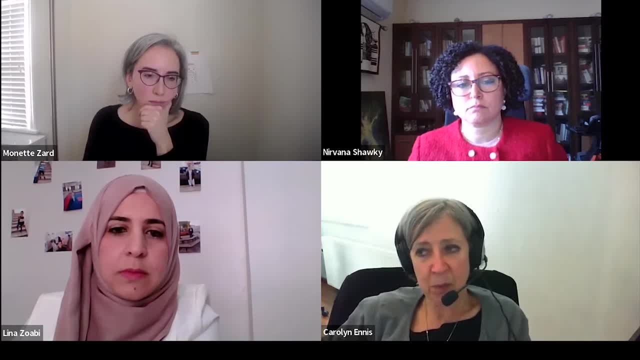 work permit for a non-Jordanian worker in the labour market, or really a non-Jordanian worker in the labour market, and there will be some work permits which will be founded for youth in the labour market, and then there's going to be that will be funded into some 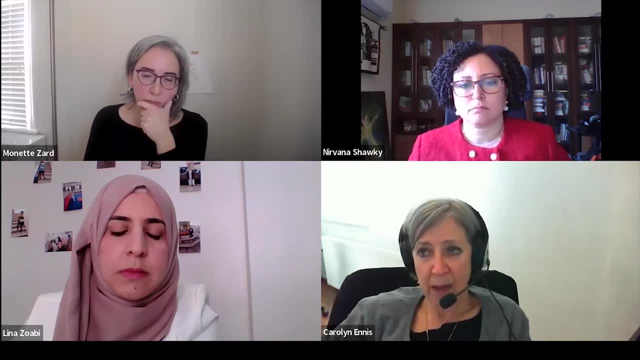 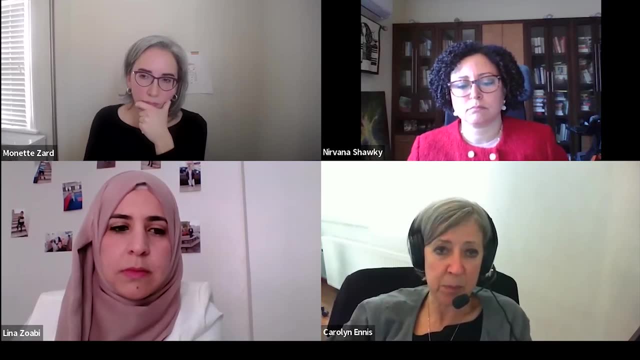 ettres, where I think the working permit is going to be given back to a worker who has been employed before. Thank you permits that they've applied for as a migrant worker and it's quite complicated, if not impossible sometimes, for refugees to obtain these work permits for non-Syrian refugees. 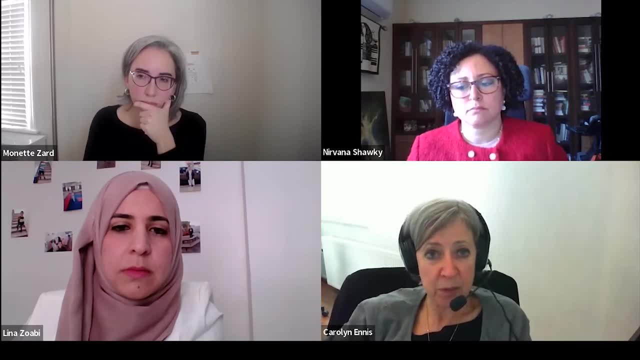 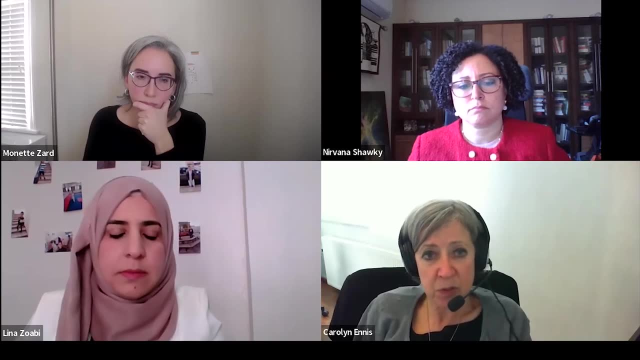 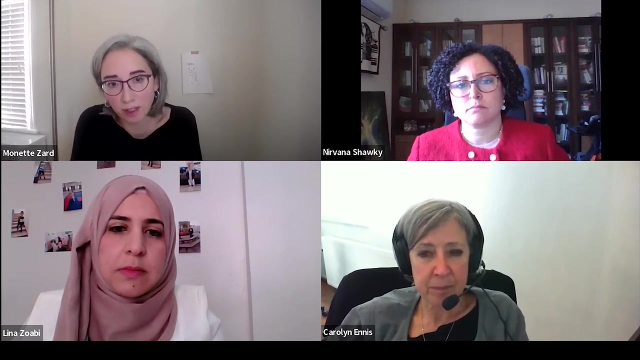 This is challenging and something where we are working closely with the government to minimize protection risks to refugees and to really, you know, promote refugees having the permission to work that's required for any foreign worker in Jordan. Yes, I mean, I think, the size of the informal sector in many of the countries in the MENA region. 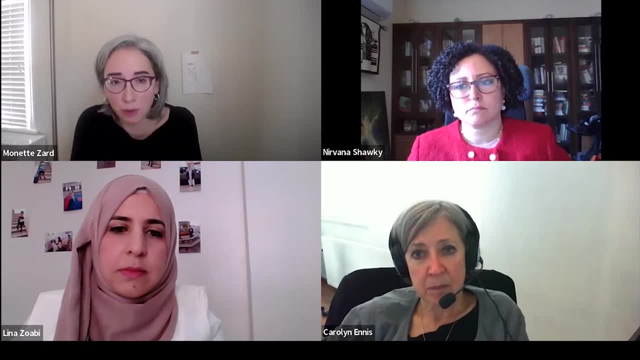 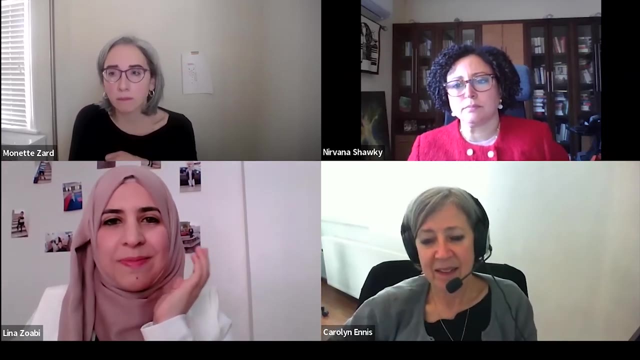 you know, points to some common vulnerabilities and areas where I think strategies that do focus on both hosts and refugees can be really quite productive. Lina or Nirvana, is there anything you would like to add to that? Yes, Okay, Okay. 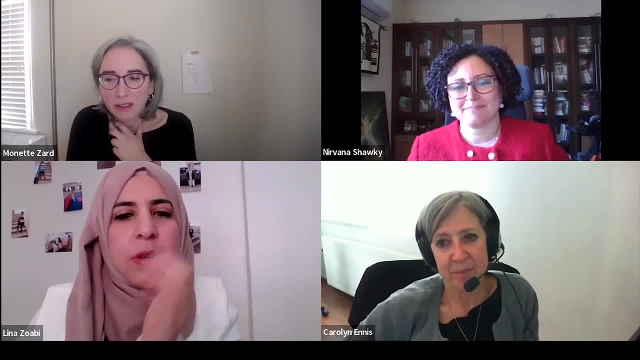 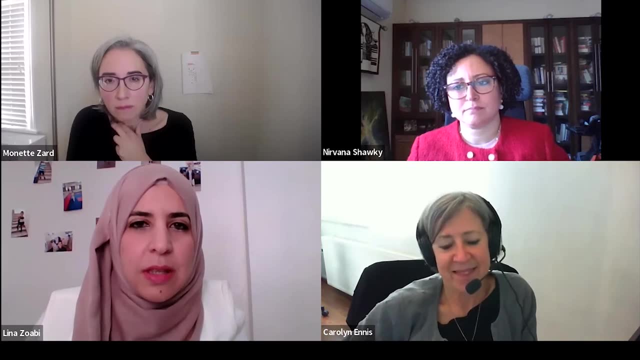 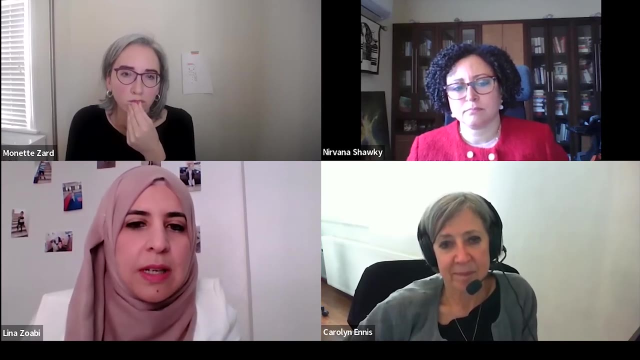 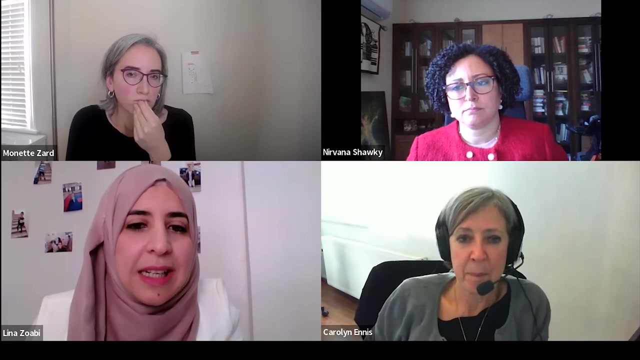 Yeah, Related to Jordan, I think. starting from 2018, they issued work permits for home-based business so that it can be legal to work. I think this gives a lot of opportunities for families to work legally, although most of them used to work- let me call it in such- an illegal way. 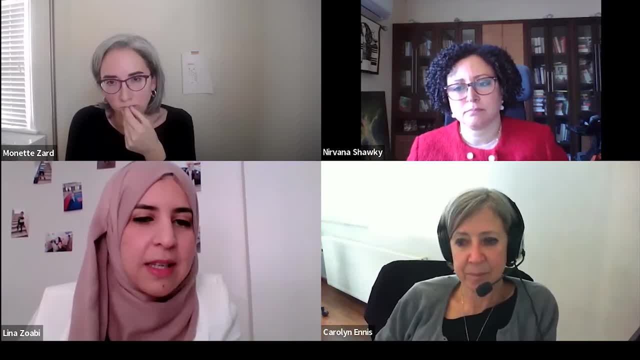 However, they were faced differently. Okay, Yeah, I think it's very important that they are protected. I think it's very important that they are protected. I think it's important that they are protected. It's important that they are protected, but also that they are protected in different. 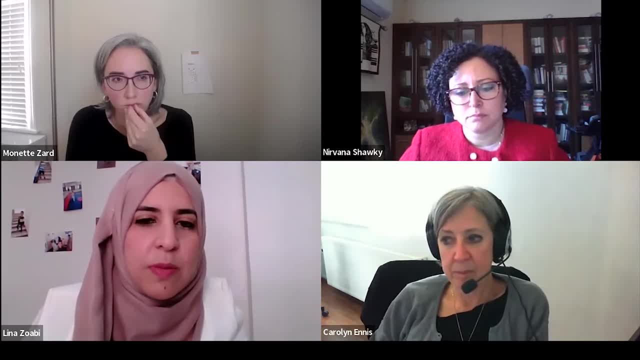 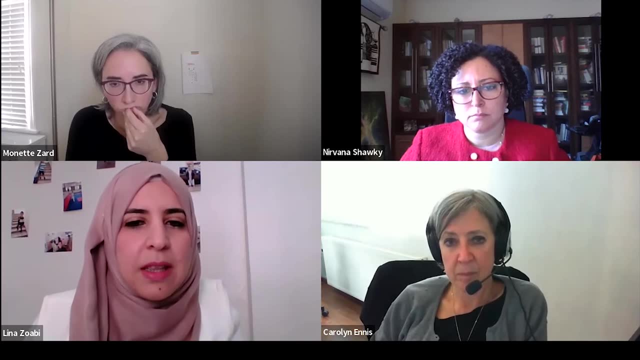 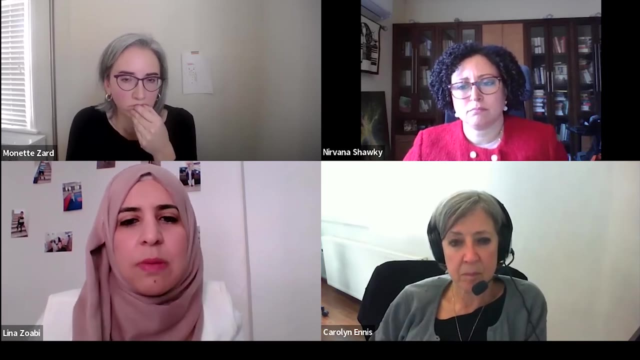 situations that they were exploited or were exploited, And by turning it to legal way with permits. I think this is ensure them safety and protection and getting the most of their rights. Even this will be more productive for the countries that they reside in also. 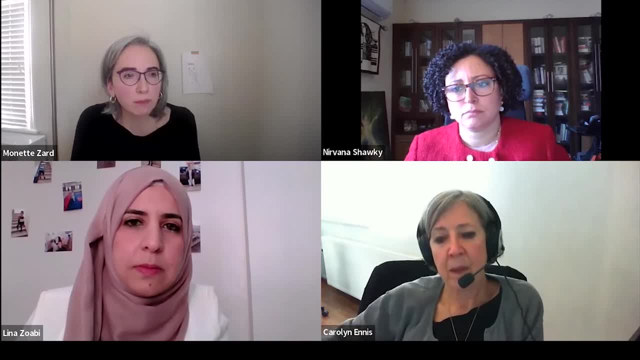 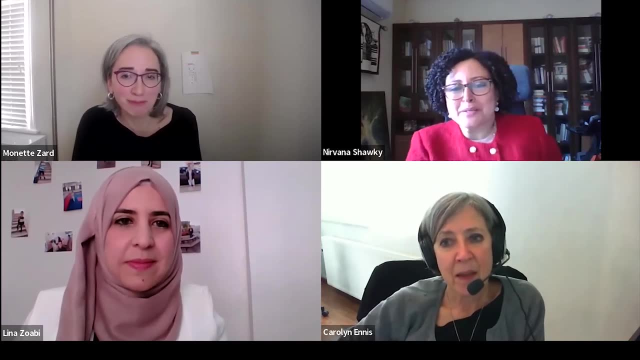 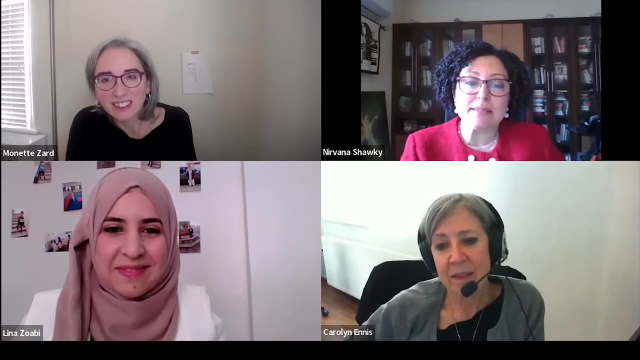 Great, Great. Thank you. I'm happy to take a couple more questions if you don't have anything to add. Nirvana, No, actually, no, Yeah, I was actually struggling to unmute. I mean, I wouldn't actually try to repeat what Caroline and Lina have already covered. 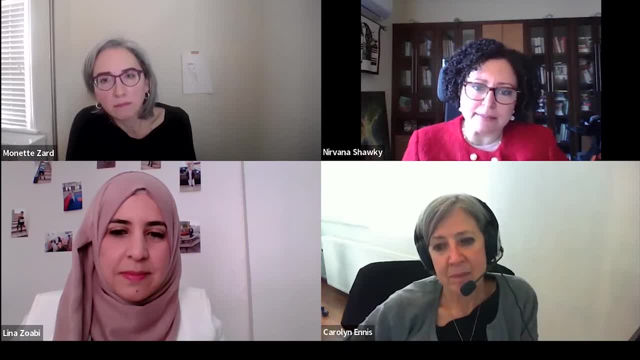 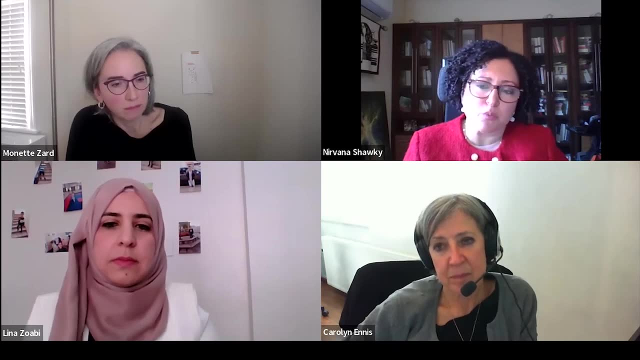 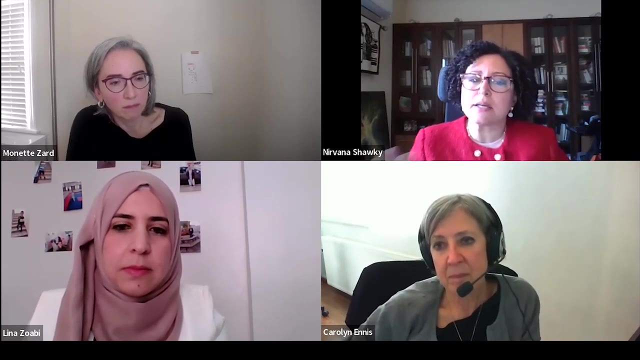 very eloquently, But I think that, looking at how can we effectively- I mean include, I mean refugee, I mean women and men, of course, in the policymaking processes that affect their livelihoods? I think that there are two key approaches that we try to really advocate for. 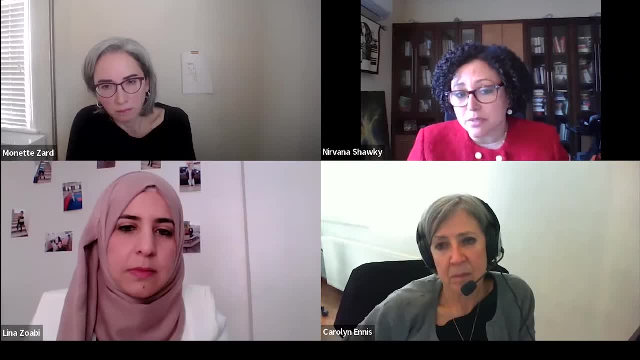 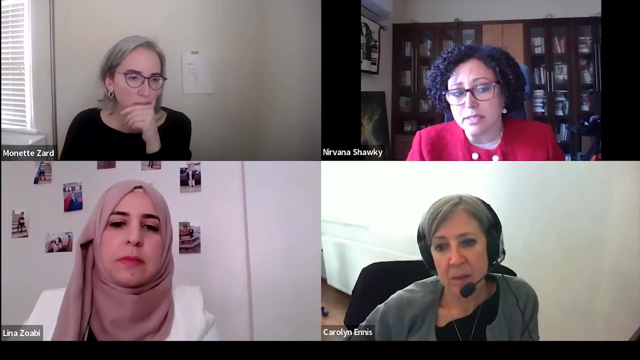 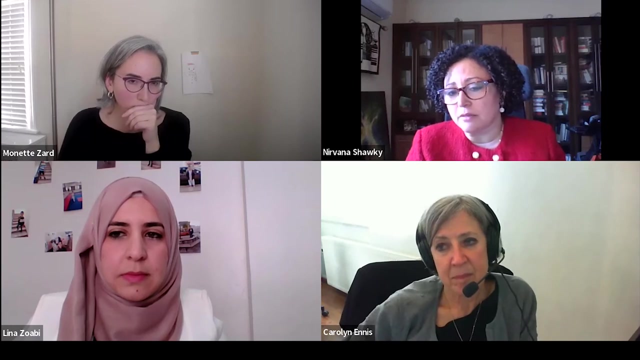 I mean. the first one is actually to- I mean to call for an investment, a further investment in supporting local capacities, including local women's leadership, through sharing and supporting capacity. that is, strengthening of- I mean national and local, I mean NGOs. I think this is really important and key to ensure that they are best equipped to engage meaningfully and effectively in the humanitarian response. 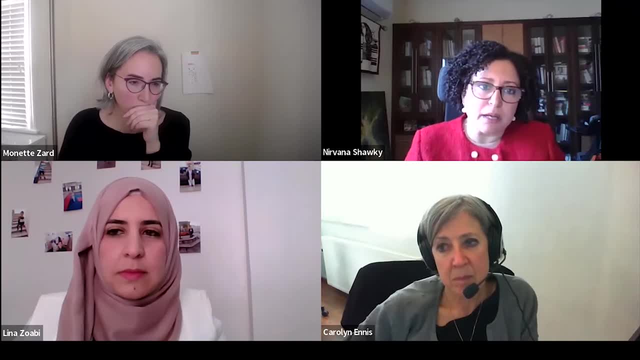 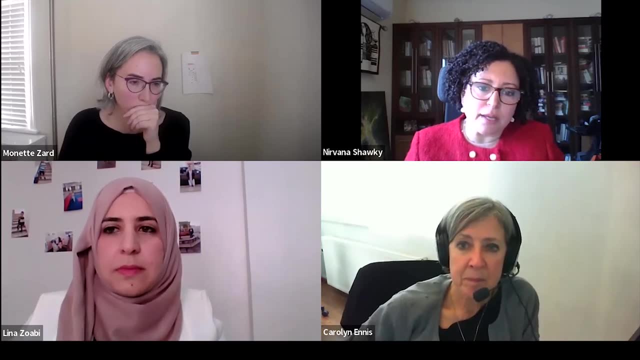 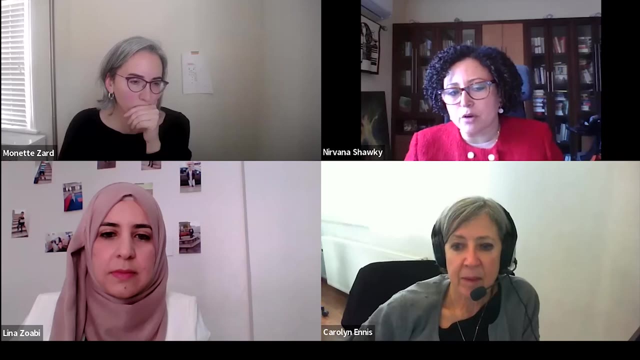 And this actually really opens the door for multiple initiatives. Multiple I mean avenues for engagement, I mean on a livelihood front. and of course, the national and local partners have power. in relation to the local context and with the deep knowledge of the communities, they are often better placed to advocate- and to I mean respond for the needs. 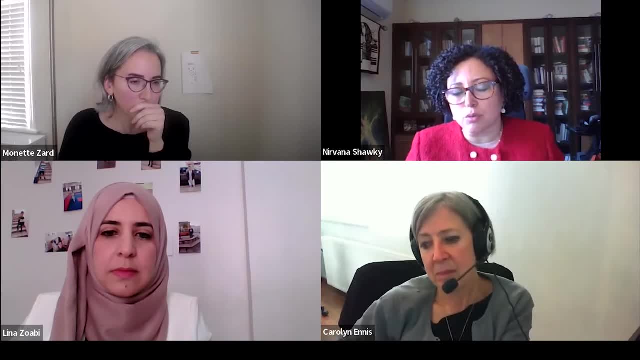 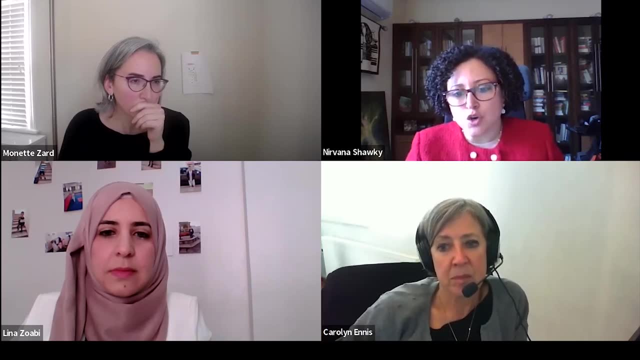 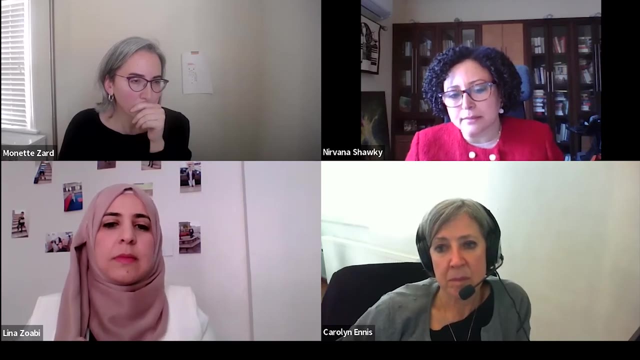 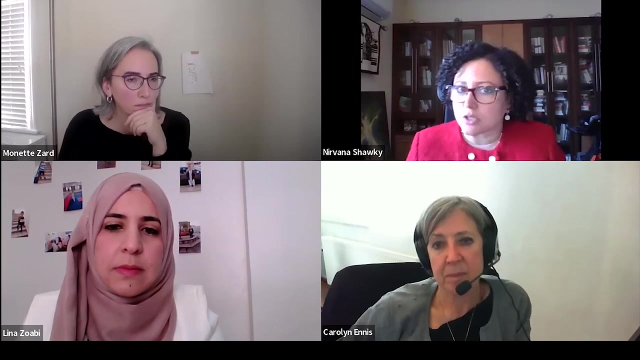 The other piece is actually really related to the prioritization Of national and local NGOs and organizations in the participation of the advocacy and letting them really lead the agenda, because I think that's one of the key pieces in advocating, for example, with national governments, as the Jordanian government, as the Turkish government, as the Lebanese governments. 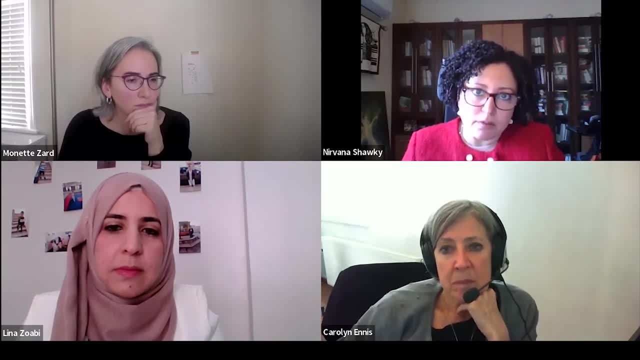 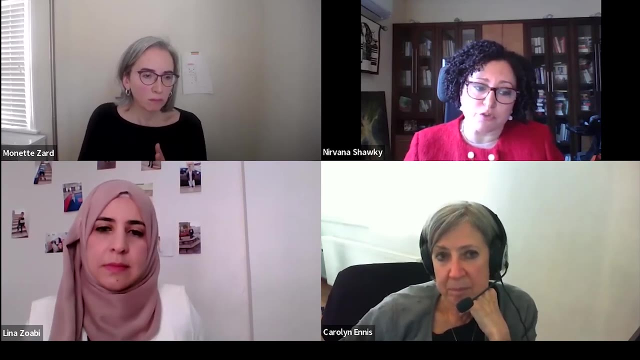 I mean there is so much. I mean different weight that the local organizations bring when they are advocating for bettering Inclusion for refugees. and better inclusion for I mean fair and open opportunities for ensuring, I mean livelihoods for refugees. 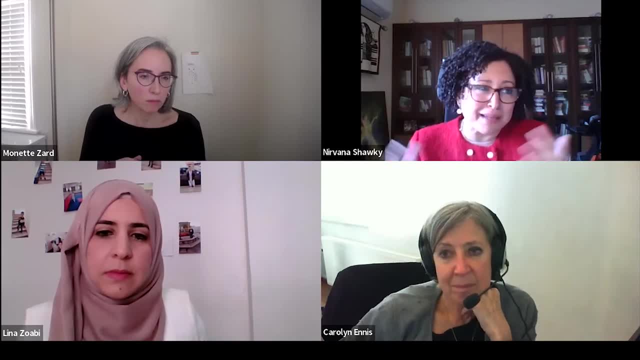 And I think that one of the key pieces- and I know that I mean again, I'm advocating to, I mean to my peers- is that I mean what we need to really be calling for is the donors to ensure that the national and the local organizations can really engage in influencing structures and seeking the change at the level of policy. 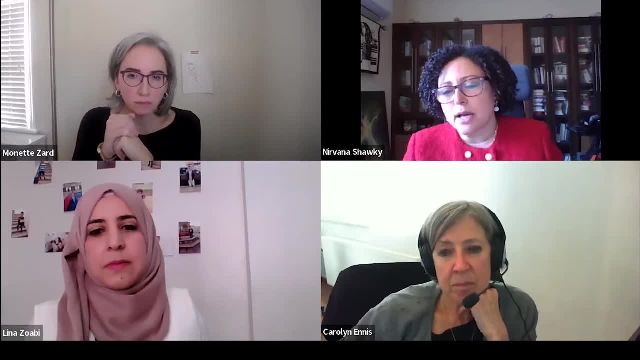 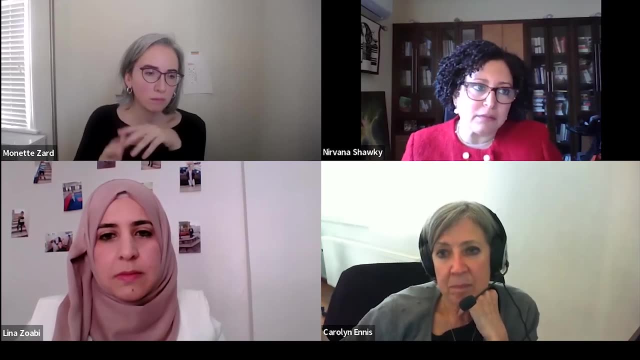 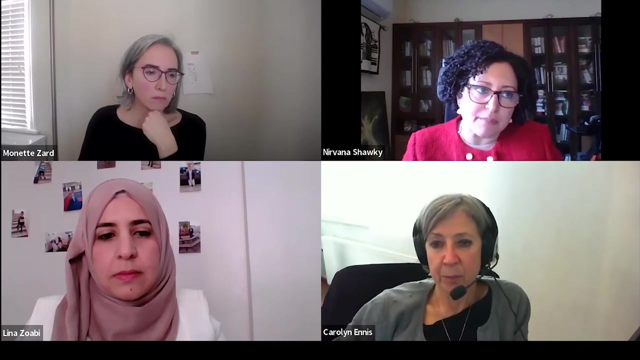 And legal frameworks or social norms to ensure that both the most urgent needs and the long-lasting challenges are addressed. And we have great examples from the last- I mean decade- working on the Syria crisis, where really the national and the local- I mean partners have led a lot of the efforts for better integration and for better- actually I mean working conditions for Syrian refugees. 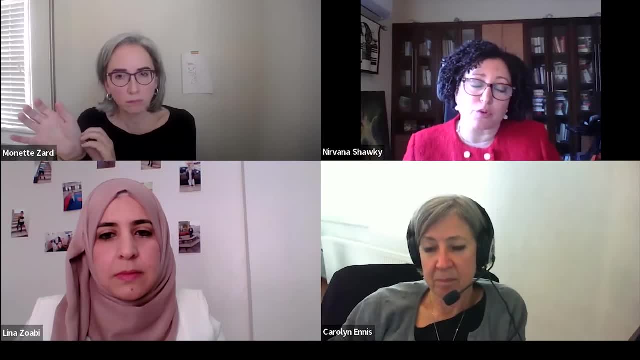 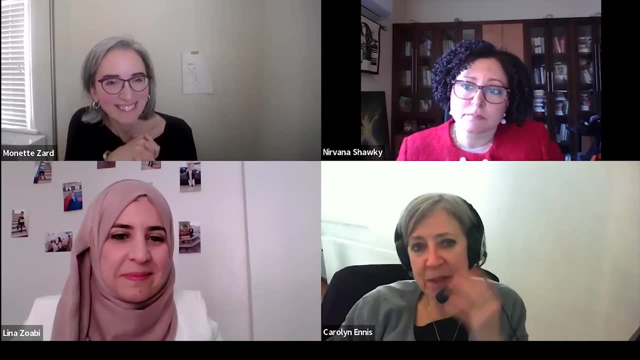 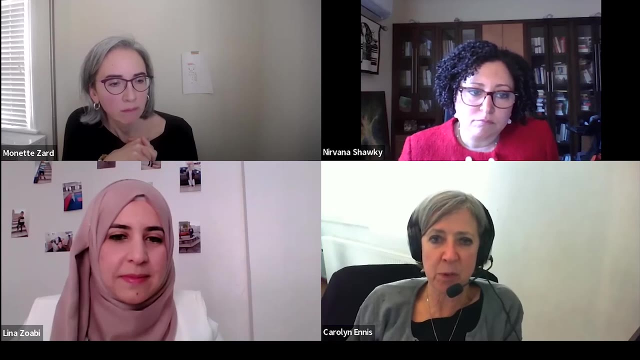 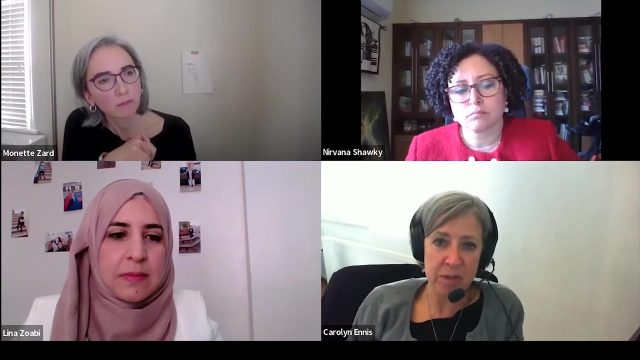 And I think that this is really, I think, the recipe for success: moving forward. Thank you, Carolyn. Yeah, I'm sorry to jump back in again, but I think the work that we do with the UN country team supporting the government in its work towards the 2030 goals and the strategic development goals, leaving no one behind and the right to decent work and including refugees in this type of initiative- 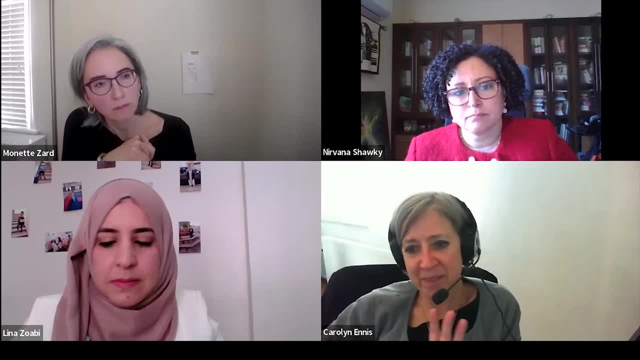 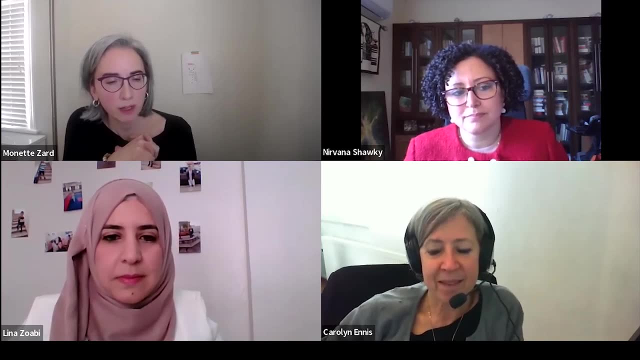 I think that's also critical at the very, very strategic level. That was just my additional comment. Thank you, Absolutely Great. Well, in fact, we have an extensive question coming up on refugee inclusion, but I'm going to leave that to last. 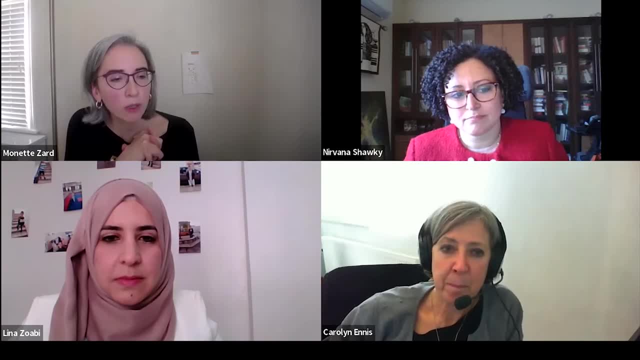 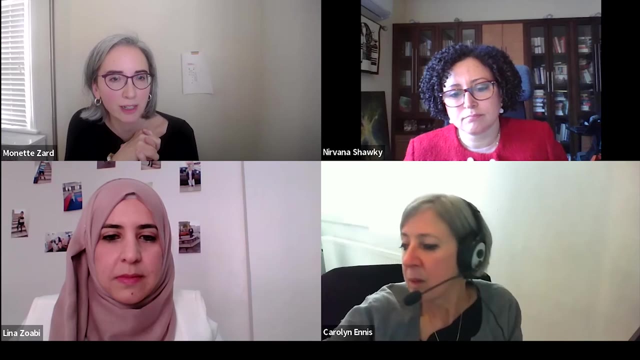 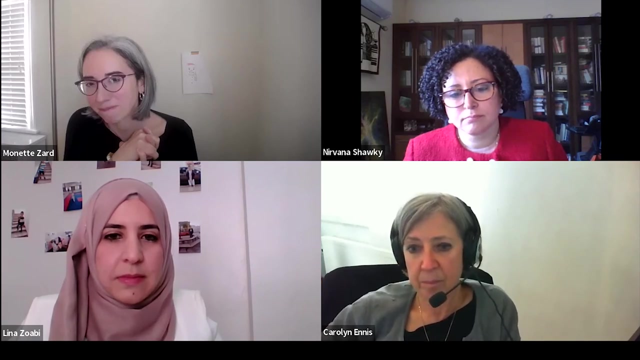 There is a quite specific question here about how would the panelists assess the contribution of cash for work projects for building Syrian women's resilience? Do, in any of your experience, stretch to the cash for work project? Okay, So maybe that's one thing we can take. 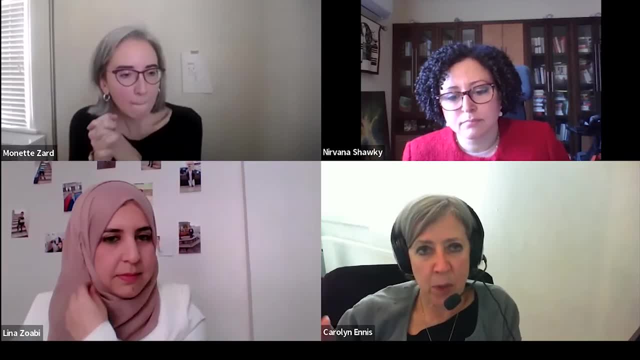 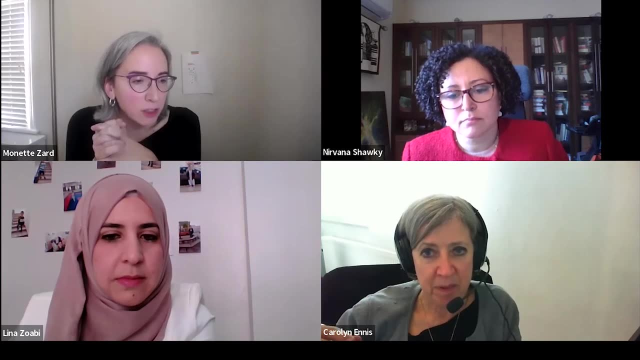 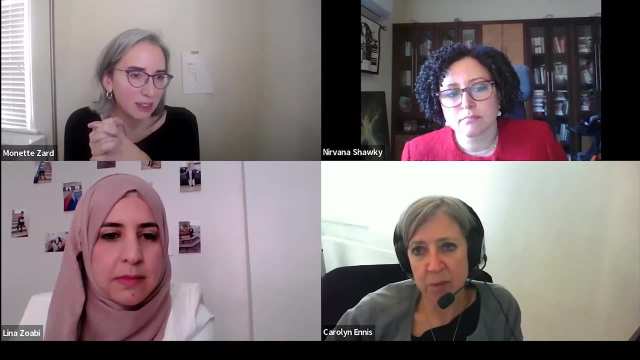 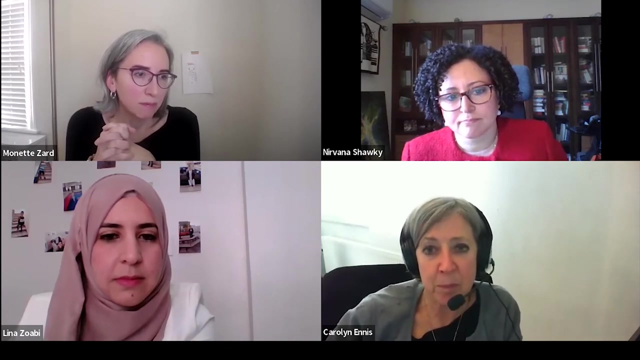 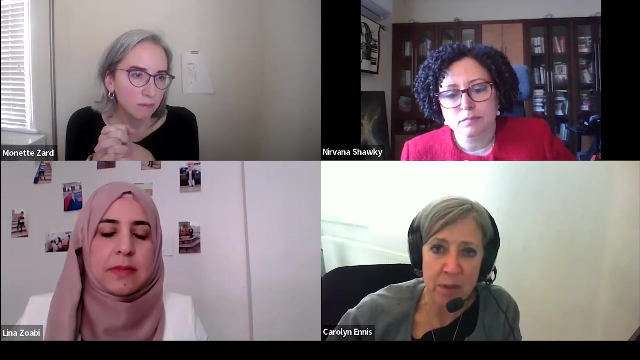 Oh, Carolyn, The question: is it cash for work or is it cash assistance? It's very different. I interpret this as being cash for work Because multi-purpose cash is a fantastic way for everyone across the board to support Refugees, and cash for work is just one component of cash-based interventions, which are really effective ways of protecting vulnerable women and even supporting them while they get trained so that they can get a job. 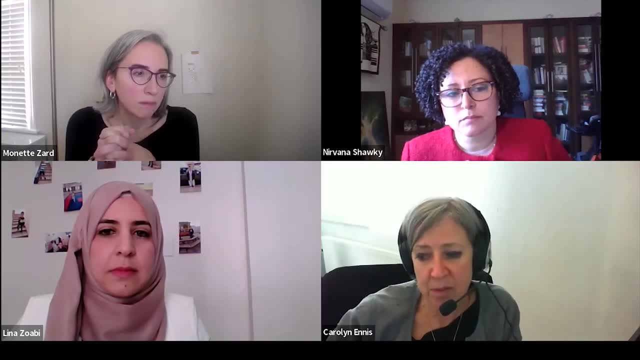 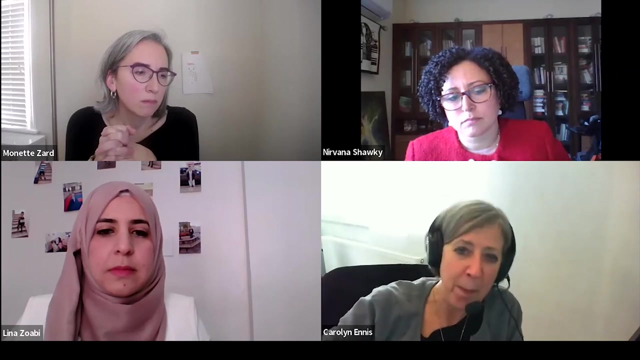 So just to emphasize, I think, the importance of cash-based assistance we've dispersed to 32,000 families per month every year. We dispersed over 5 million US dollars in February alone And it's a really important aspect of protection. and cash for work is one part of the full range of cash-based interventions which are carried out by our partners at many, many different levels. 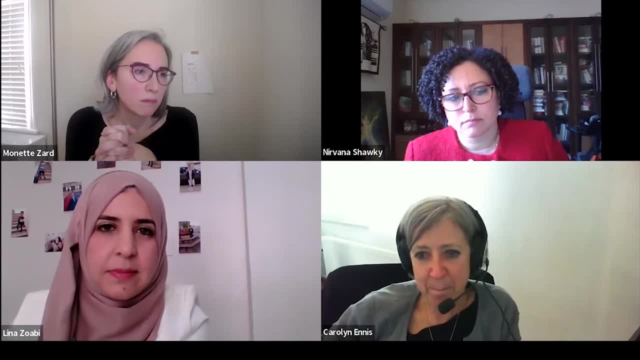 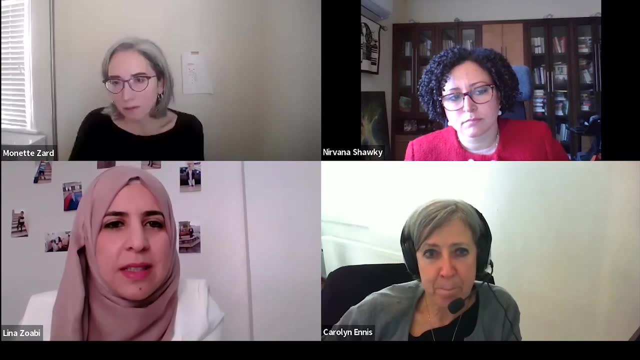 So just wanted to emphasize that I think Monata that was one of the strategies that is training the. I think Monata that was one of the strategies that is training the. I think Monata that was one of the strategies that is training the. 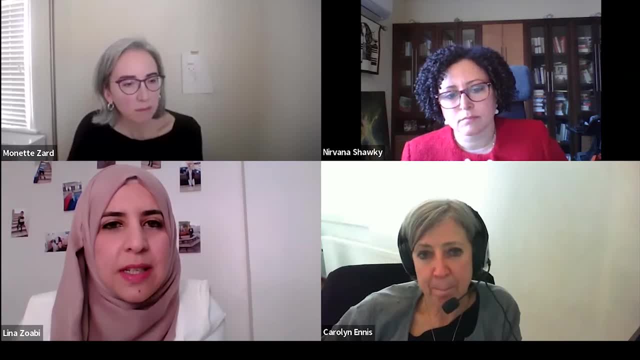 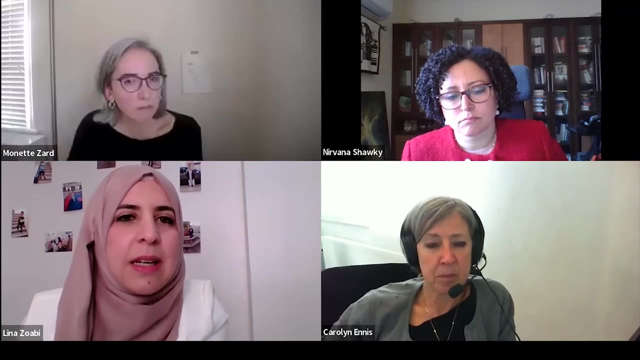 Participants as women, for example, on different skills that the program targeted, then seeing the project's proposals and what is successful and useful for them and then giving them the money, waiting for a few months to see how is it successful or not. 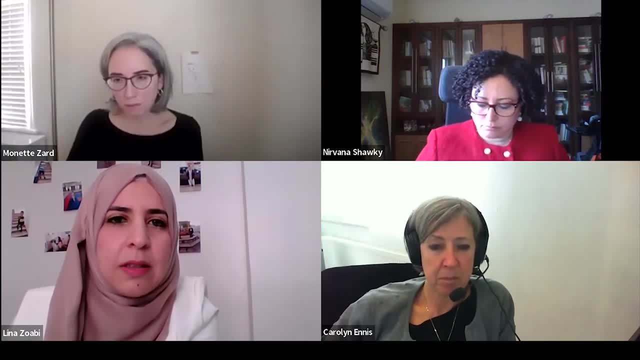 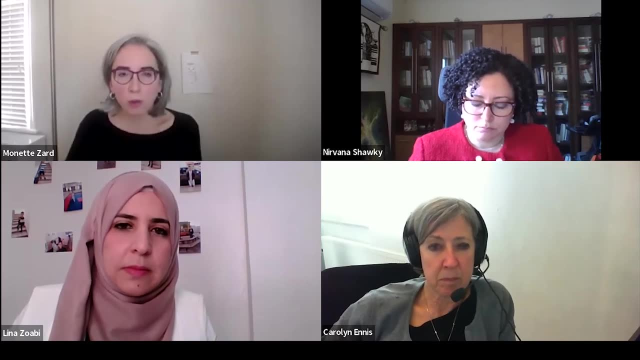 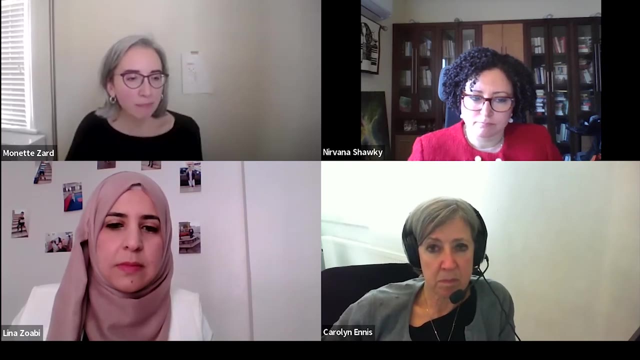 I think this is one of the assessments for that. So I wanted to come to a question that we've been talking around quite a bit, but it's posed by someone in our audience, so they want to hear more. Can you please share with us your experience and thoughts on women's perceptions on work? 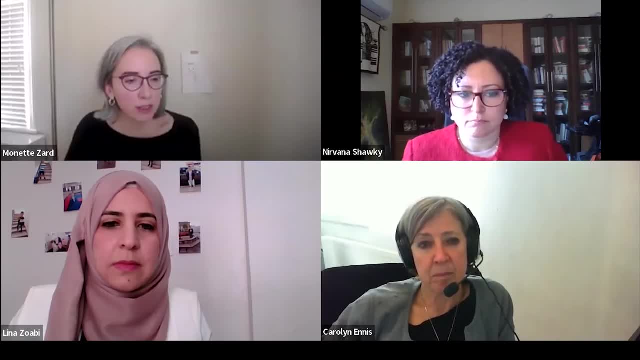 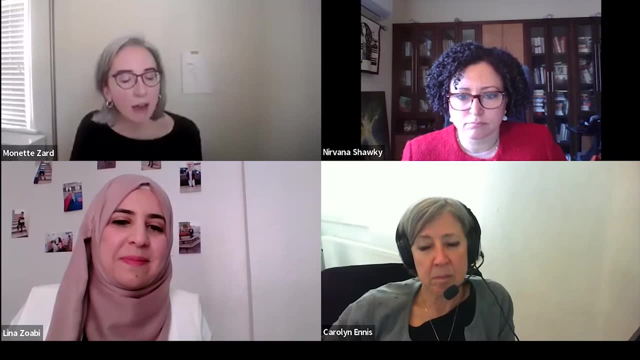 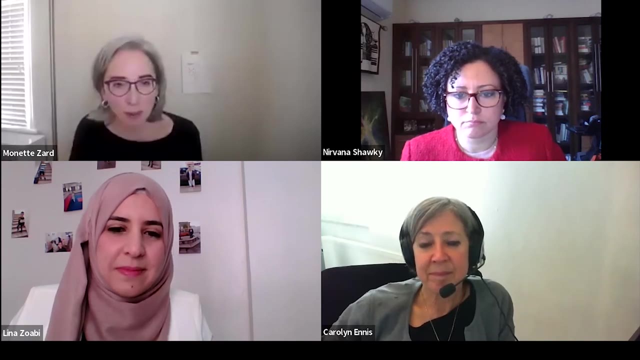 What trends or common education and skills Syrian women possessed before the crisis compared to what they've acquired after the crisis? And then, finally, how do you engage women in your programming, Which I think we've been talking about quite a bit, but another opportunity perhaps for you all to reflect on how important this is and what you're doing. 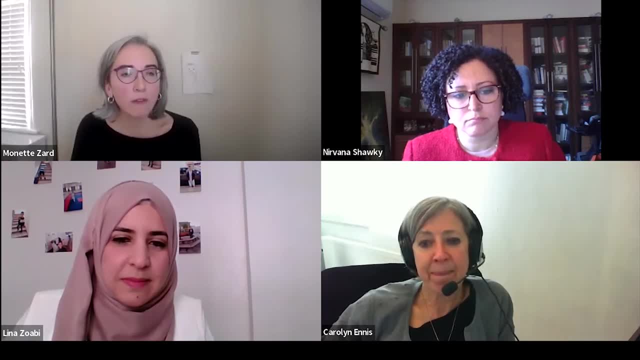 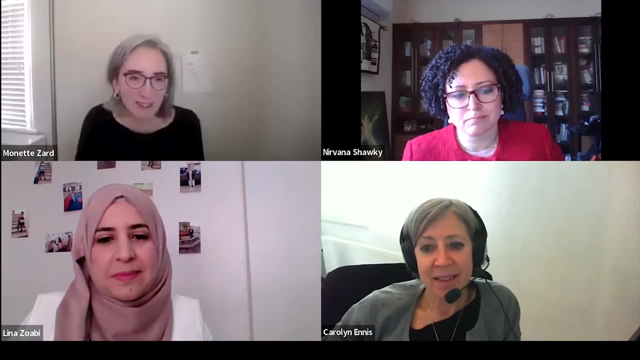 How do you engage women in your programming in response to the evolving needs and addressing some of these barriers? So happy to take whoever would like to go first. Carolyn, I love it. Go for it, Yeah, and please make me wait, you know. 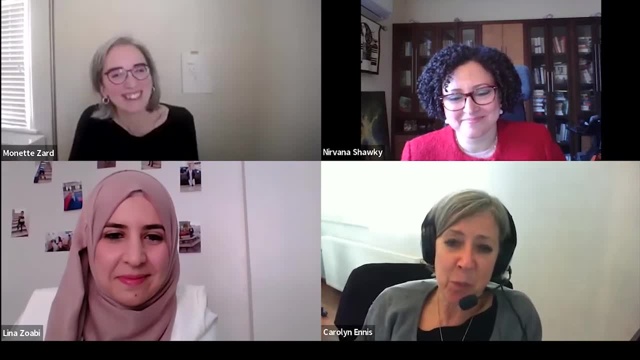 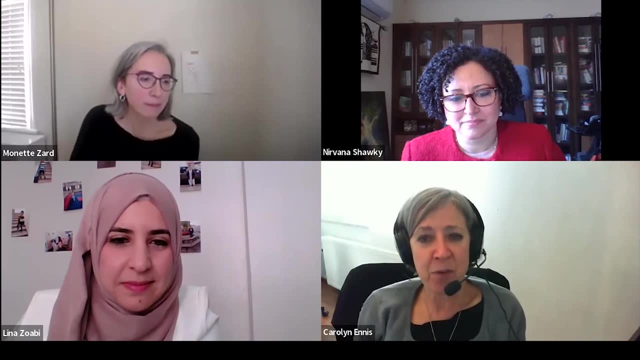 But I'm really excited about this because we have so many different ways of involving women in our programming And every year, every quarter, we have focus group discussions with men, women, girls, boys. We have a series of questions and we ask them for feedback. 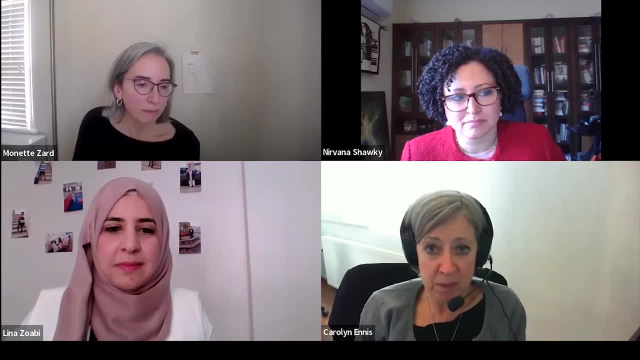 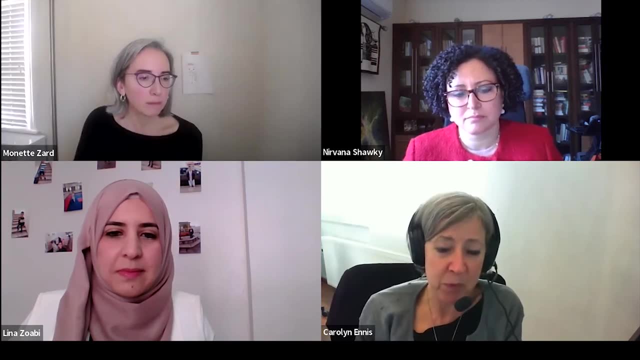 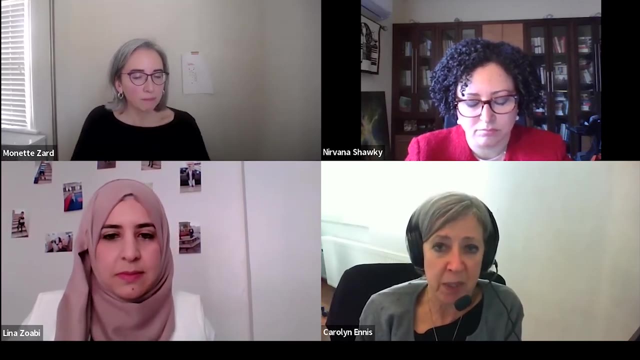 So we don't plan anything without going to the community, the community outreach centers, and listening to what- well, in this case, what women want. We try to get feedback from everyone, but it's absolutely core- And I think it's part of the IASC guidelines- to all of us working in a humanitarian setting. 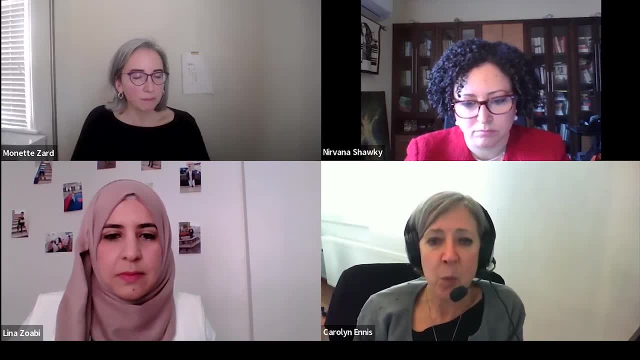 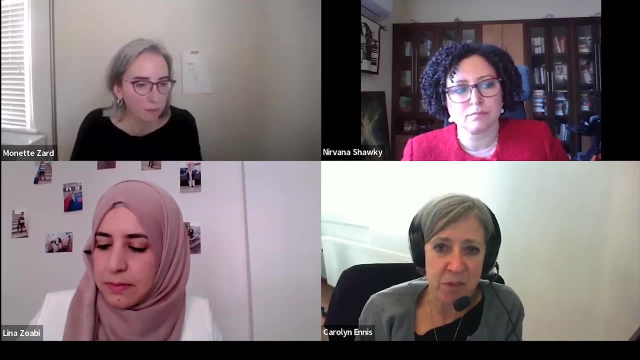 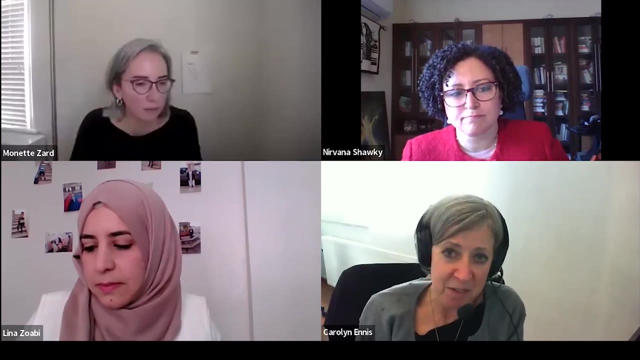 That all of our, Our programs are based on planning with the community and it's built into our results based framework and our planning, which is based on the strategic development goals, among others, and listening to the refugees, And very often we the answers we get are not the answers that we've been expecting. 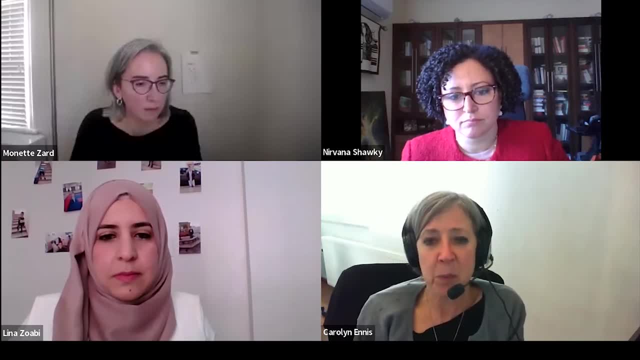 And so we sit down, we discuss, we ask women what they want and then we build our programming around what refugees want and how much money we have, of course. And very often we get feedback from you know, the community, the organization, from the women that we have and how much money we have, of course. 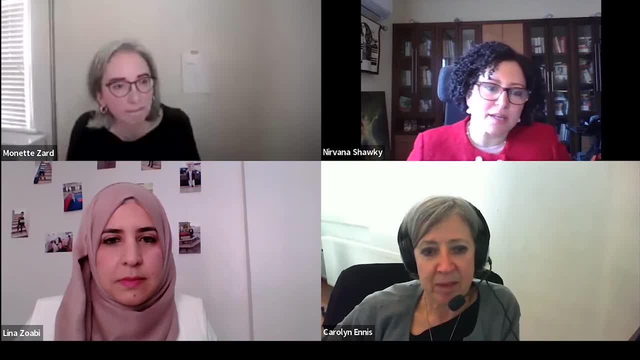 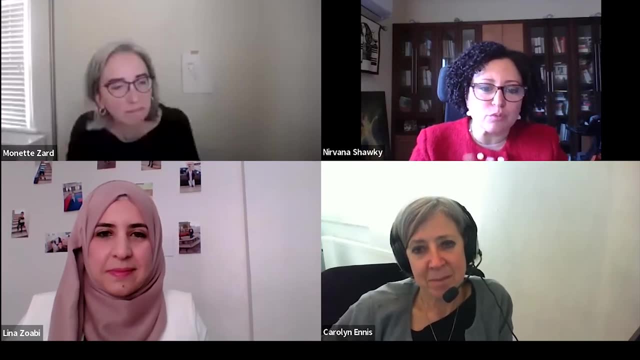 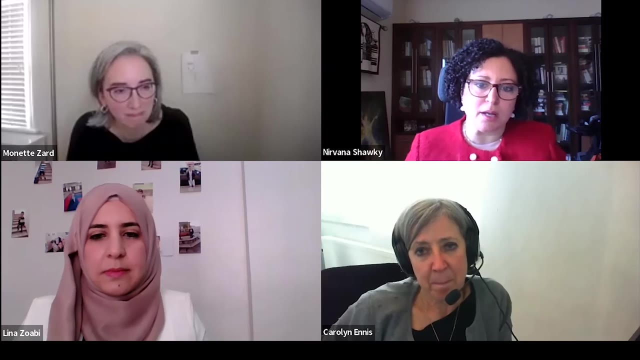 So we try to build a framework that we've been expecting. So we try to build a framework that we've been expecting. Yes, I mean thank you. I mean this is, this is really a big question, And I think that it requires actually, I mean, a workshop on its on its own to really, I mean look at, I mean, women's perception to work and how it has actually evolved with, with, with the crisis. 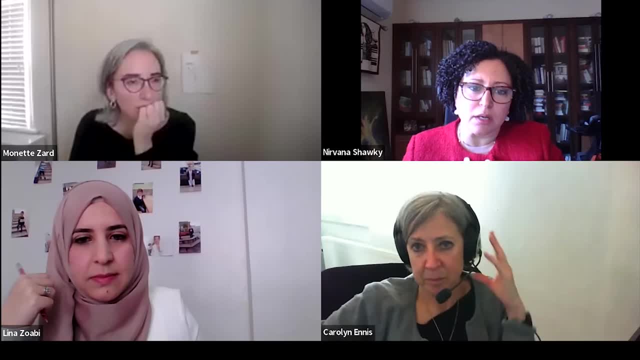 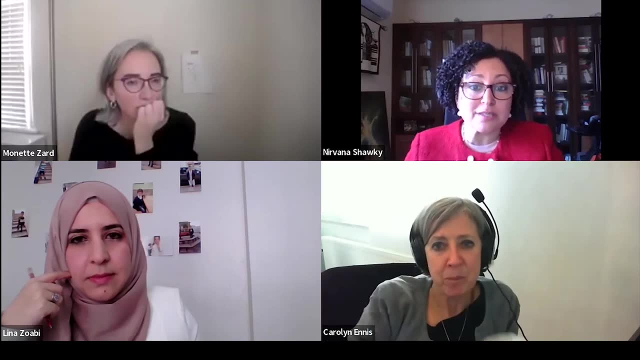 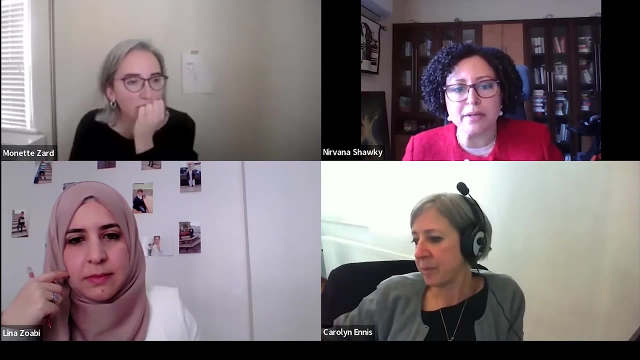 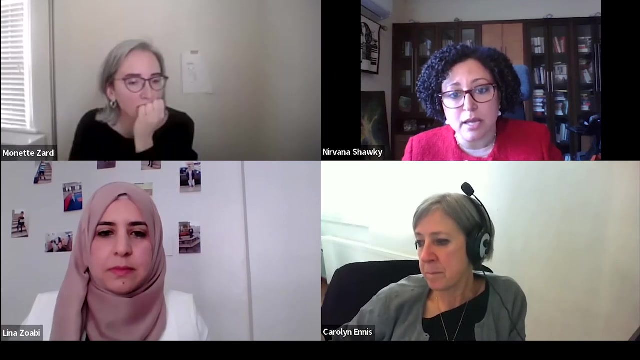 And I I mean I can actually give you one one example from our annual needs assessment in Jordan, where employment across genders and nationalities declined in 2021, even with the reopening of the Jordanian economy and the high COVID-19 vaccination rates. 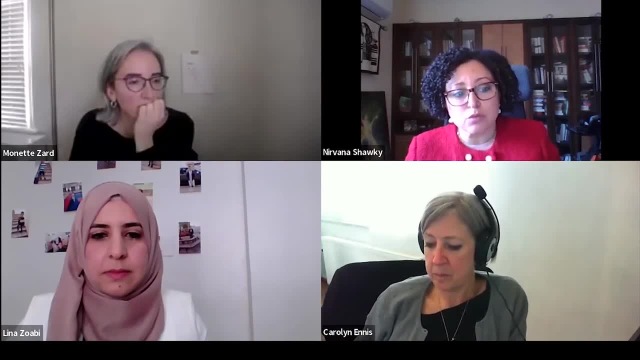 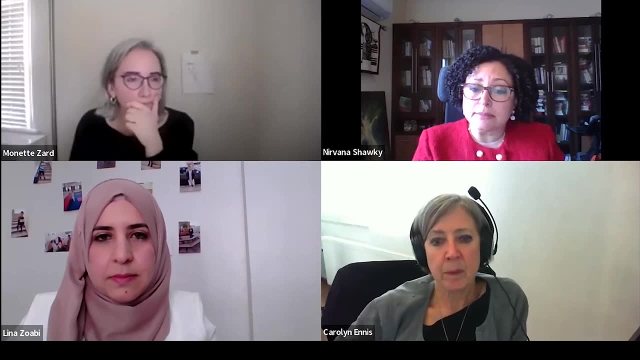 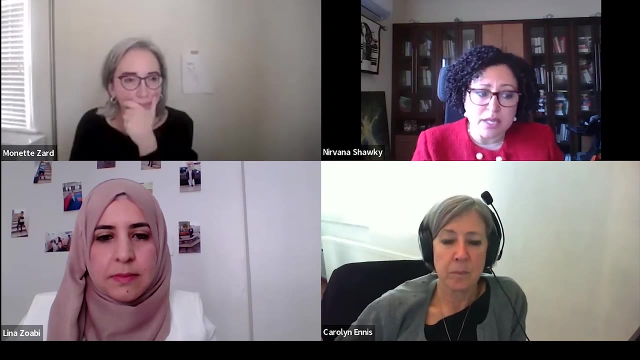 And only actually 41% of those interviewed had jobs, with Iraqi refugees bearing the brunt of unemployment, And among Syrian refugees, less than a quarter- around 22%- had work permits, as Caroline was saying, which is the lowest rate recorded in two years. 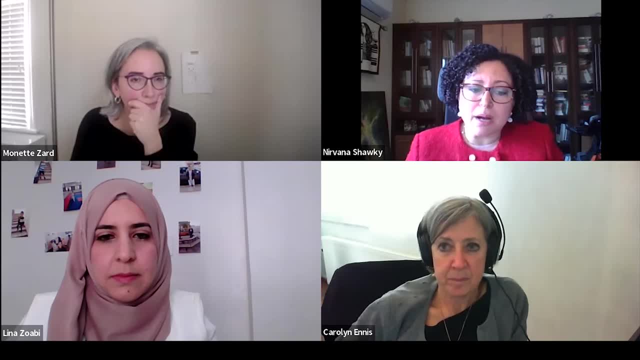 And unease among families is also heightened by the constant threat of homelessness, where more than half of the households surveyed said that they fear eviction And that fear has left them. They're feeling unsafe at home, And for many Syrian families living outside the camps, 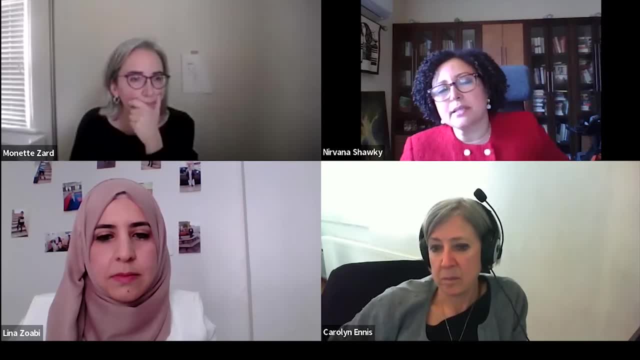 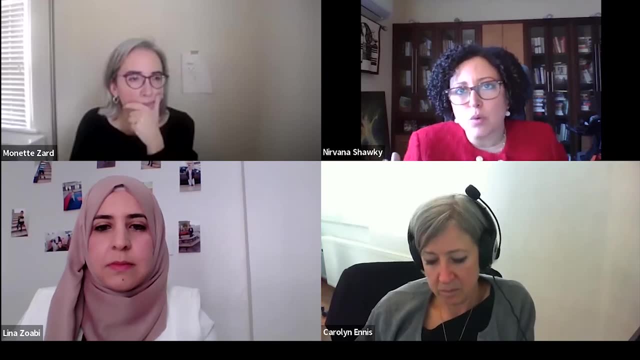 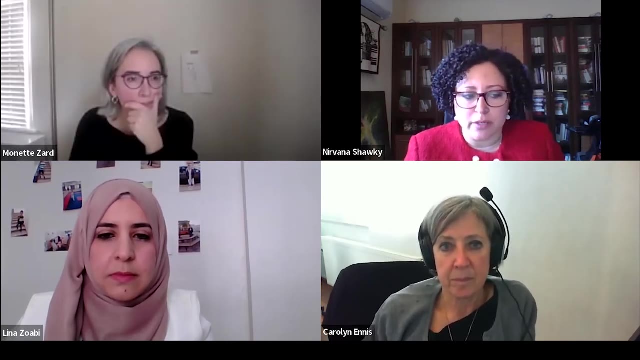 where rent constitutes over half their monthly income, if not more, leaving them with little food and other necessities, is what I mean. they managed to get by with their income after paying for rent, And I mean they have really been. I mean looking. 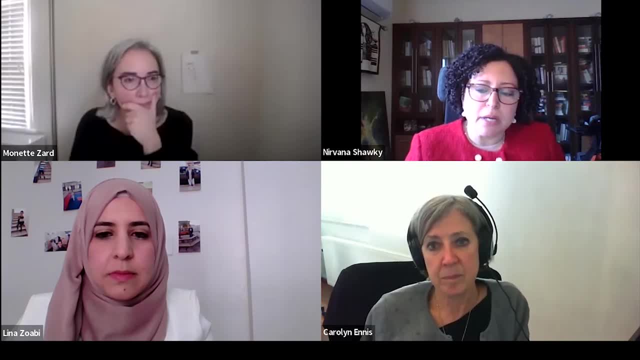 for different solutions, but the problem, I think, I think that the- I mean that- can be quoted in one of the quotes of the respondents for this annual assessment, which was saying, and I quote: without jobs or savings to fall back on. 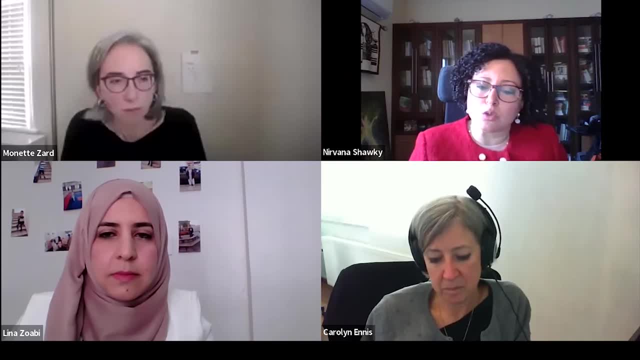 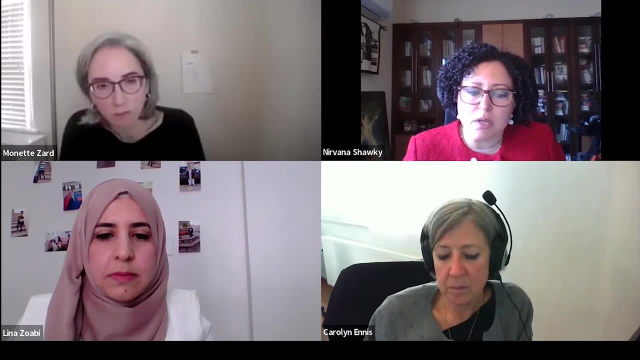 families live in perpetual fear of having their landlords turn them out or their water or electricity being cut off, And I think that this actually is a constant solution, is a constant problem That requires really- I mean again- a very, a very comprehensive approach to address it and not only to deal with it from one angle. 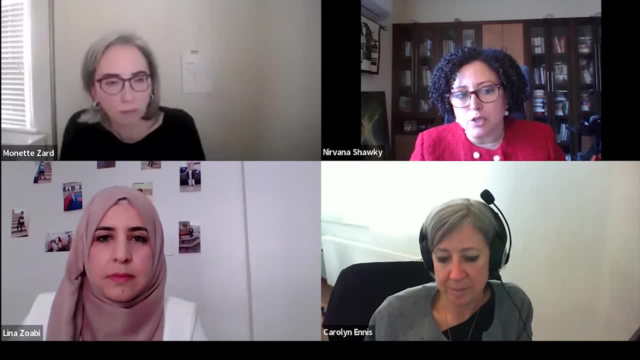 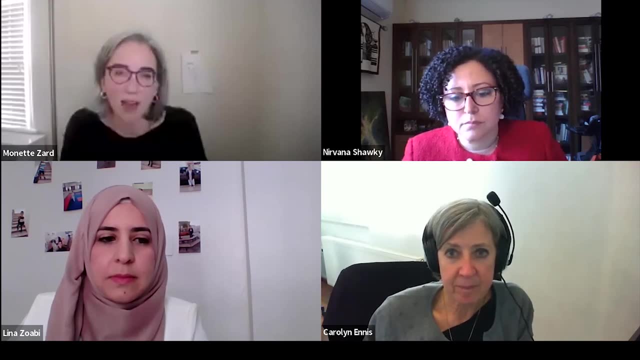 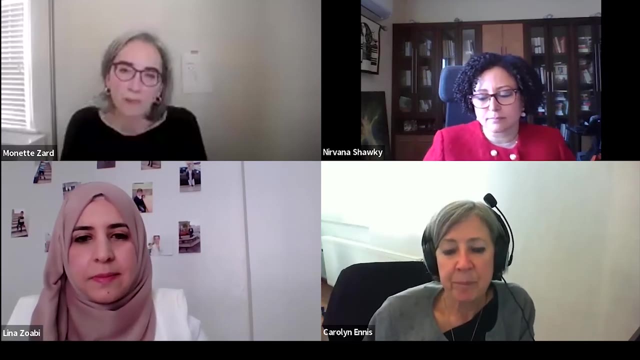 And this is what we try to do in CARE, I mean, as we engage in the Syrian crisis. Thank you, Thank you. So I'm conscious of time and we're coming up against, you know, the culmination of this conversation, but I'd like. 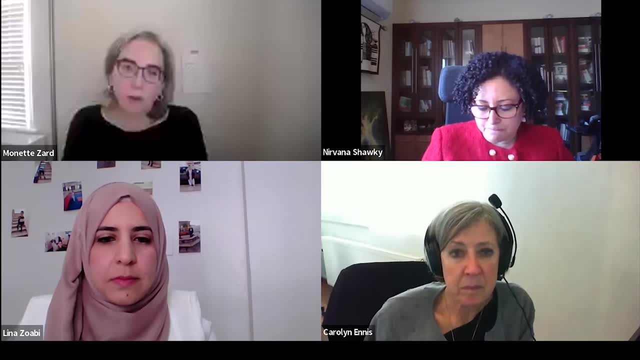 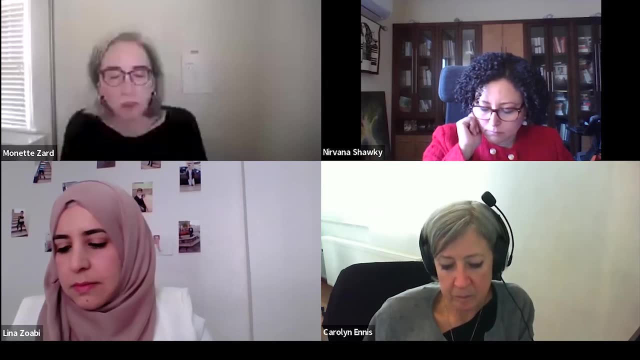 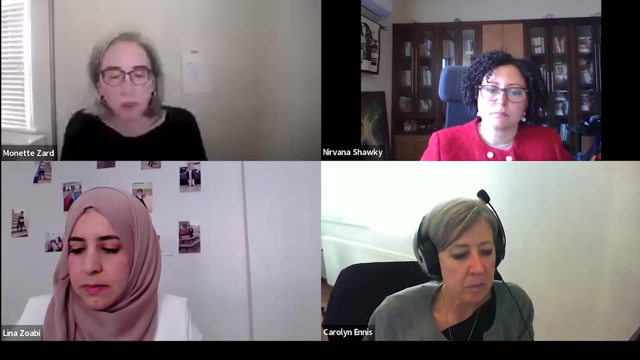 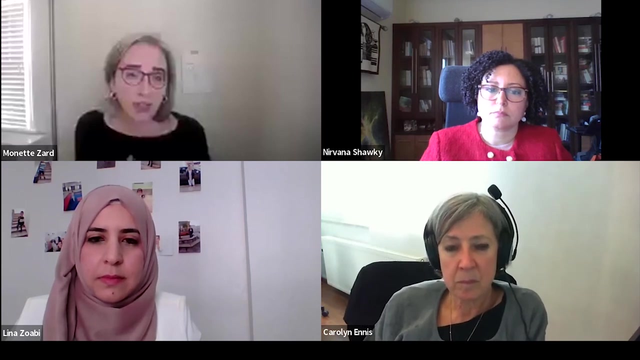 to throw you a question, which is- you know, we've heard some wonderful initiatives here and really comprehensive thinking about the scale of the problem, the needs and some really innovative strategies to tackle the need to involve more in the workforce. I'm conscious that today we're operating in the 11th year of a conflict. 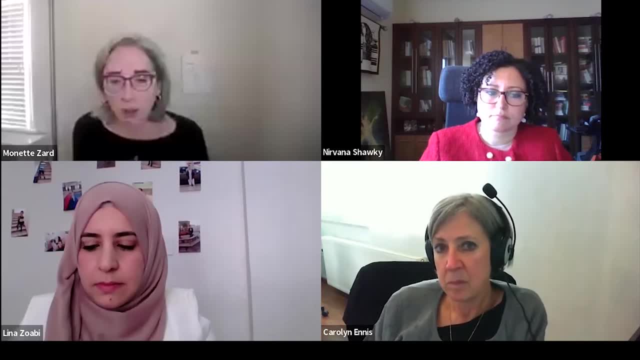 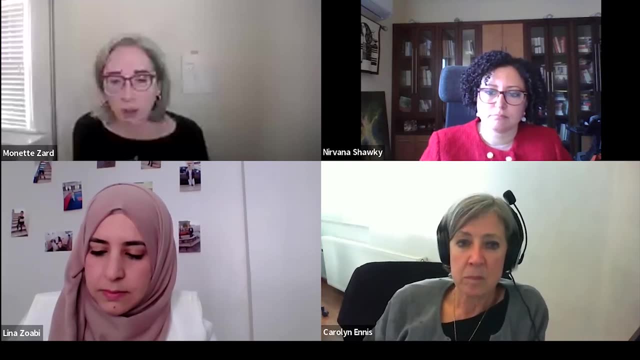 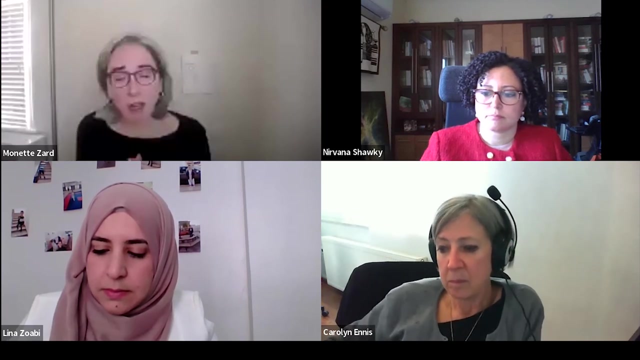 We know donors' attention And we also have Ukraine, which is certainly diverting potentially attention and fortunately also resources, although we hope not in the future- from this crisis. So I would like to ask you all if you had to convey, you know, one or two key messages to 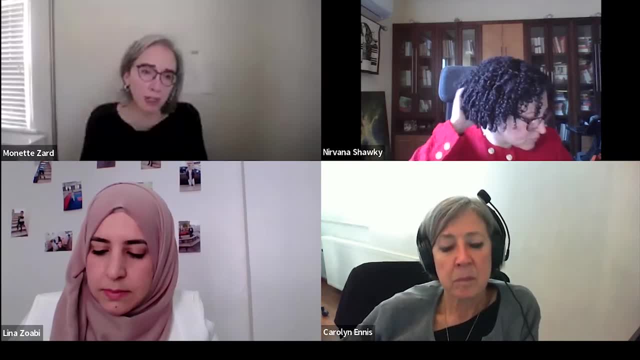 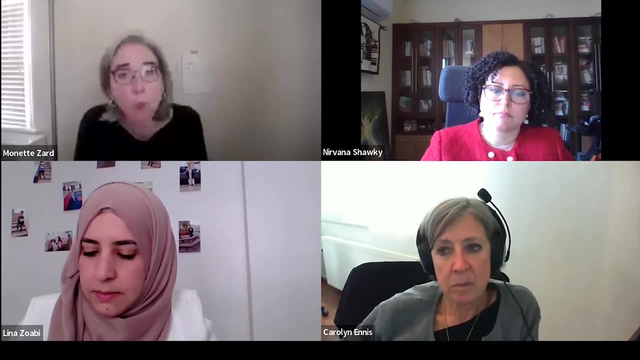 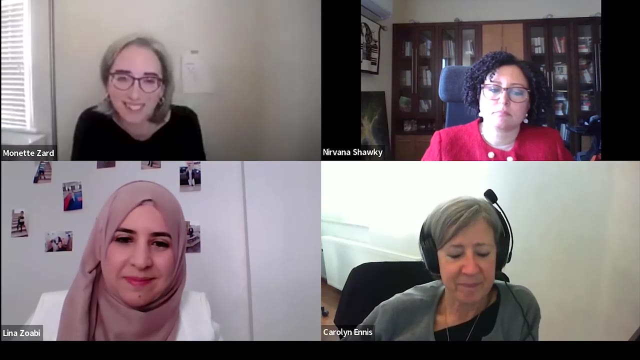 you know the international community and the donor community here- about how to address this crisis, How to capitalize on all of this important work and how to scale up this work. What would those messages be? And I might start with Lina, if you don't mind. 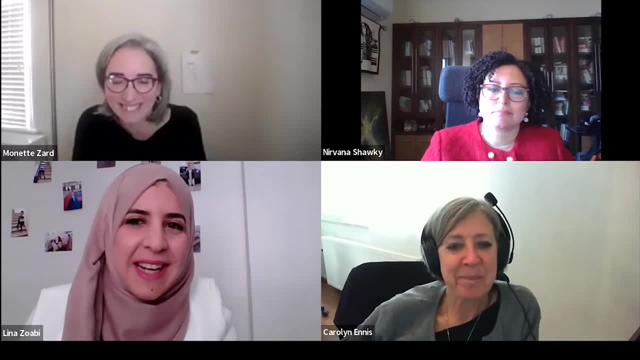 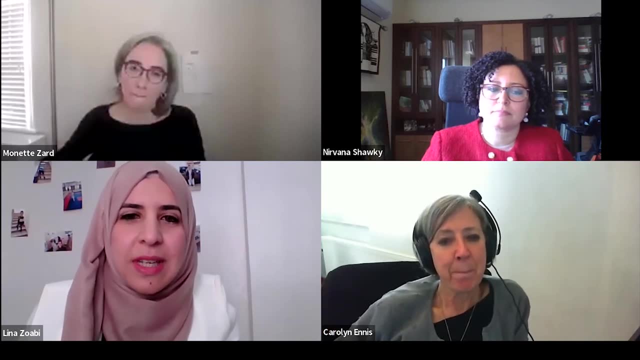 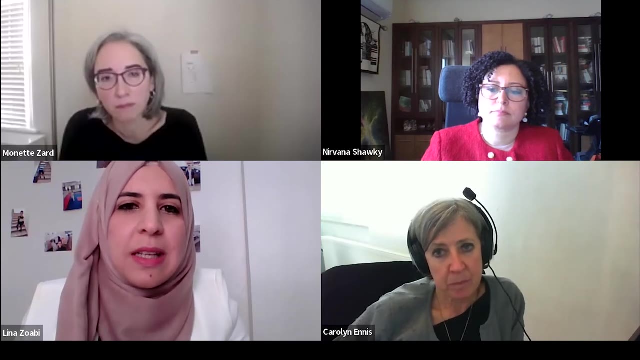 Do you feel ready to go first? That's okay. I hope nobody would go through the situations that most of the Syrians go through, starting from the displacement and the suffering that they go through, integration and getting adapted to a new environment. So the basic thing: to try to elevate some of the pressures that any human being can go through. 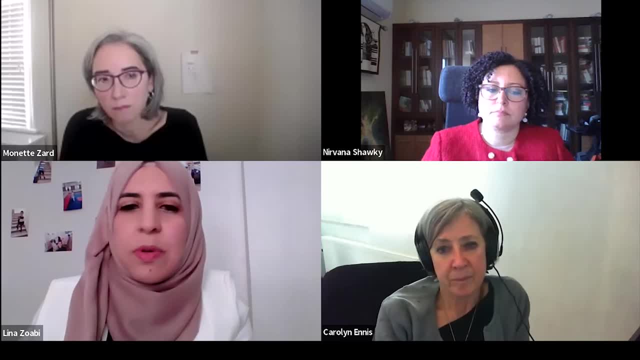 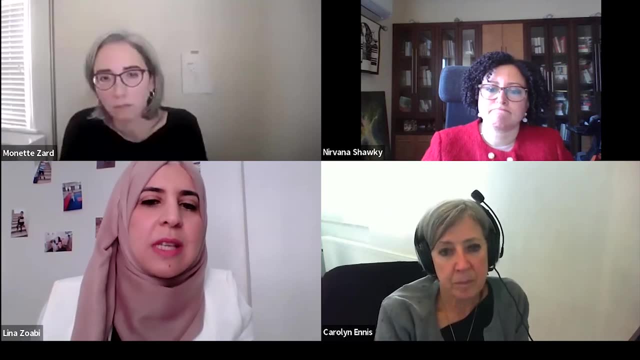 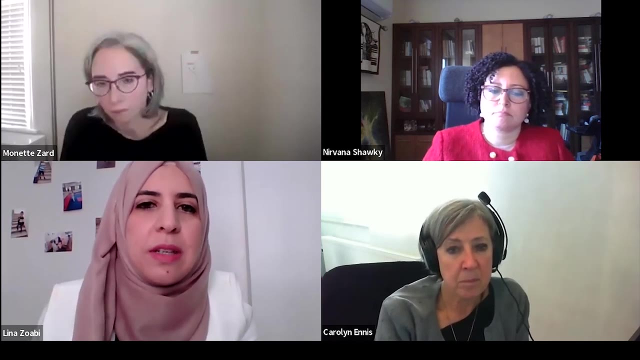 starting from the displacement, and try to support them, offer them the basic needs that any human being can need, And taking into consideration that some people need some special things for their survival. It's not a matter of just food and drink And drinking or shelter. 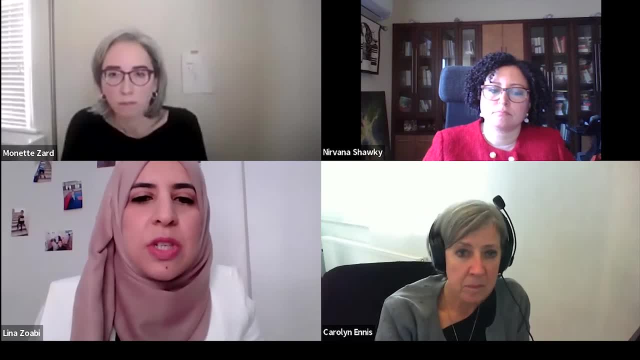 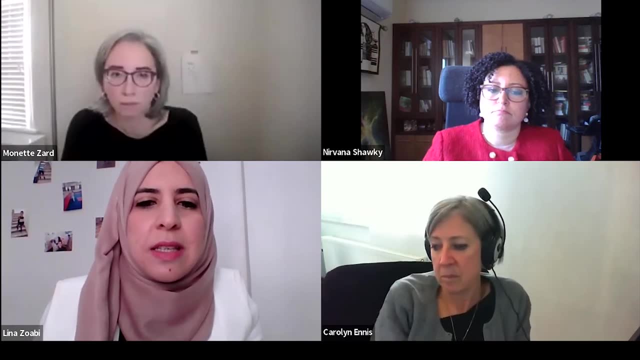 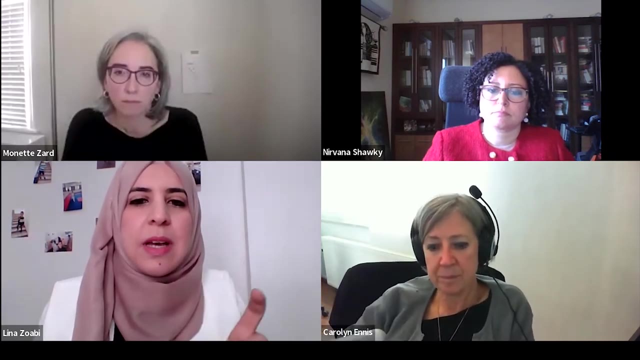 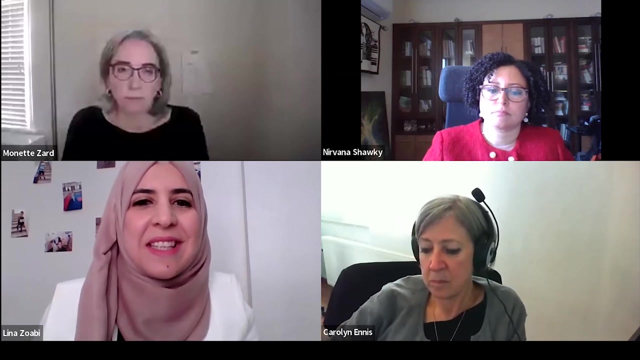 Then we should look to situations and see if it's short-term or long-term, As the Syrian crisis. basically, most of the organizations start to build short-term approaches or plans for the Syrian. However, as you can see, we're now in the 11th year and still discussing the Syrian matter. 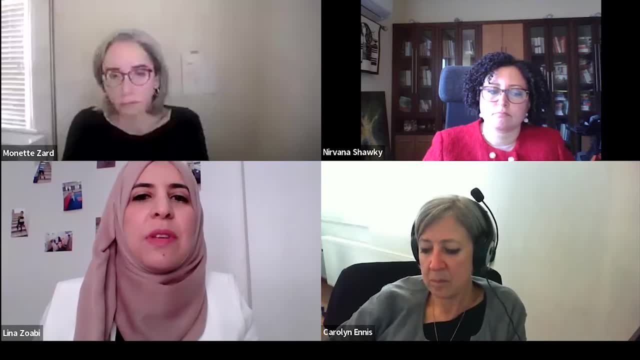 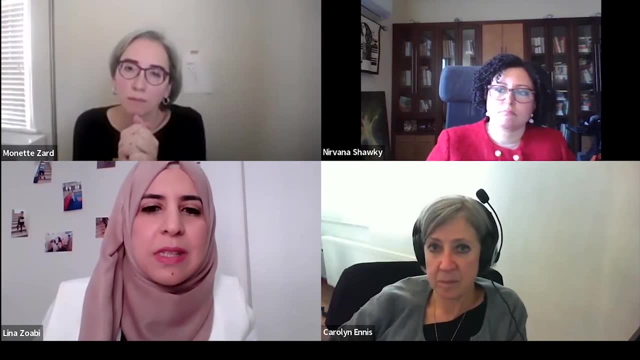 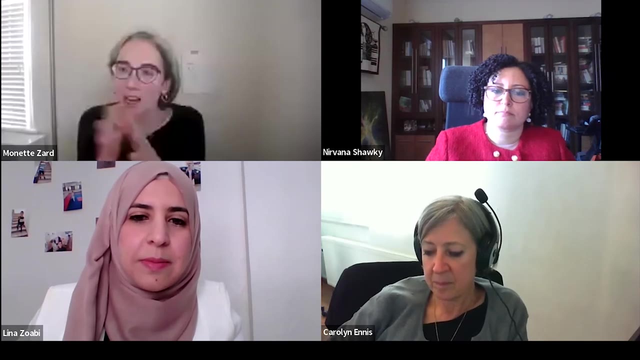 We should handle the situation from different perspectives. Is it the short, long and different needs that people, especially the displaced, need? Thank you, Lina. Thank you, Thank you for being concise, Carolyn. can I go to you next? 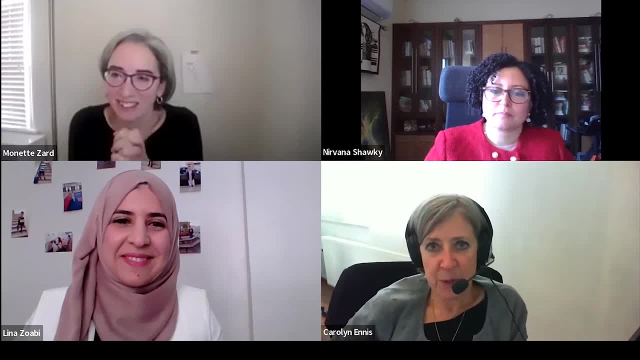 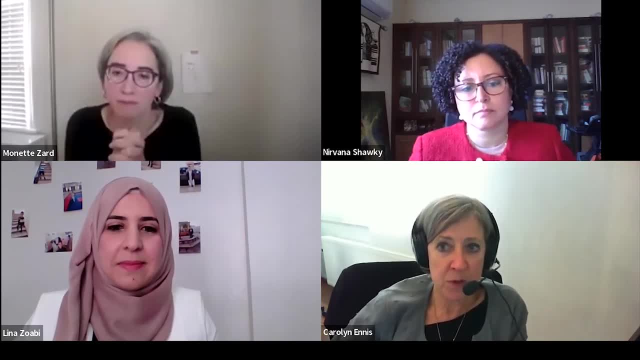 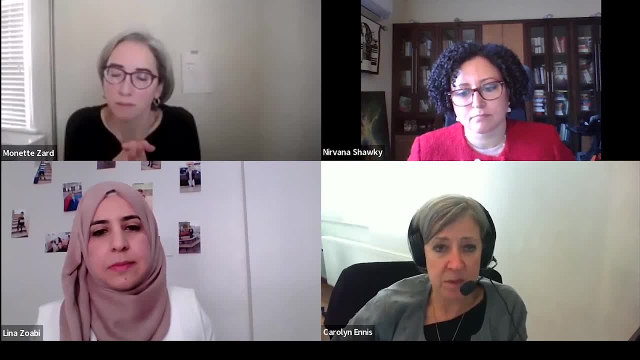 which are often the poorest countries, And I mean he's highlighted their needs in Afghanistan and Ethiopia for Ukrainians and, of course, in the MENA region, And we need really to try to plan in a sustainable, strategic way and work more closely. 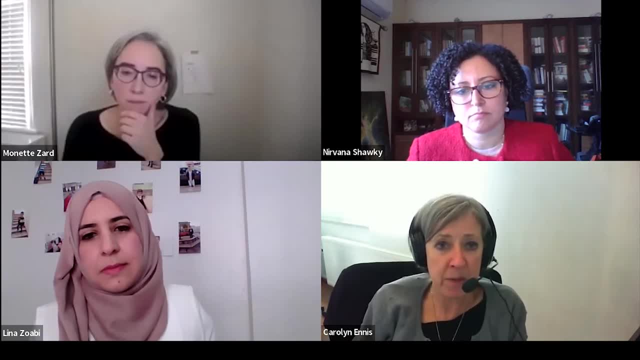 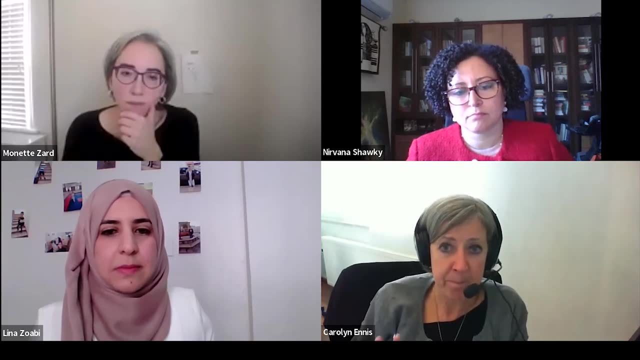 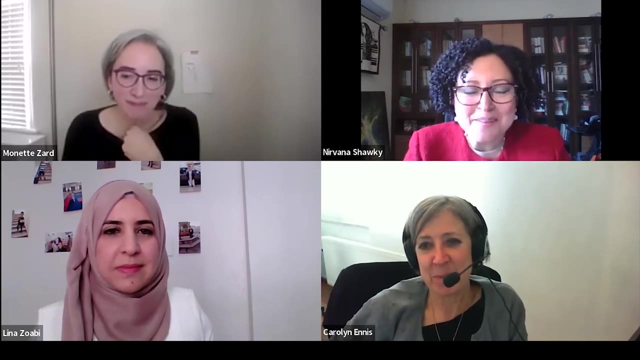 with the development actors for greater inclusion, to the benefit of both the host communities and the refugees who are being hosted. Thank you, Thank you, Carolyn Nirvana, you get the last word. I mean that's the hot seat, So I mean, and you said concise, so I'll try to be as concise as I can be. 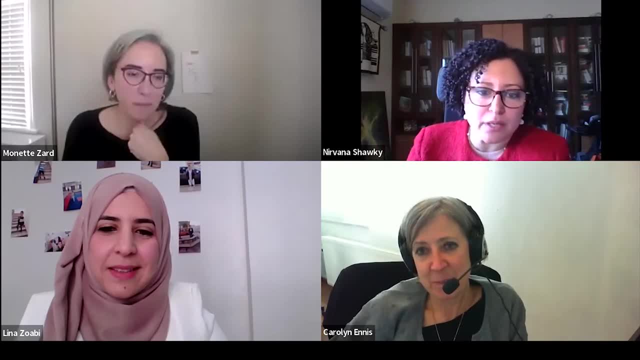 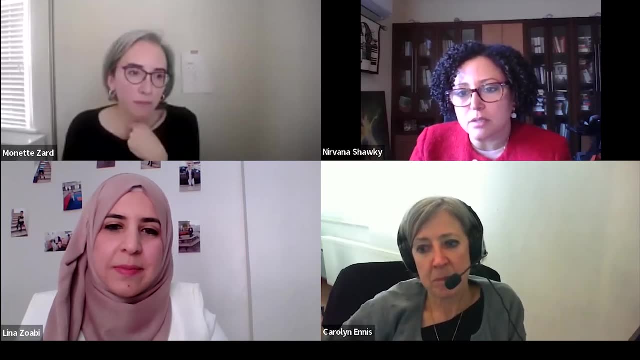 I think that I mean, in addition to echoing all- I mean all the esteemed panelists have highlighted and all the points that we, I mean raised in the discussion, I think that the ones that are not key message that is important to highlight is that as important as the Ukraine. 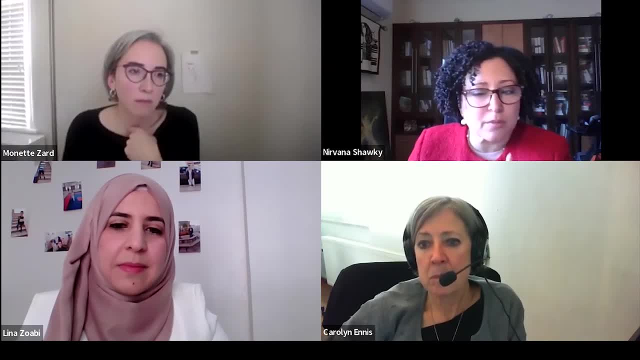 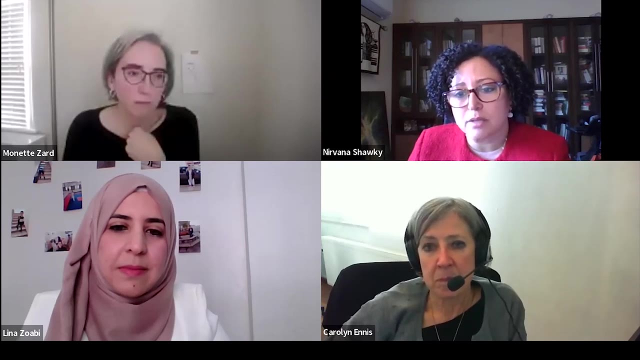 crisis it is. we should not forget the Syria crisis and the major humanitarian needs on the ground that are worsening rather than improving with time. I mean, with so many forgotten crises around the world, we need to keep our focus on the real needs on the ground in the various MENA countries. 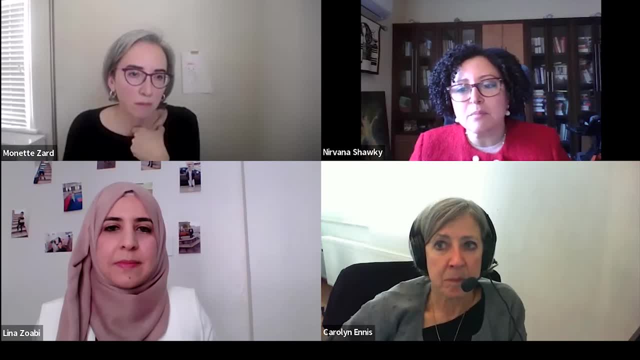 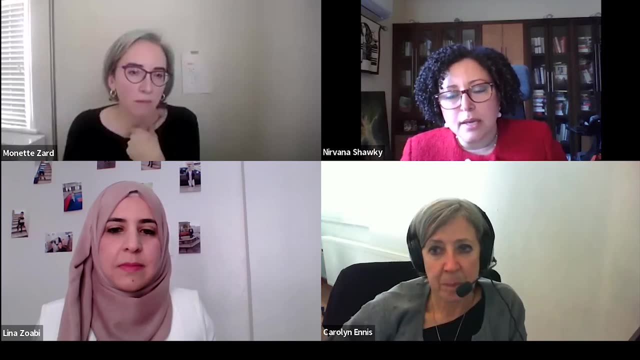 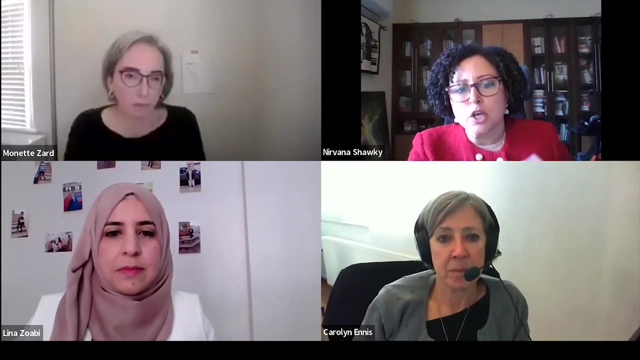 And I mean Yemen and Somalia, And I mean the number of crises are really countless And we really really need to ensure that the international community is does not actually focus its- I mean their attention to, I mean to- the Ukraine crisis on the cost of the other. 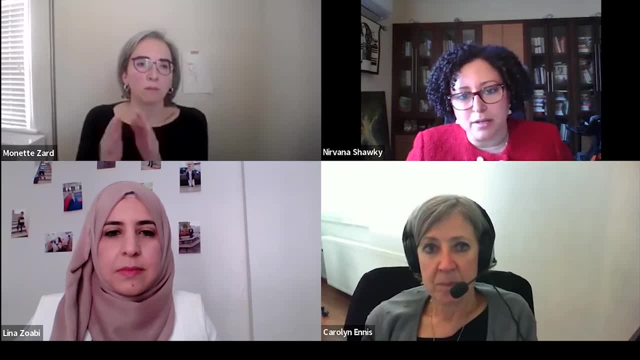 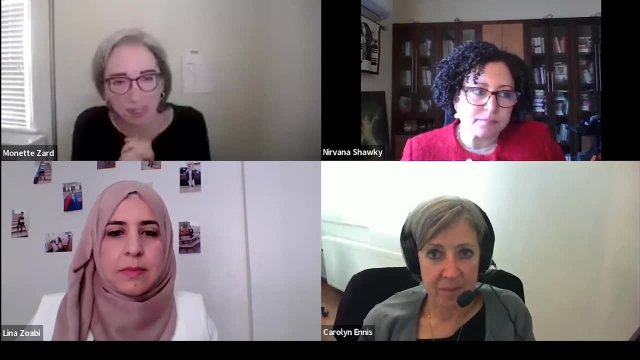 crises, which really the responses needs to be happening in parallel. Thank you, Thank you very much for the opportunity. Thank you, Thank you all for your insights today, For sharing with us just the real creativity, innovation and energy that you're bringing to. 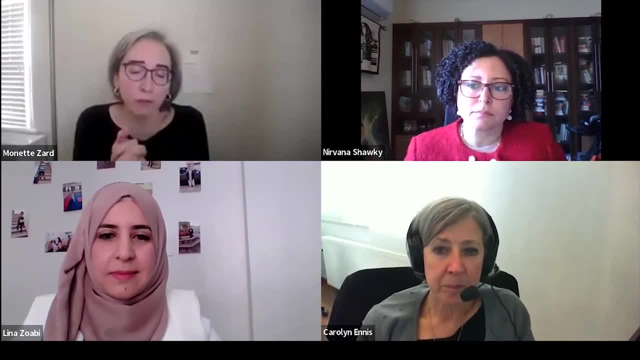 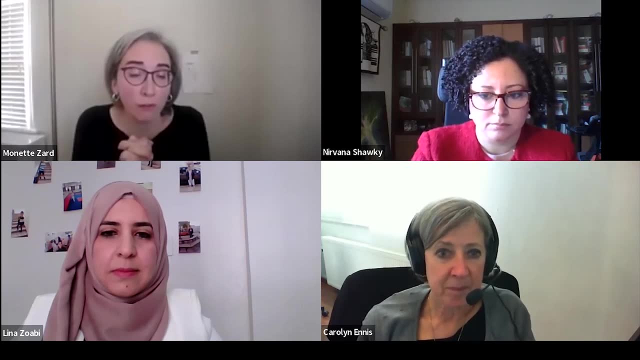 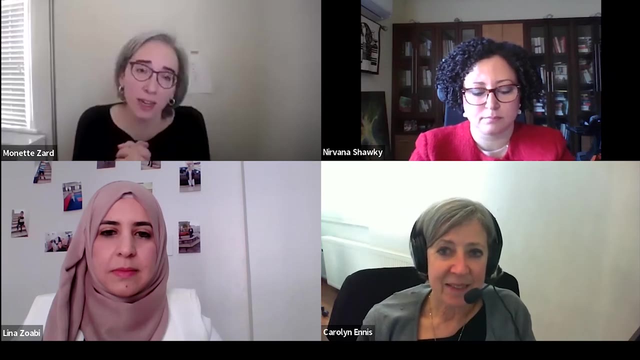 this work And for sharing with us the very real sort of challenges also that remain, And I'd like to thank our wonderful panel, I'd like to thank our wonderful audience for the great questions you posed. Please forgive me, as chair, if I didn't manage to get to all of them. 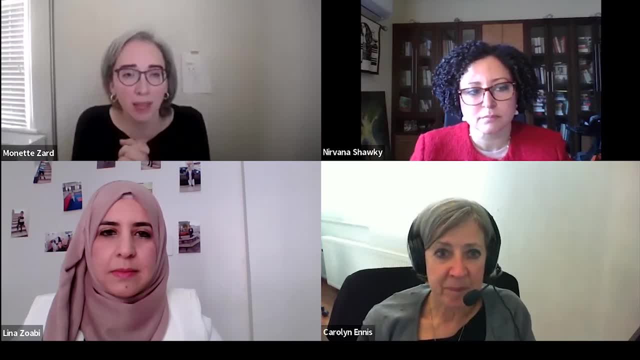 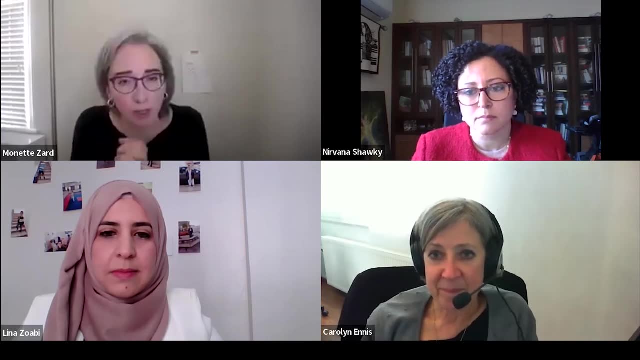 And finally, a big thank you to both CARE and the Amman Global Center team for all the work you've done. Thank you so much for joining us today And thank you so much for hosting and convening this conversation today. I'm sure the conversation will continue. In the meantime, take care everyone And thank you so much for joining us today. Bye. 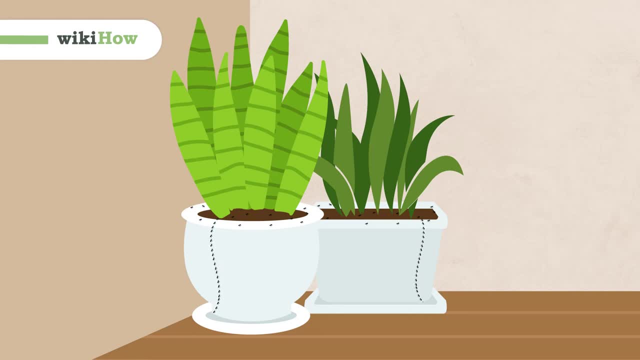 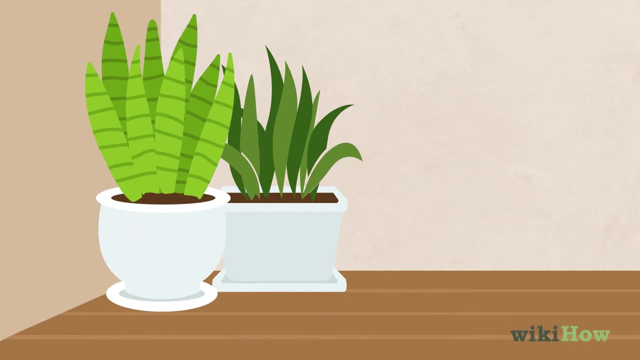 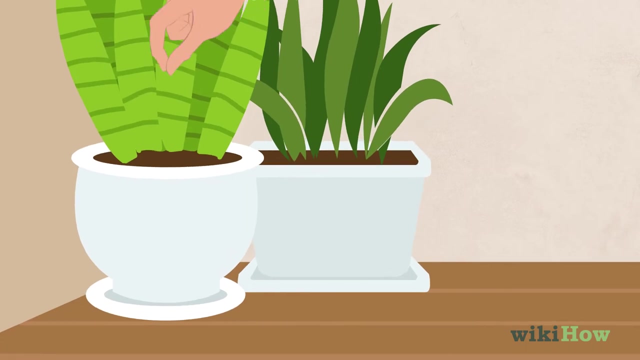 Ants usually aren't harmful to potted plants, but you can still remove them by placing bait traps on the floor around your plants. Replace the bait traps every few days until you don't see ants anymore. Another solution is to cover the topsoil of your plants with a thin layer. 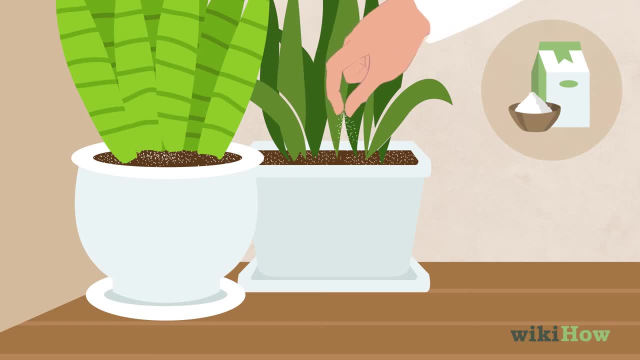 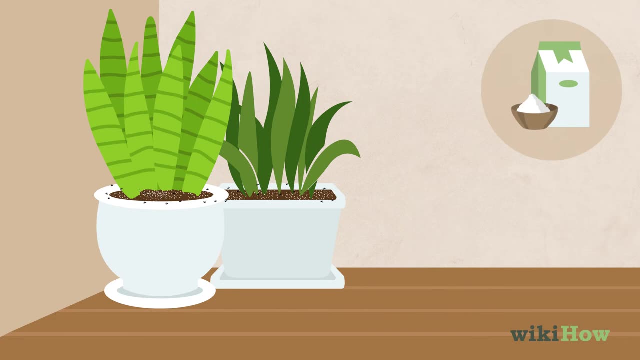 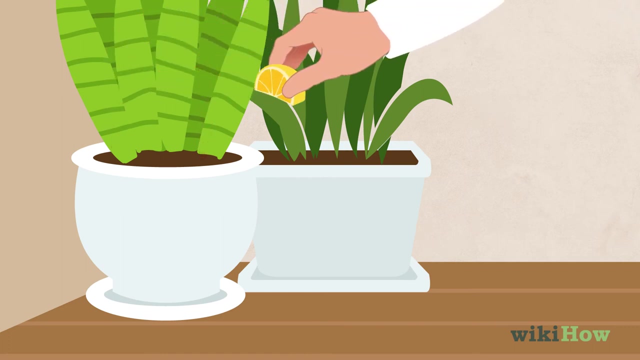 of diatomaceous earth, which is an organic insecticide. This will kill any ants on your houseplants and it's completely plant-safe To make an ant repellent. squeeze some citrus juice over your plants. Ants don't like the smell of citrus, so the citrus juice will help keep them. 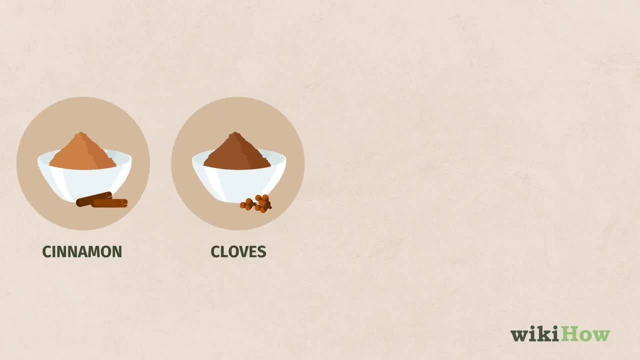 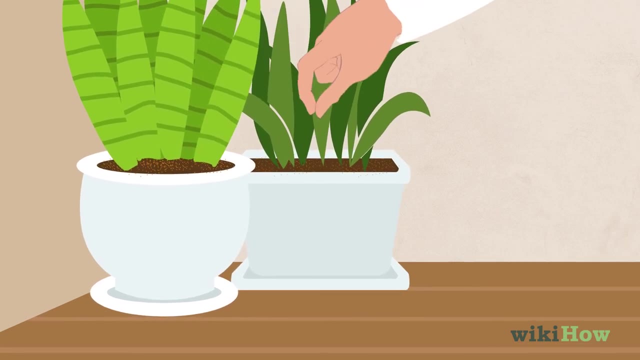 away. Cinnamon cloves, chili powder or coffee grounds sprinkled around the base of your plants will also deter ants. You can also place your plants on a ledge or in hanging pots so they're more difficult for ants to eat. You can also place your plants on a ledge or in hanging pots so they're more difficult for.